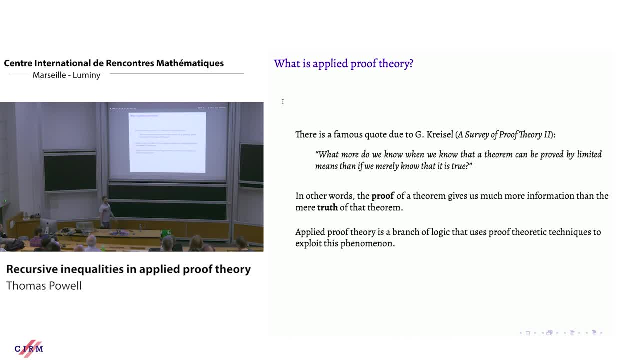 by Kreisel. You know I've had some talks where I didn't include this quote, but I've realized: no, I've got to stick with the tradition, and so the first slide always needs the Kreisel quote, and it's the motto of the area. What more do we know when we know that a theorem 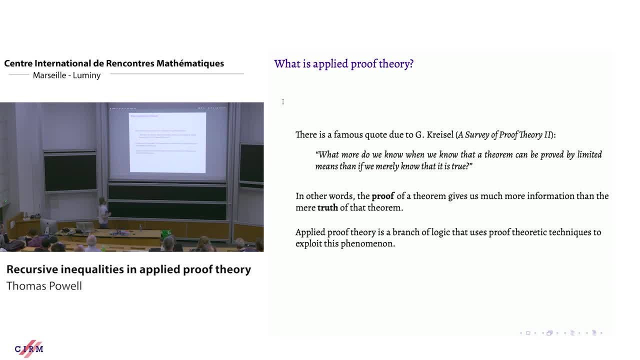 can be proved by limited means than if we merely know that it is true. all right. And so any mathematician will know that if you've proved a theorem, the proof of the theorem will give you more insight than the truth of the theorem. It somehow explains why that. 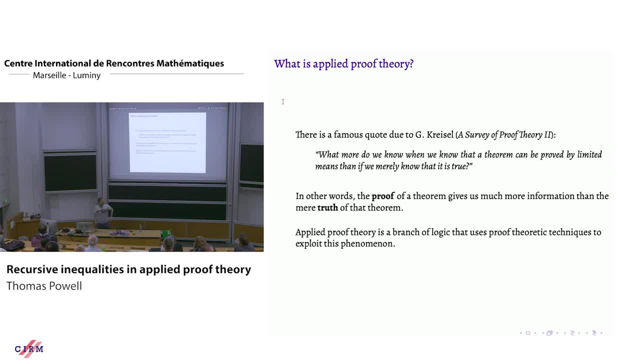 theorem is true. But what Kreisel is getting at is: can we use proof theoretic methods to actually produce something more? So can we give actual concrete mathematical new theorems that come from inspecting the proof, And can we use proof theoretic techniques to actually 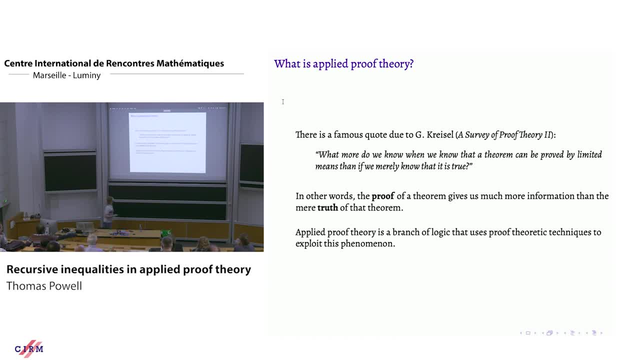 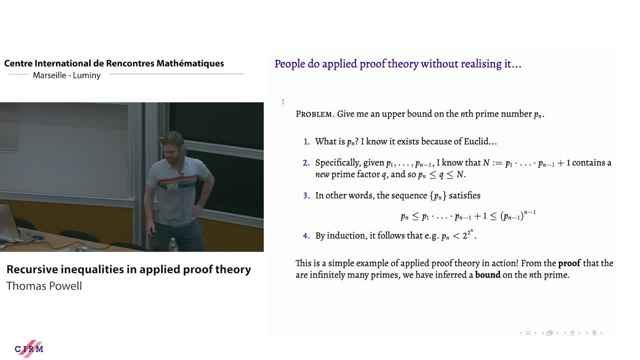 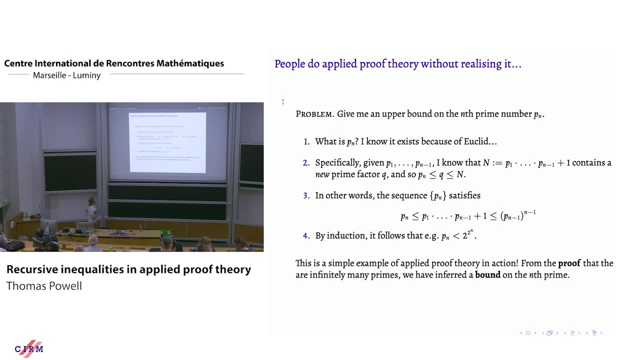 get stuff out of those proofs that a mathematician wouldn't see. So people do apply proof theory without even realizing it. all right. So here's Euclid's nice proof that there are infinitely many primes, And so if you're asked in a pub, give me an upper bound on. 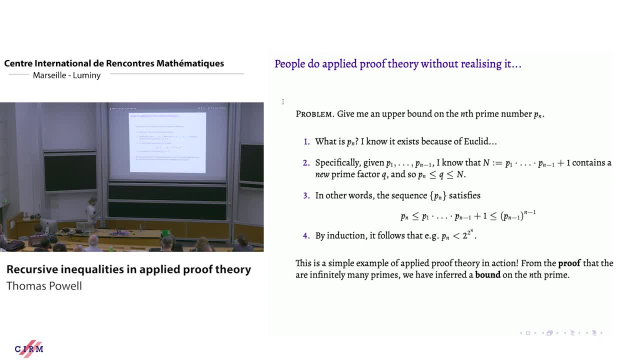 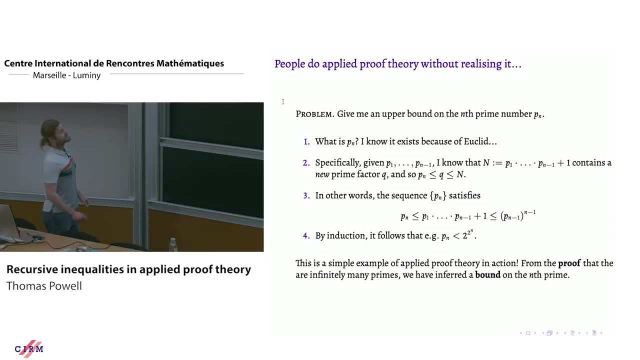 the nth prime number. what would you do? all right. So what is the nth prime number? You know it exists because of Euclid, And so if you're given the first n prime number, you're given n prime numbers. you can multiply them together, add one and that new number contains. 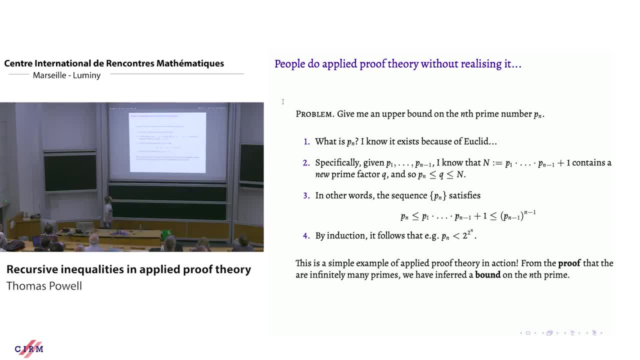 a new prime factor. okay, And so you know that the next prime number must be contained in this pn to pn minus one plus one, And so by iterating this you can come up with a very crude upper bound on the next prime number. So this is a simple example of applied proof. 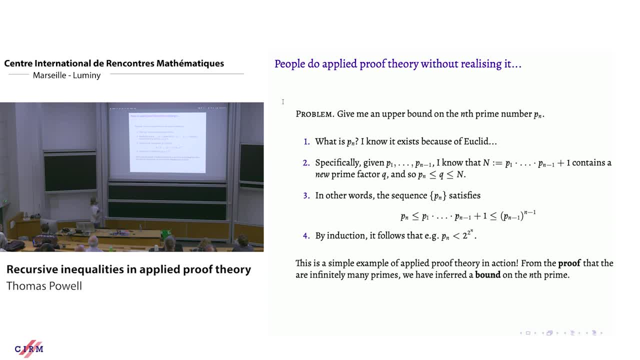 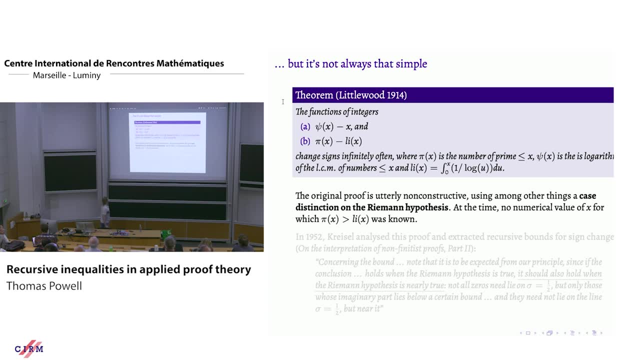 theory. From the proof that there are infinitely many prime numbers, we've inferred a bound on the nth prime number. It's not always that simple, okay. So the reason that we use these techniques from applied proof theory is that there are situations where you can have a really complicated 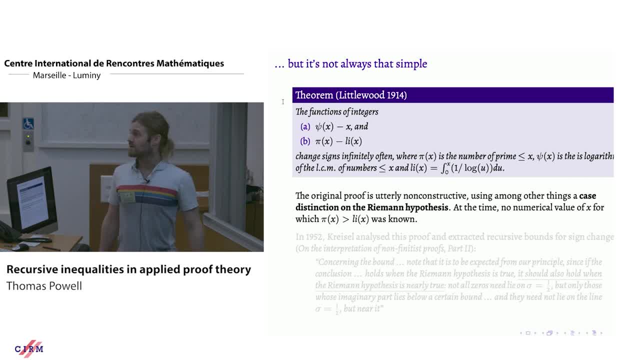 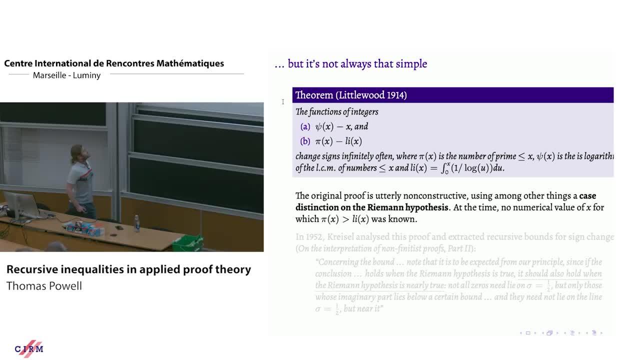 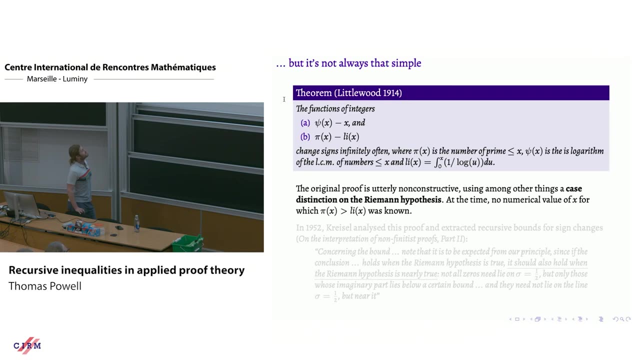 theorem with a really complicated proof and, using proof theoretic methods, actually gets information from it that a mathematician didn't see. So this is another theorem about prime numbers due to Littlewood, And this is a beautiful theorem of Littlewood that said that these functions change sign. 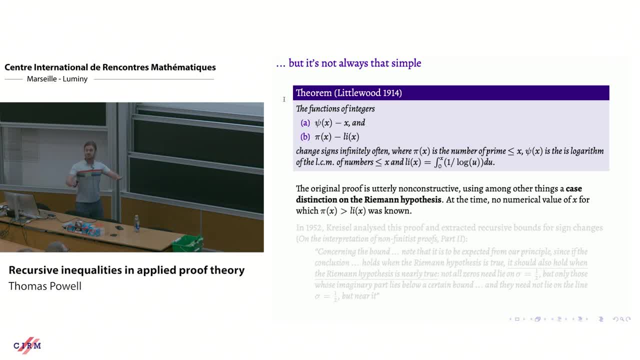 infinitely often. but when he proved it, the first point at which they change sign wasn't known. And the reason you know. it's an utterly non-constructive proof. It uses a case distinction on the Riemann hypothesis. So you can't just look at this proof and work out when kind 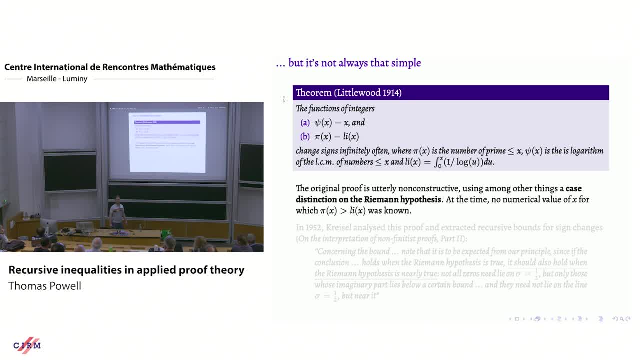 of numerical information from that, like you could with Euclid's proof that there are infinitely many primes, Okay. So Kreisel chose this as a case study for applying proof theoretic methods, and he used some complicated proof theoretic machinery to actually extract recursive bounds on the 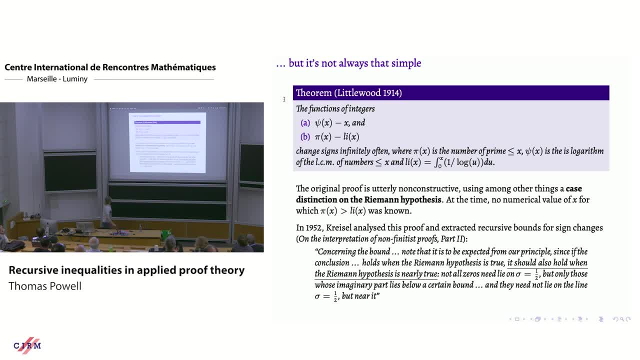 next sign changes And this is in one of his papers from the 50s And there's a nice quote from this paper and I'm going to come back to that. Concerning the bound, it is to be expected from our principles that if the conclusion holds when the Riemann hypothesis is true, 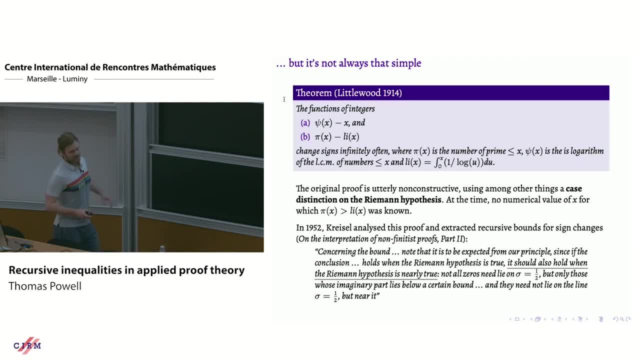 it should also hold when the Riemann hypothesis is false. So this is a very interesting thing. The Riemann hypothesis is nearly true And what's going on here is, if you've got a non-constructive proof, that's got a case distinction on something complicated, one way of getting around that. 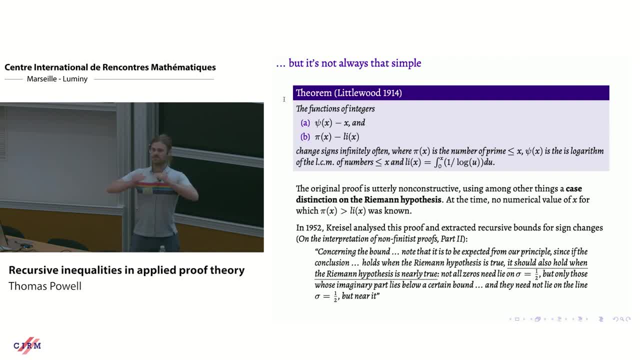 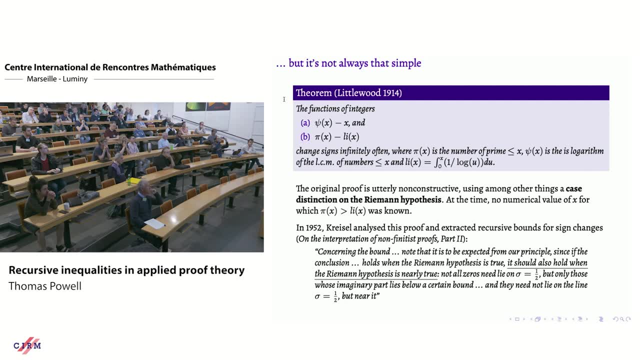 case distinction is to kind of convert it into an approximate case distinction. All right, And I'm going to give you an example later on where we can show quite concretely how that might happen. All right, So it's very clever tricks, If sort of an ordinary 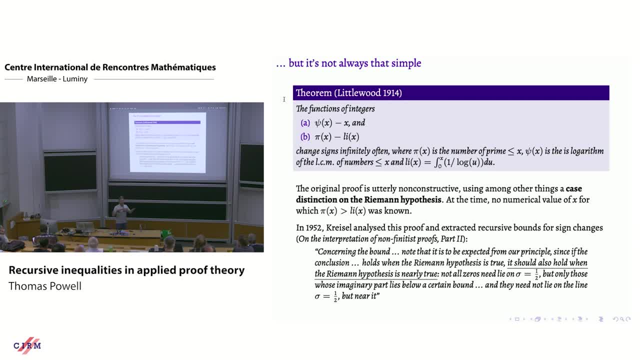 mathematician looks at this proof, they'll have no idea how you get any kind of computational information from the proof. But if you have techniques that allow you to deal with non-constructive things like horrible case distinctions on the Riemann hypothesis, often you get something. 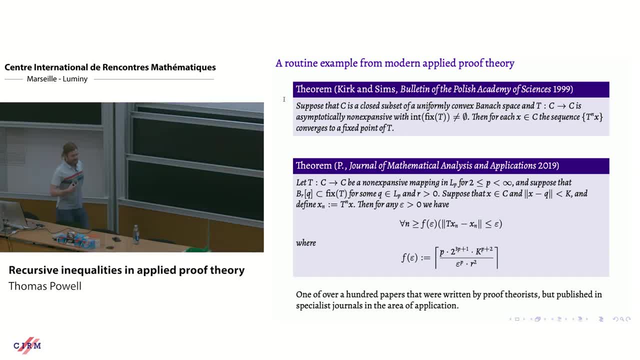 Okay, So applied proof theory is now a fairly standard area. Most of you have seen a talk in it, And so we produce papers routinely that allow us to get new concrete mathematical proofs—mathematical theorems from non-constructive proofs. So this is just one of mine. I picked 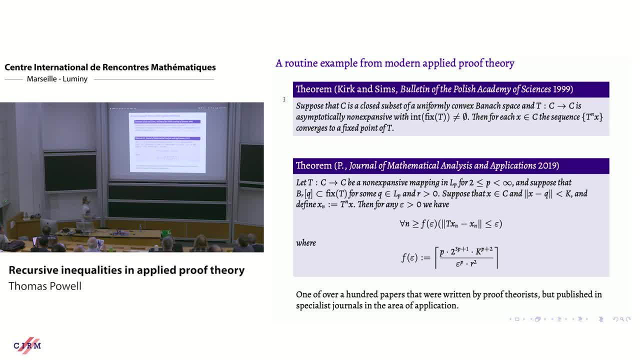 that just because I thought it was really useful. And I think it's really useful to I'm talking and I can say without offending anyone that it's not hugely interesting. So the idea here and you don't need to understand the details. okay, there's going to be lots. 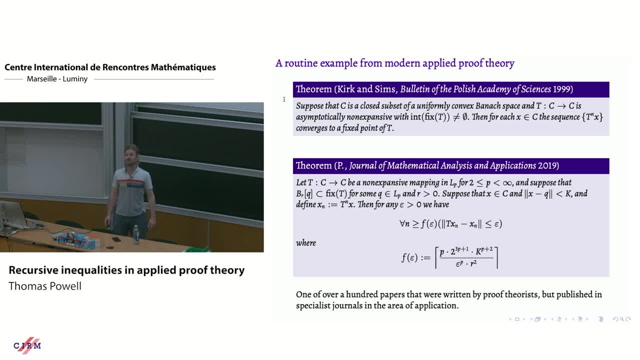 of slides in this talk where you don't need to understand the details. I'm just going to point to the relevant things. So there was a really nice paper that dealt with a particular kind of mapping and it showed that if the interior of the fixed point set was, 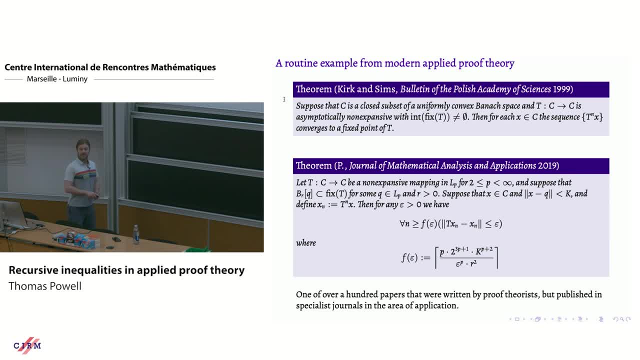 non-empty, then fixed point exists and the usual iteration scheme that you see in Banach fixed point theorem converges to that fixed point. The proof of this statement used all sorts of non-constructive reasoning, the existence of Suprema and so on, and there was lots of 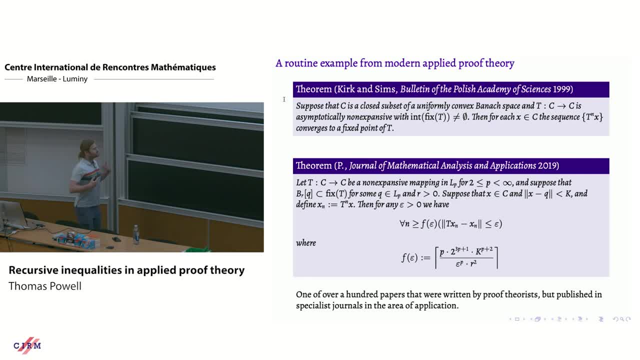 nice geometric reasoning in it as well And so applying proof theoretic methods in addition, so in conjunction with ordinary mathematical reasoning. one is able to get nice constructive information from this, And one corollary in the paper was a very, very concrete result that says well, if you're in an LP space and we have 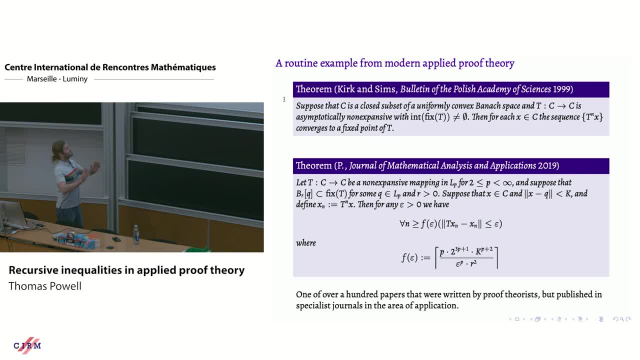 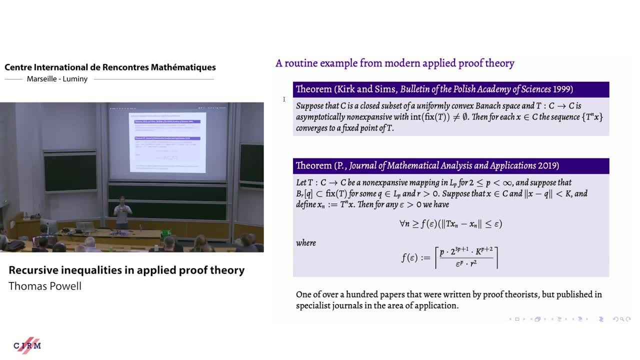 some data on how big this fixed point set is. then there's a concrete rate of convergence in terms of sort of how close the iterates get to being a fixed point, And so for people in areas like you know- a functional analysis, optimization- it's actually really useful. 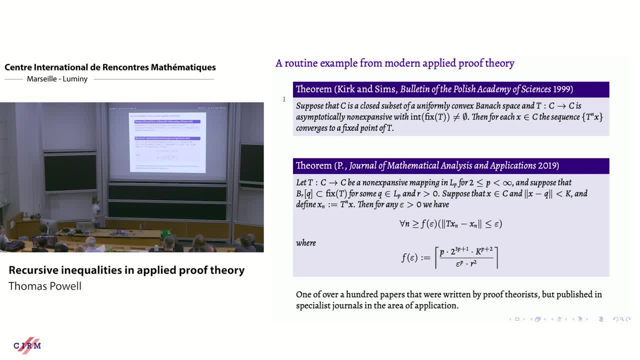 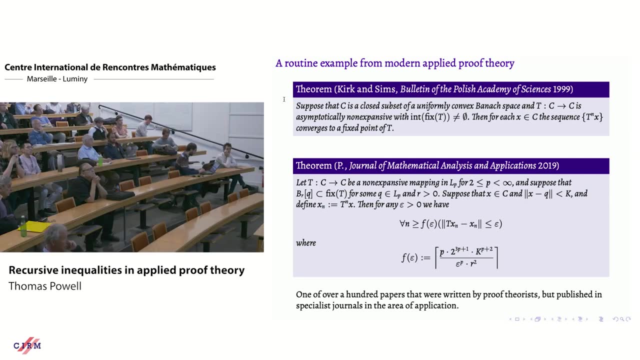 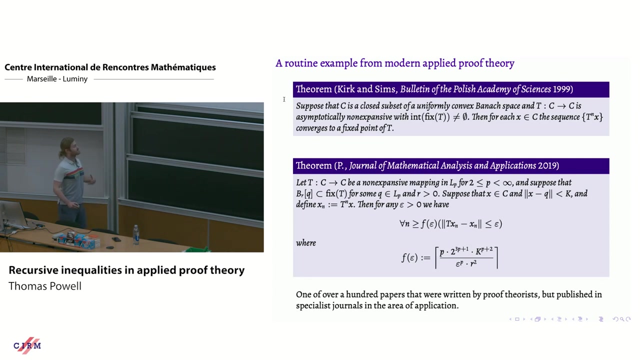 to have concrete computational information on how good your algorithm is. And so, for example, if you're in an LP space and you have some data on how good your algorithm is And you know, a phenomenon here is that the rate of convergence. it's not something super complicated. It doesn't involve things like Ackermann functions or primitive recursive functionals or anything like that. It's just a simple polynomial, All right. So it's something that you would normally expect to get in a maths paper. when they show that you've got an algorithm that converges, You hope that the rate of convergence is just going to be some sort of polynomial, nothing horrific, And that's indeed almost always the case with results in this area- that what you get at the end is just some sort of simple polynomial band. 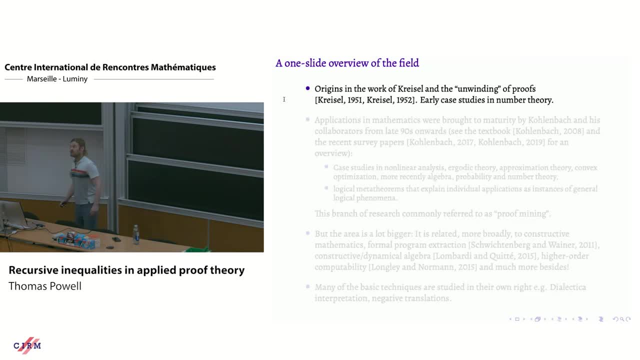 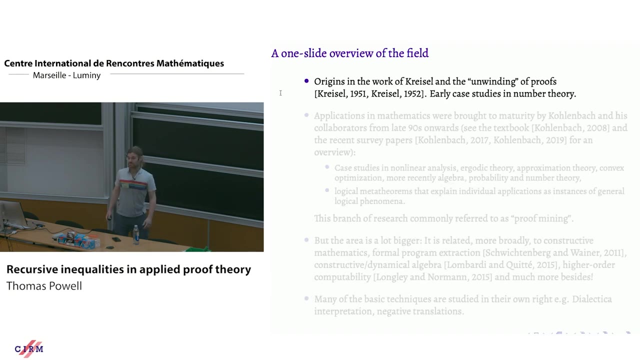 Okay, so I'm just going to give a one slide overview of the field, just detailing its history and the people who are working in it. So, as I said, the origins are in the work of Kreisel, who I mean. actually, the origins are in Hilbert's program. So the idea of 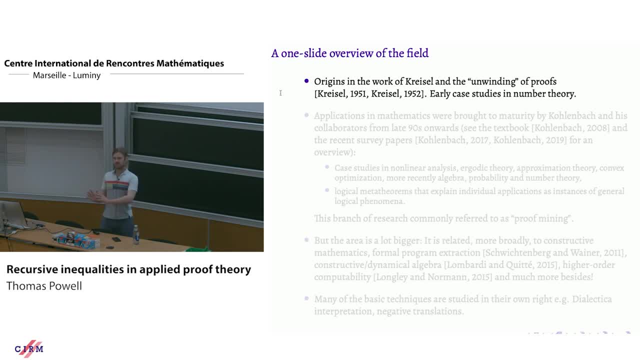 finitizing mathematics, reducing it to a proper finitary system. And there were lots of tools that were developed then to try to do this, And so Gödel actually developed a technique that took proofs in piano arithmetic and reduced them to basically programs in system T- He didn't call it system T, but basically higher order programs, And these are relative consistency proofs. So people are much more inclined to believe that a higher order functional language is consistent than they are inclined to believe that piano arithmetic is consistent. 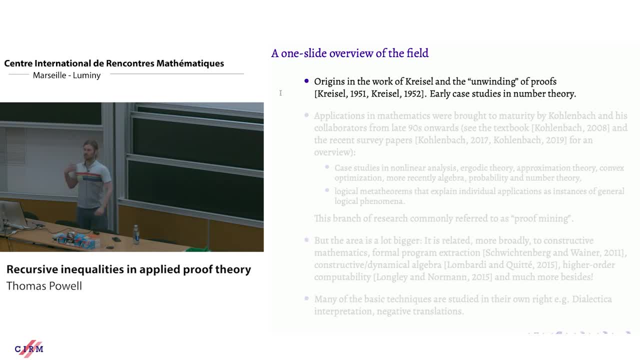 And so reducing it to a simpler language. you kind of you're more inclined to believe the consistency, And what Kreisel observed is that kind of. while these techniques used to prove relative consistency were somehow used in a negative way. So if we don't have a proof of contradiction in this system, then we also don't have a proof of contradiction in this system. you can use them in a positive way. 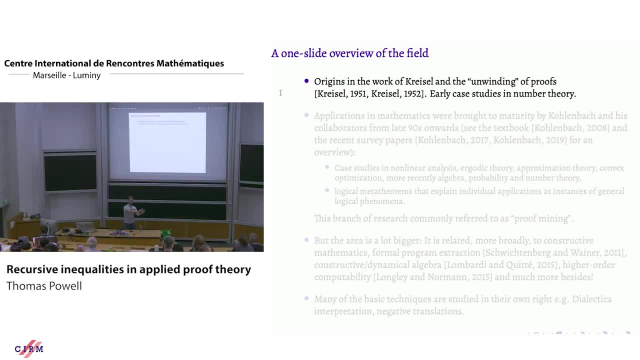 Namely, if we have an existence proof in the complicated system, we can turn that into a program in the computational system, And so the very same tools that had their origins in Hilbert's program can be turned on their head and used to extract programs from proofs, And that's typically how they're used today. 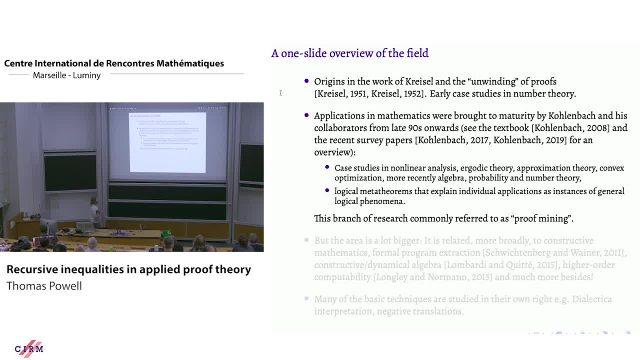 So applications in mathematics. there are a couple of really crazy case studies in the 50s, very dramatic ones kind of, you know, Riemann hypothesis theorems about prime numbers. But this area really found its ground when it was shown that you can consistently use proof theoretic techniques to produce new theorems in mathematics and publish those theorems in mathematics journals. So this was primarily due to Ulrich Kohlenbach and his collaborators around about the late 90s They found the first really good seam of applications in applications: Approximation theory. Since then it's been applied in all sorts of different areas by different people. 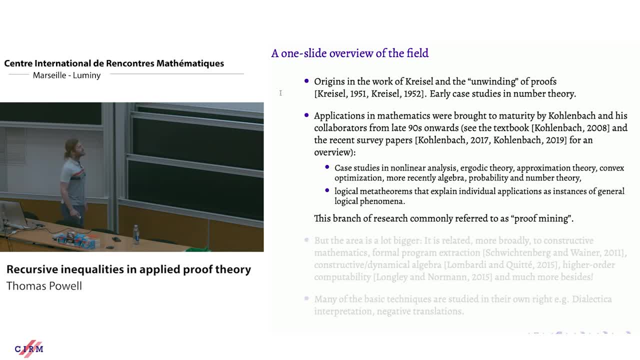 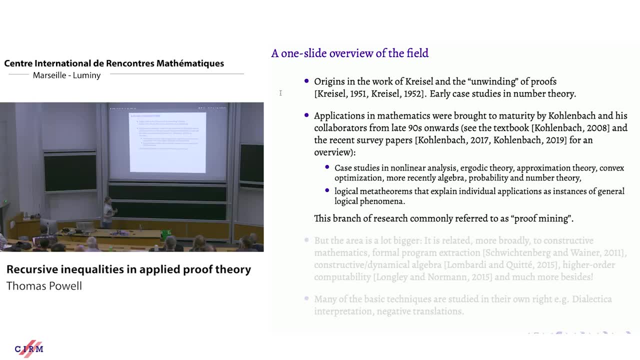 So ergodic theory, convex optimization and more recently we're starting to see applications in algebra, probability and back in number theory. So as there are more and more case studies in parallel, one starts to see logical papers that describe what happened in the case studies in a general way. 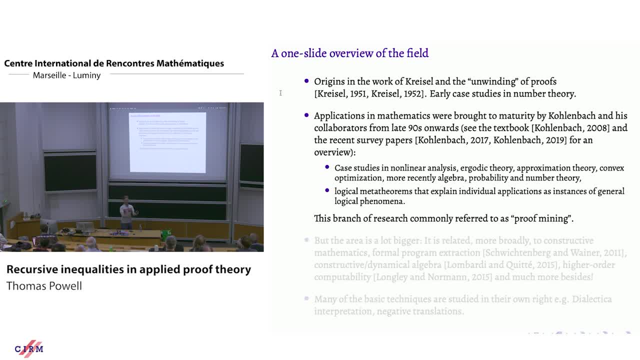 So if you found that, for a certain kind of proof, in a certain area of analysis, You kept being able to get good information, The answer is: well, why was this? Why did we get nice polynomial bounds? Why was it that all of these horrible, non-constructive principles in the proofs didn't impact our ability to get quantitative information? 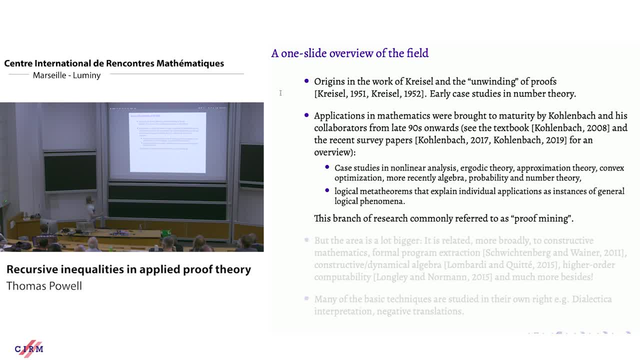 And so typically these are then explained using logical metatherms that say: well, if you always have a proof of this form in this kind of logical system, if you have a proof in that logical system, then you get a reasonable program. 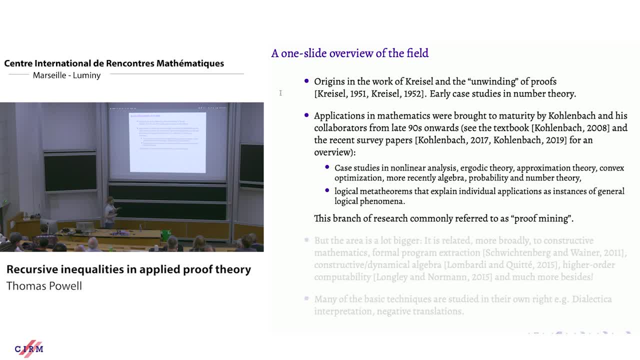 And so these two things kind of go Hand in hand. On the one hand, you've got pioneering case studies that try to bring proof theoretic techniques into new areas of mathematics, And then, once you've got a critical mass of those logicians start thinking: well, why was that possible? 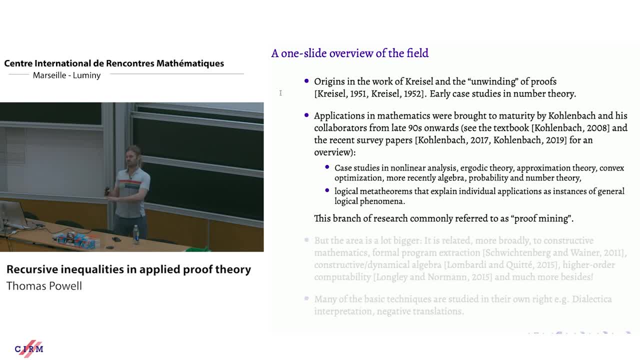 Can we explain that in general terms. So can we explain mathematical phenomena in terms of logic. So both of these are really interesting And the interaction between those two things is really interesting as well. So this branch of applied proof theory is commonly referred to proof mining. 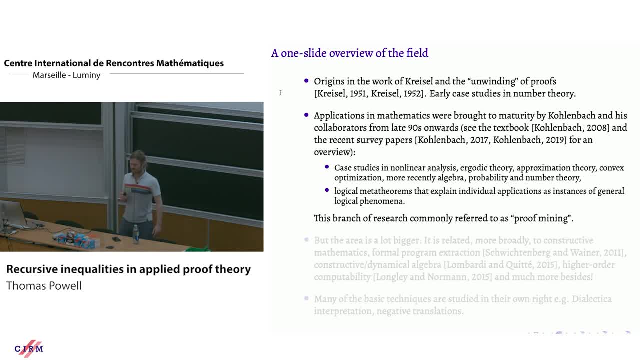 I really hate that term because it's it kind of It gives the impression that you're just hammering away. right, You've got your proof, you've got a technique, you crank the sausage machine and something comes out. But it's really not as simple as that. 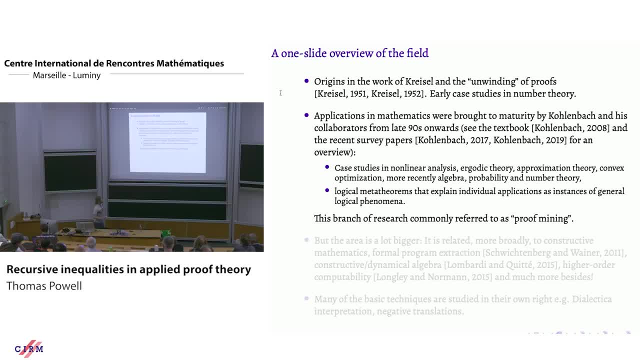 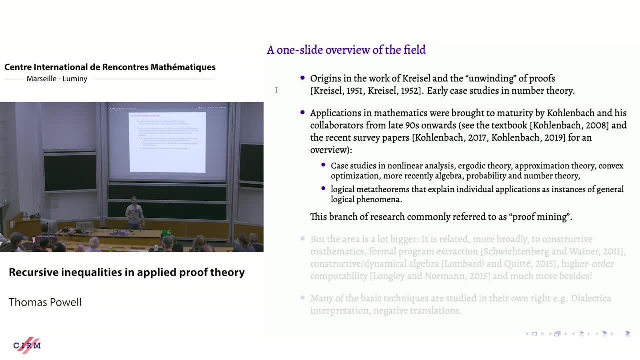 So I wish they would, they would stop using this terminology. But it's, it's, it's, it's stuck, And actually my grandfather was a coal miner, so it skipped a generation, But the family is back in the business. But just to be more inclusive, I mean, if one defines applied proof theory as just being the people who are doing it- 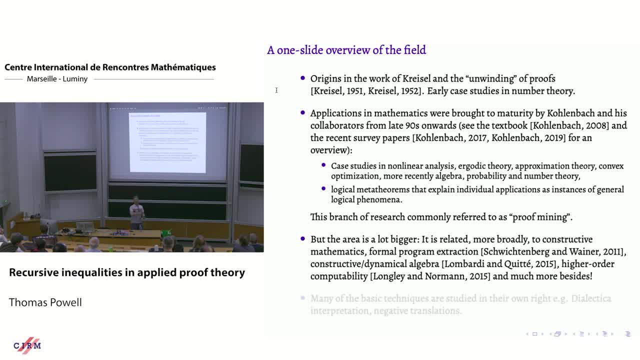 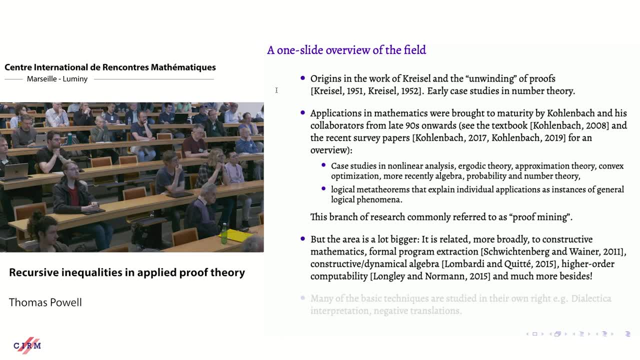 People who use proof theory to and proof interpretations to get computational contents from proof or to to understand proofs on a computational level. Of course this is a much bigger area And there are many people in the audience here who do that. So kind of constructive mathematics, formal program extraction, for example, being implemented in theorem provers. 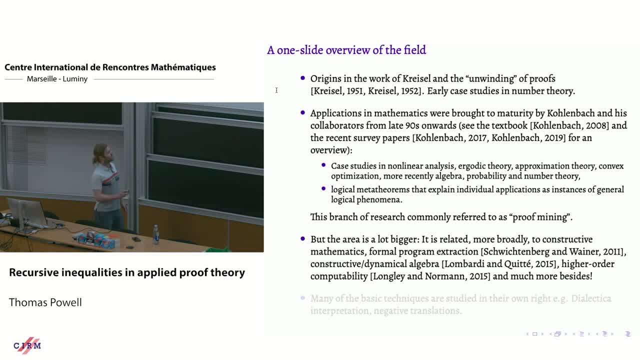 That's a really important area And there's a nice alternative perspective to proof theoretic techniques in the book by Schrichtenberg and Rayner, Constructive dynamical algebra. I mean, these don't always use Explicit proof theoretic techniques but I think you know, often in this area people look at the non constructive proofs and try to kind of massage them to get some sort of computational equivalent out, and that's very much applied proof theory, even if you're not applying techniques explicitly, I would say. and of course there's all sorts of areas that are connected to it, like higher order computability. 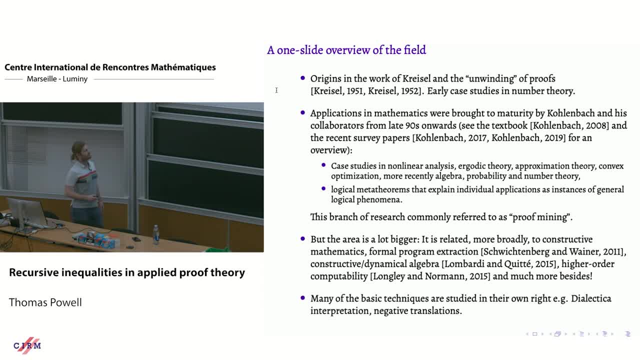 And I should also mention that lots of techniques that are used in proof mining and applied proof theory in general, like the dialectical interpretation, negative translations are studied in their own right and used for other things. So we saw negative translations Yesterday and dialectical interpretation that's been applied from a categorical perspective. it's been extended to say things about programming, languages and type theory. 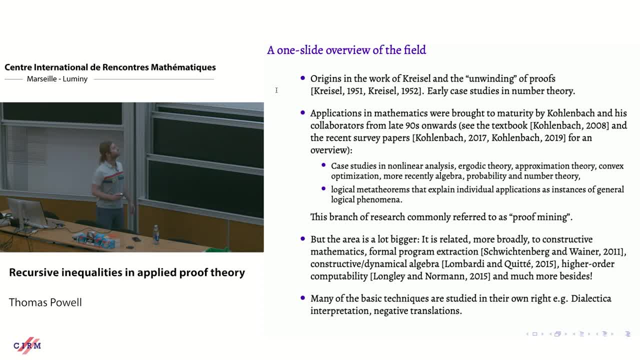 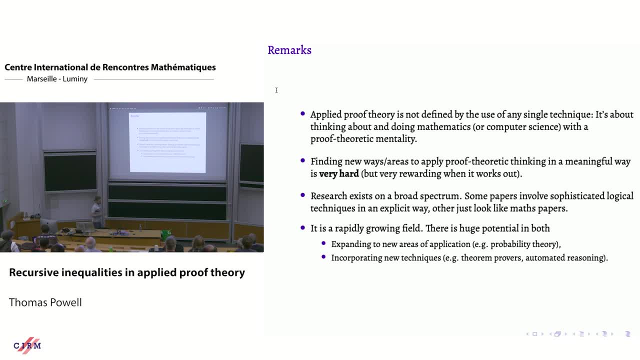 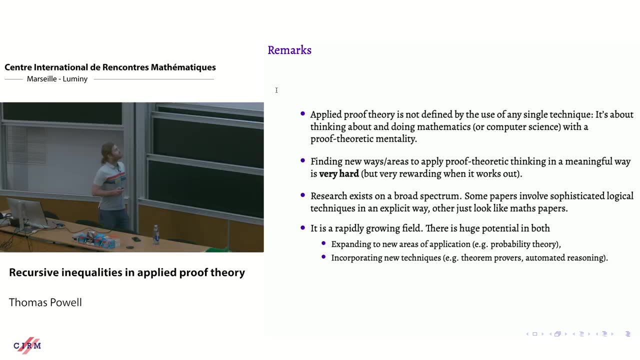 So there's a very rich world surrounding applied proof theory, Mr slides. Yes, So just some remarks before I go into the talk and present the explicit results I wanted to talk about. Proof theory is not defined by the use of any single technique. 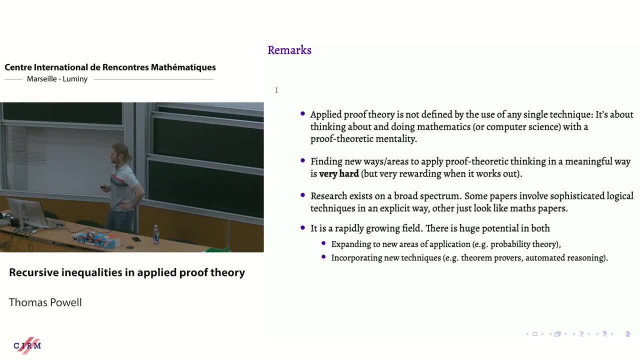 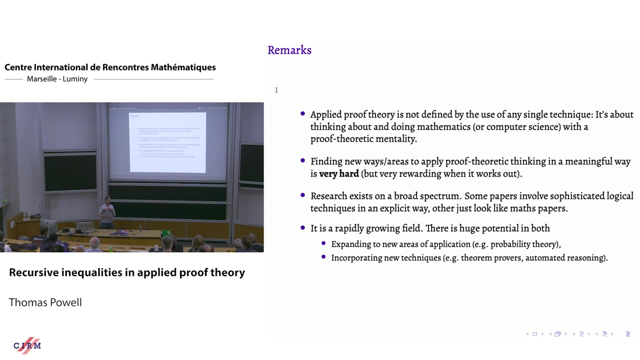 So it's not just about people who use dialectical or use realize ability or anything like that. I think one should really define this area it's it's it's thinking about and doing mathematics or computer science with a proof theoretic mentality. Finding new ways to apply proof theoretic thinking is really hard, and that's something that you don't necessarily see when you read a paper. right, so kind of, if there's a paper that presents some new theorem in a particular area of optimization. 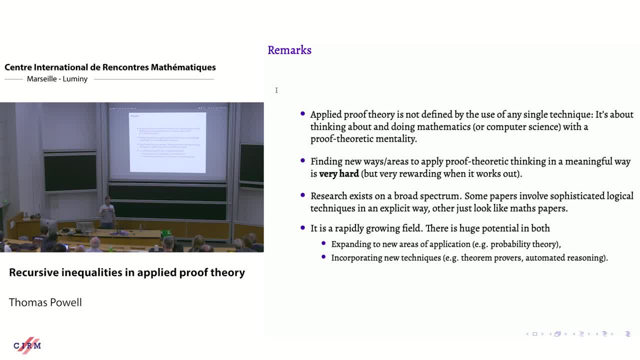 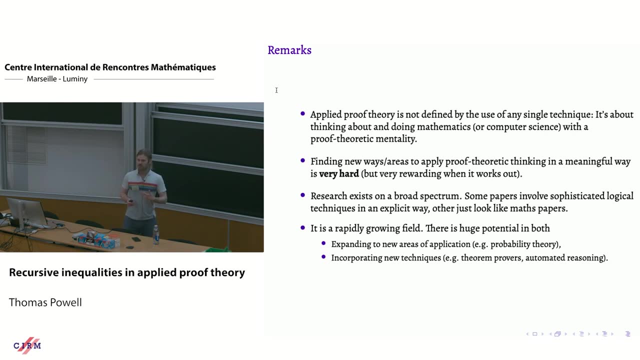 You don't necessarily see what's being done. but what one doesn't see is the sheer number of papers that were read and understood to get to the point where one could find An area where these proof, theoretic techniques do something. And so I've, you know, I probably read hundreds of- not not in detail, but go through hundreds and hundreds of papers to try to understand an area, to try to get a sense of kind of 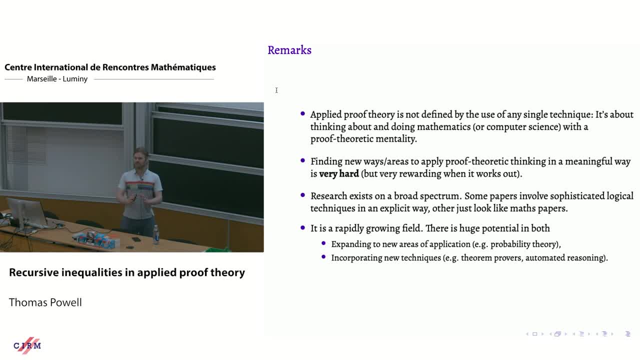 Where are the bits? were looking at a proof as a proof, theorist would help and if they do, Is it of relevance in that area? Is this an area where people care about bounds? all right to the proofs, to the theorems. have the right form that what we could expect to extract would be relevant for the people in that area. 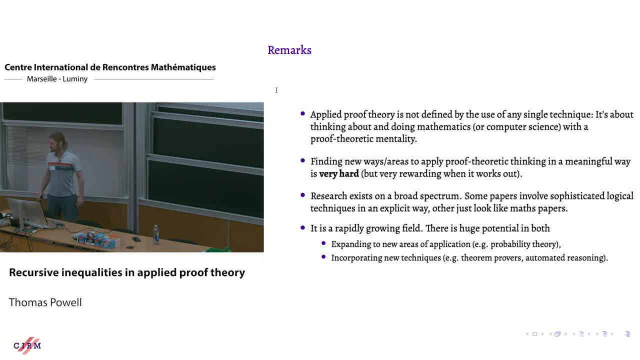 So it's hard but really rewarding when it works out and the research exists on the broad spectrum. so you've got some papers in this area that just look that they're probably logical right. so they introduce a type theory and they present metamathematical results. 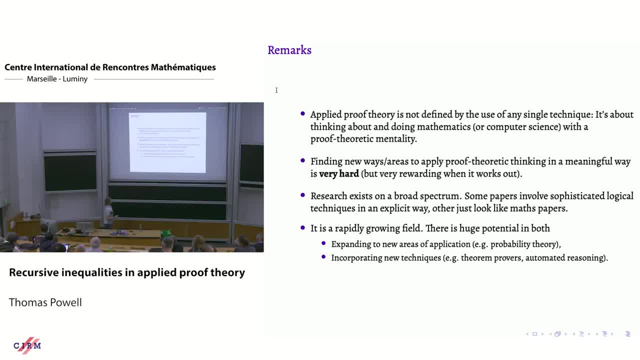 Other papers just look like maths papers and i've given talk, represented stuff that just looks like Maths research and people have asked: well, where is the proof theory? and that's a really good question. it's somehow there, but Really done informally and so when applies formal methods, but not in any kind of rigorous way, you do that in conjunction with 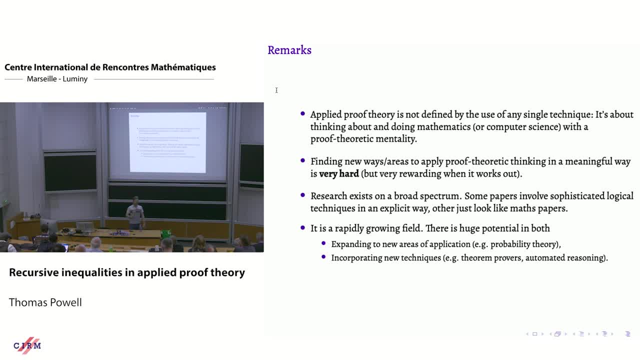 Ordinary mathematical reasoning and i'm writing a paper at the moment where i'm trying to give a worked example of how this kind of how this informal use of proof theoretic method goes. and i'm finding it really hard because I know i'm doing proof theory but i'm not quite sure how and 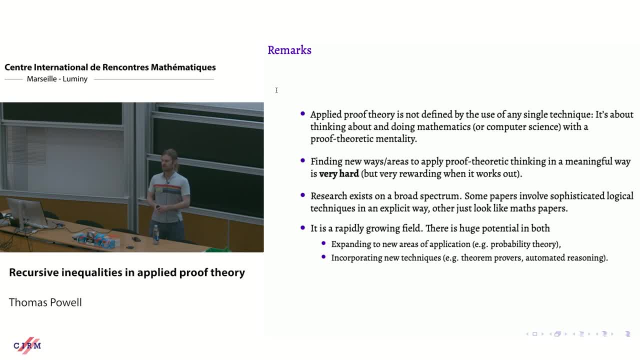 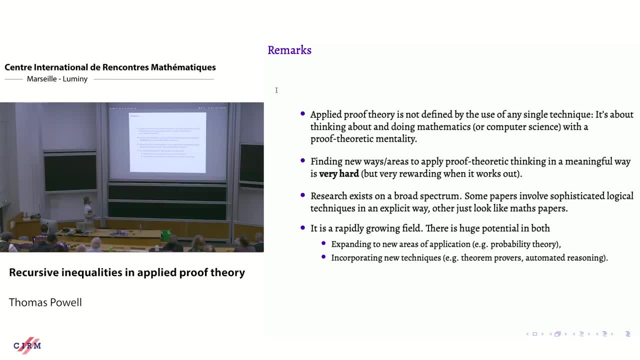 i'm trying to. I'm trying to sort of design informal proof cheese that explain what's going on. but it's really tricky. But this is really rapidly growing field, so there's a huge potential both in expanding to new areas of application and also incorporating new techniques, and those are things I want to talk about at the end. 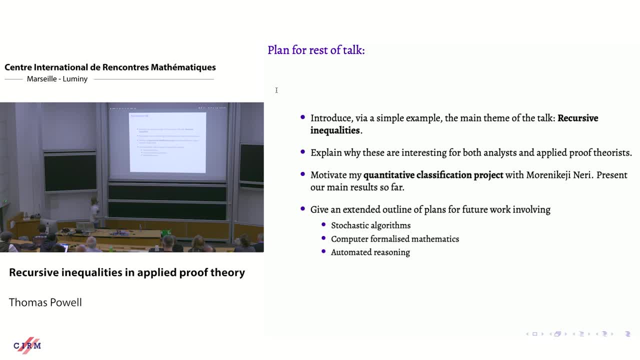 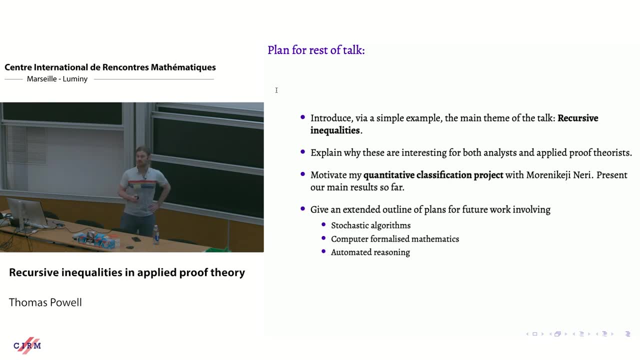 So there's my short introduction. so The plan for the main part of the talk is to Present the main topic, Which are recursive inequalities, Explain what they are and also why they're interesting for both analysts and applied proof theorists. and then I want to motivate a classification project i've been working on with my PhD students. so what? i'm going to present his joint work with keji neri. 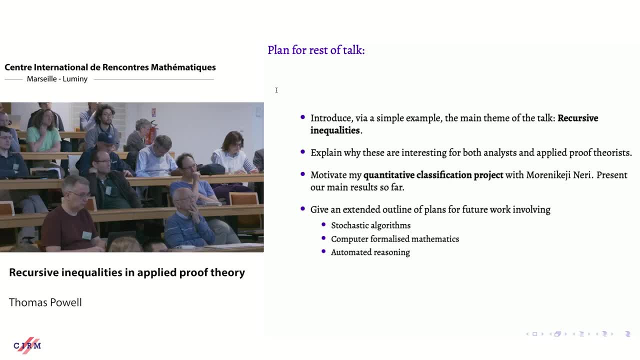 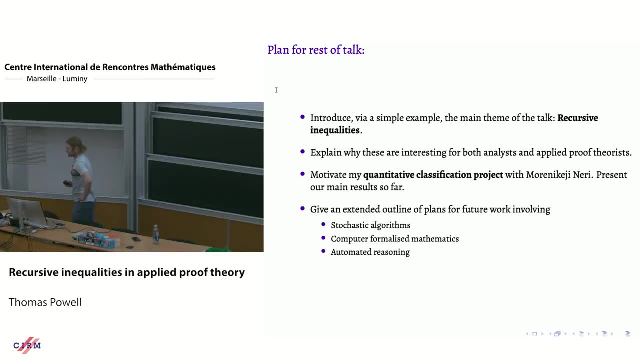 And i'm going to present our main results and also explain where we want to go in the future, and that's probably the most important bit of the talk, which will be presenting things that we haven't done yet but we hope to do. Okay, so recursive inequalities. 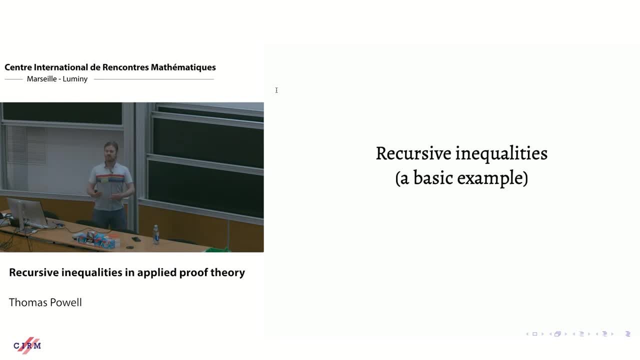 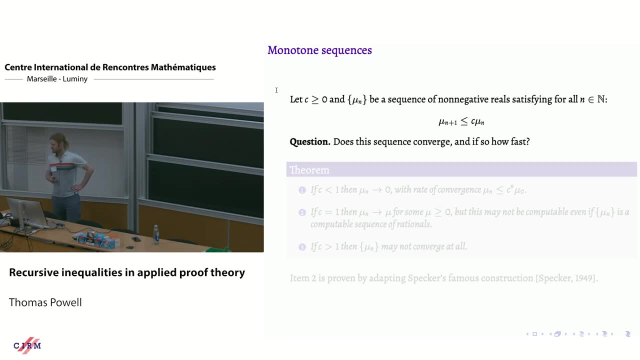 And i'm going to motivate both recursive inequalities and the proof theoretic ideas that are associated with them by a really simple example, And it's the following: So forget everything that's gone in the talk so far. that was just a general overview of the field and i'm going to try to make it self contained from now on. 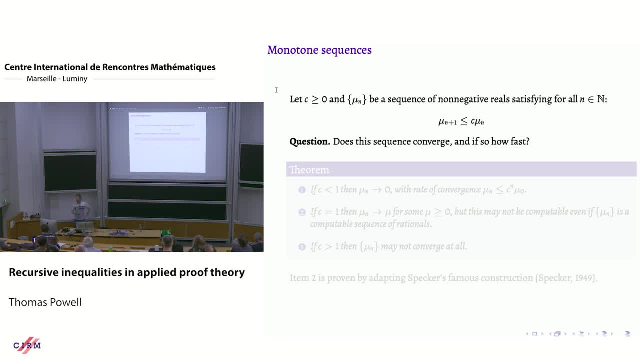 So let's just pick some positive real number and a sequence of also positive real numbers that satisfies this recursive inequality here, right? So it's kind of monotonicity With a constant, And so very natural question is: does the sequence converge? and if it does converge, how fast does it converge? and there are three answers to this question, depending on the value of c. 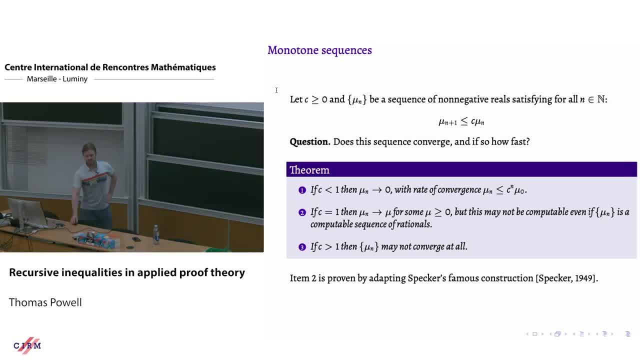 So if c is less than one, then we essentially just have a contraction right to each element in the sequence. the next element is going to be less than c of the previous one, and so if we iterate that, that's eventually going to converge to zero. okay, so it converges. 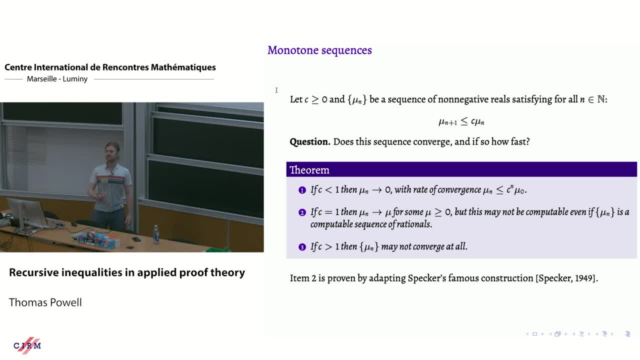 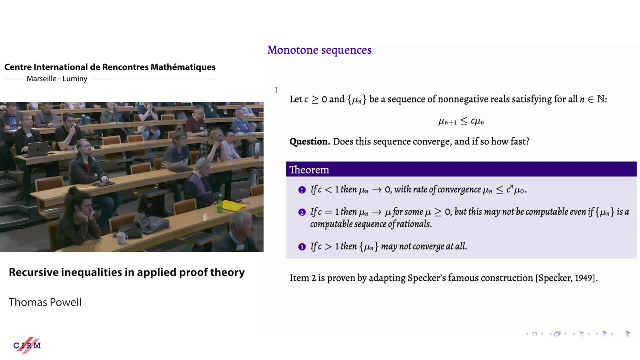 And also you get a completely obvious rate of convergence is just c to the n. All right, so that's all very straightforward. If c is greater than one, the sequence might not converge at all, because if we allow that then we can get oscillating sequences. so that's fairly uninteresting. 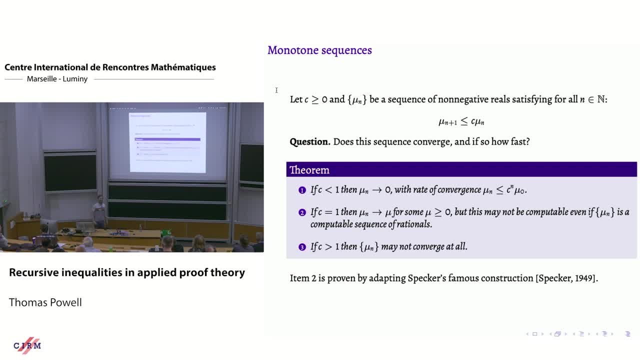 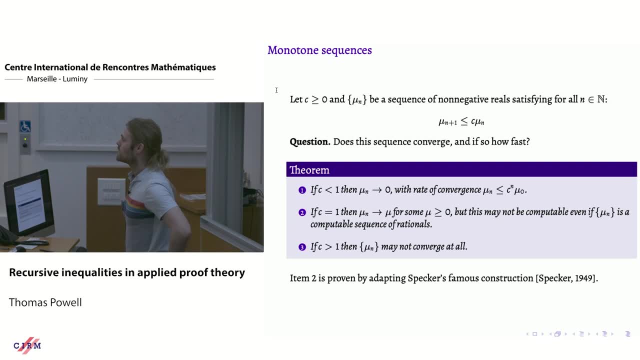 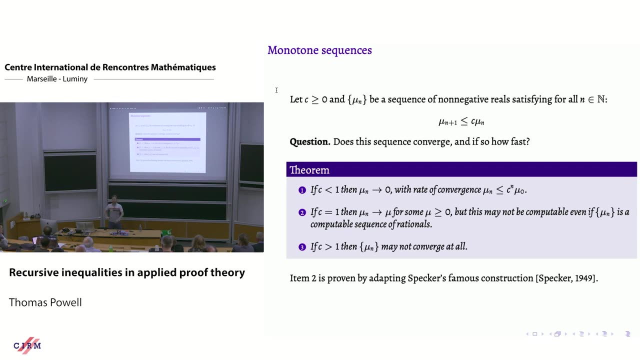 If c is equal to one, we're in the situation that we have a monotonically decreasing sequence. we know it's bounded below and so it must converge to something. but yeah, You said oscillating, but i will report it as divergence. Yes, It could do as well. i mean, it could oscillate, it could, it could diverge, it could do anything, but it may, it may not converge. that's the point. 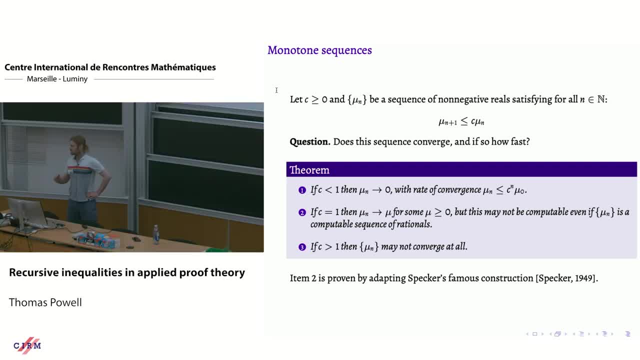 But if c is equal to one, We know it will converge, but there's a well-known fact from computable analysis that what it converges to may not be computable. in other words, it converges but it may not have a computable rate. and this is a really interesting construction that involves somehow defining a sequence in terms of the halting problem. 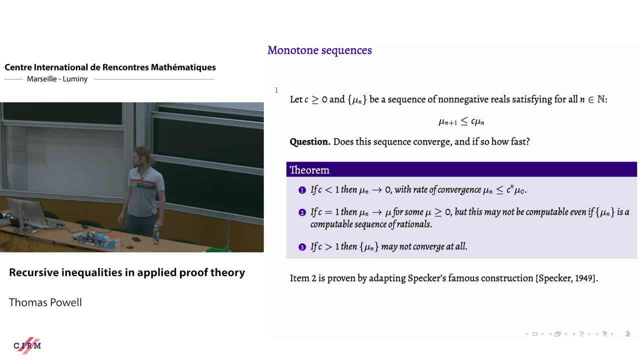 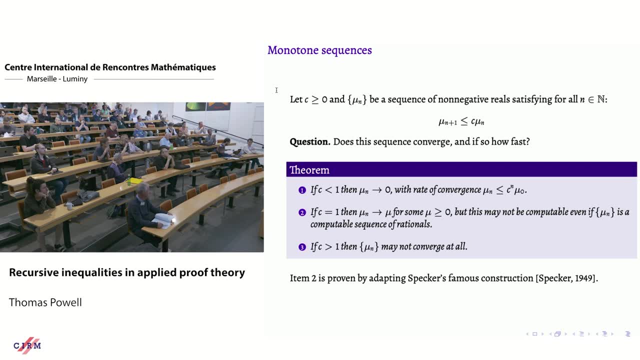 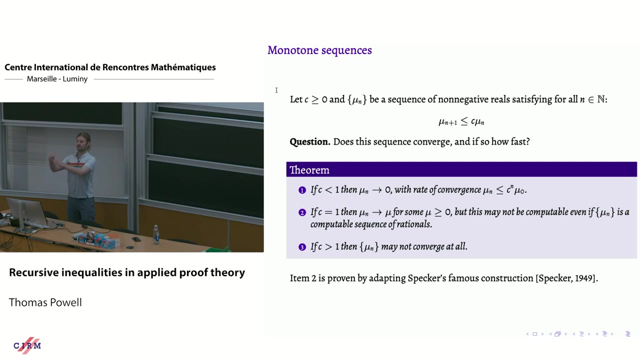 It's quite weird. And when you present people with this fact and they haven't heard it before, they, they somehow don't believe it. yeah, In what sense? using the sequence and see it, or He, What is that case? the question? so A computable real number. so one way you can, you can always find a, an excellent approximation of that number in. 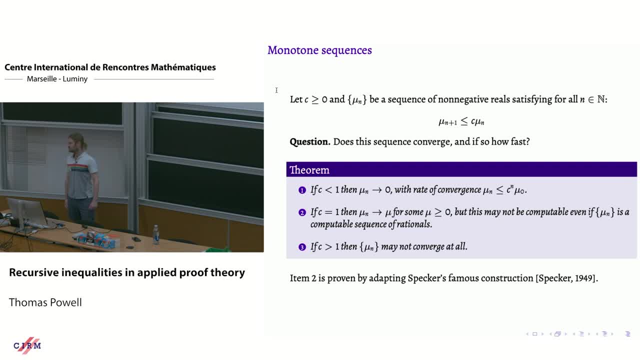 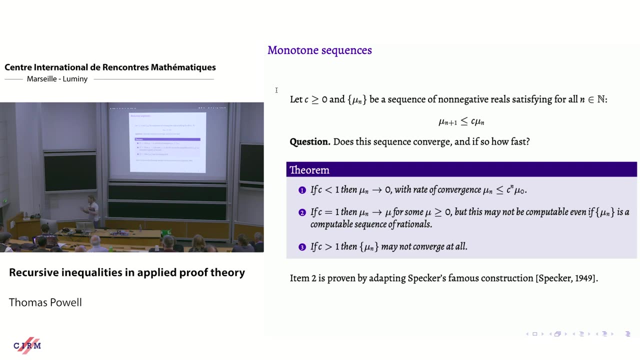 Yeah, I mean you end, doesn't that? The limit is just not, it's not to do with me, when necessarily, i mean it's No, no, okay, it's not an algorithm. what i mean is is that you can have a monotonically decreasing sequence and the limit of that? just take the limit. that thing is not a computable real number. 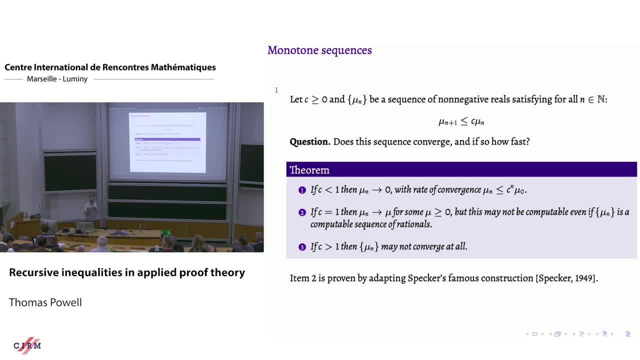 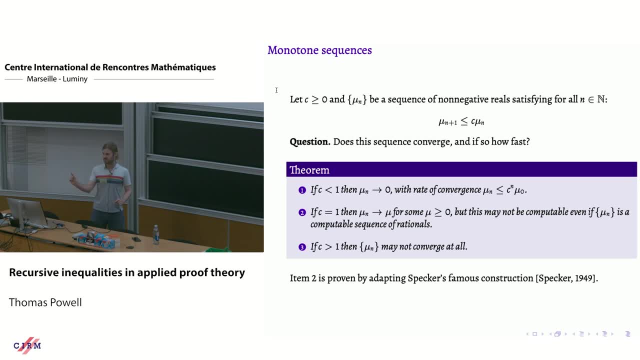 The moon can be computable. so that's the point, that so the mu? n can be a computable sequence and The individual elements are rational numbers. so you know everything about the sequence. you can compute any point in the sequence to any level of, of, of, of detail, but the limit is not a computable number. 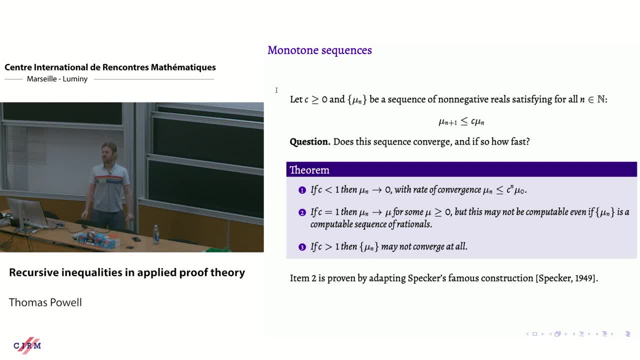 Okay, so you fix mu n and c in advance. they happen to all be Exactly, exactly so it's it's, it's, it's an established construction. is that the speck, a sequence you can? Is it all the same if mu n is actually? 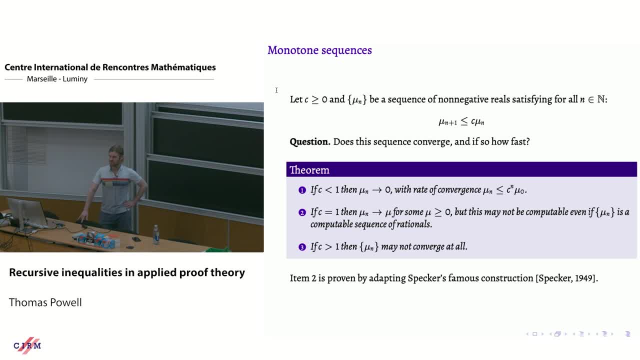 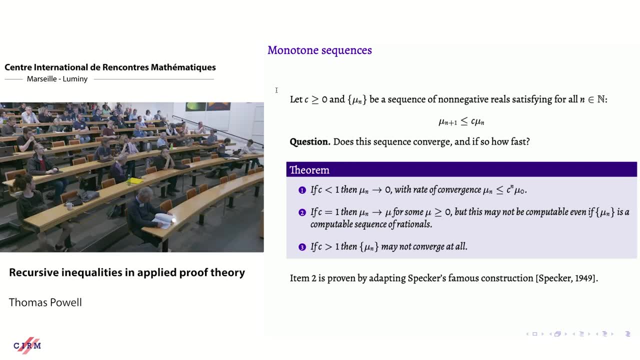 So you're not fixing mu n in advance, but mu n is somehow data, So it's like a function symbol or something You can call it a function symbol. So it's like a function symbol or something You can call it to see certain values of it, and you just know this semantic property. 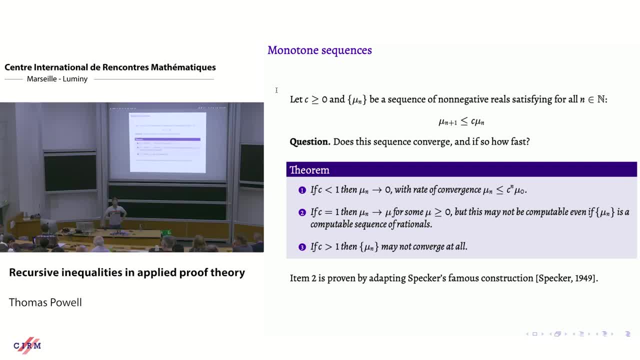 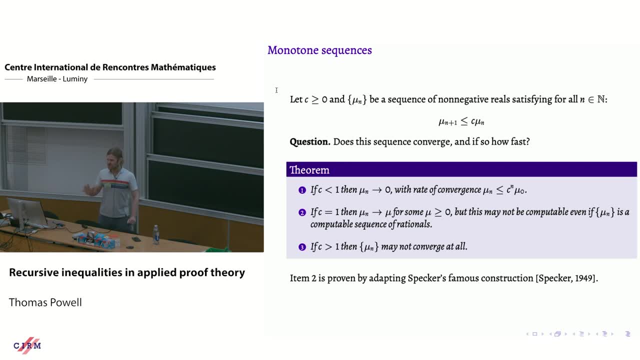 Sorry, I don't understand the comment. Is it that this, this is nothing like? this is just a fact. I'll explain it up like it's. it's it's sort of tangential, it's. it's weird, it's really weird. You kind of, you kind of construct. 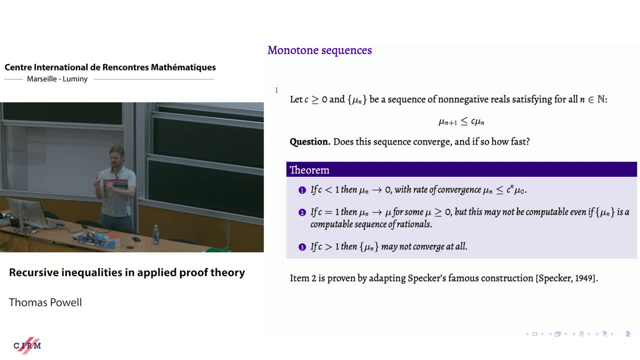 An infinite series where the individual elements of the series Are defined in terms of whether the K th Turing machine halts on input k And Within a certain number of steps, And so you can always decide that. but if you had a computable rate of convergence, you could solve the halting problem. 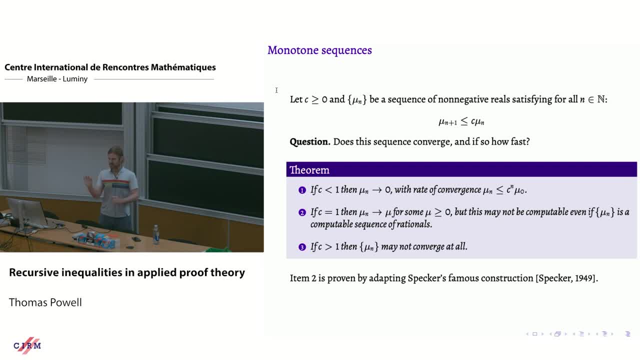 Is to do with that. so it's a. it's an explicit construction of the mu n Where the result would be: if you had a rate of convergence, you could solve the halting problem. it's so it could be that you do have a rate of convergence in this case, but there are examples where you don't have a computable rate of convergence. 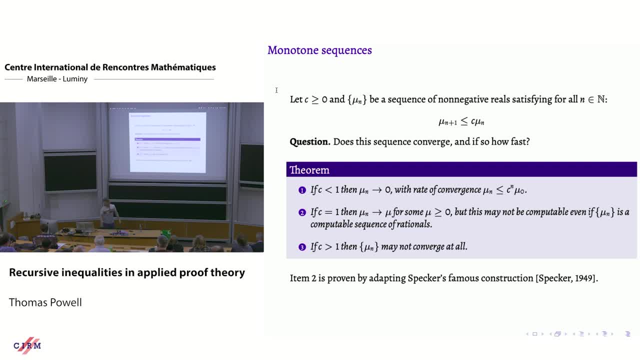 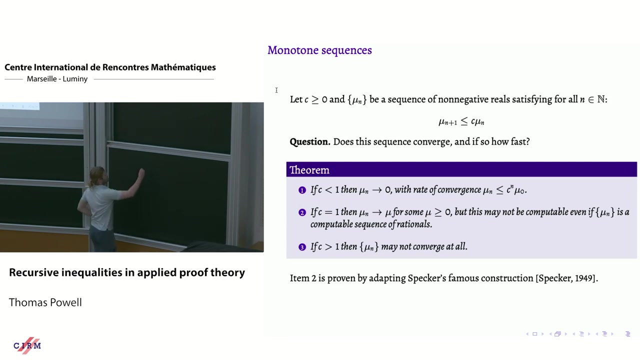 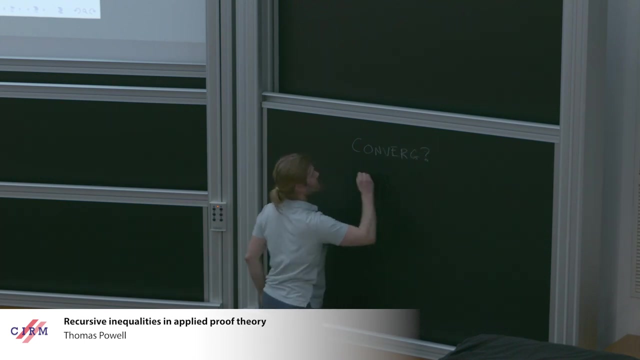 All right. So anyway, the point is that we can. I'll just write one thing on the board: Some chalk, So you somehow this have this problem. first question is: does it converge? So sort of yes or no whoops, And if it's no, it's sort of an interesting. and if it does converge, is it with a computable rate? 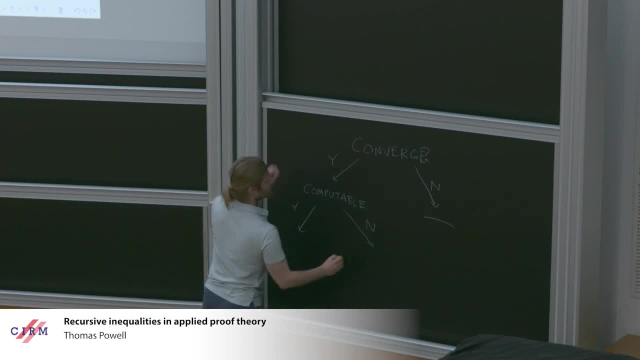 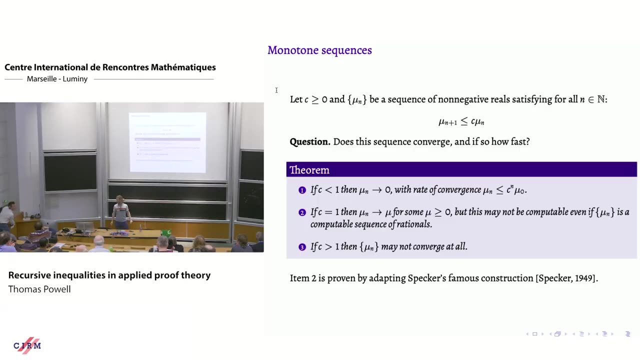 And then the answer to that could be yes, Or it could be no. And even in a super simple, Let's say I'm, I'm only going to, that's all I'm going to write on the board so I can, Just to keep it there. 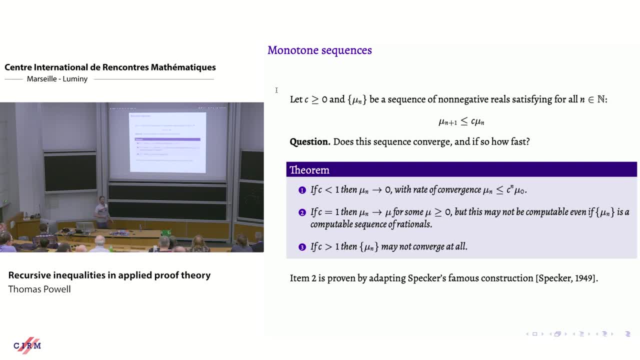 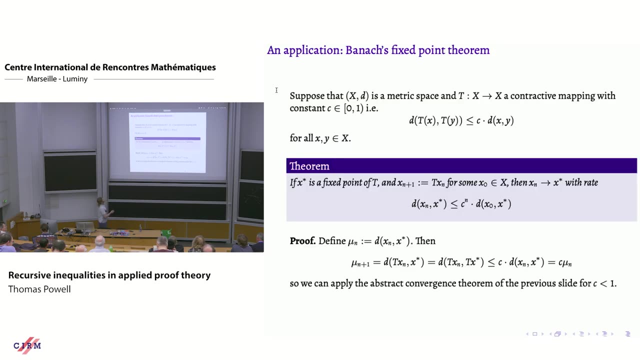 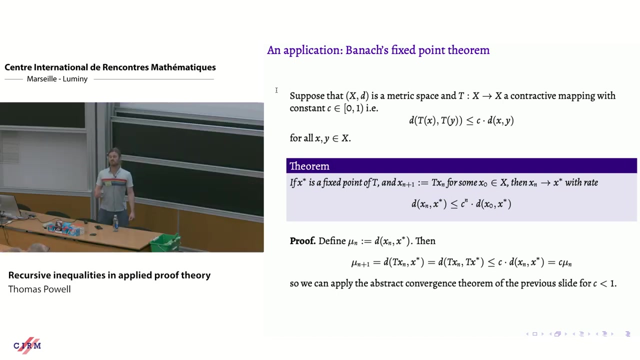 Even with a super simple case like that, answering this question is not entirely obvious and it depends on the parameter of the recursive inequality. So why these recursive inequalities useful? so this is just completely elementary analysis. well, in this case this is connected to the benefits point theorem. so the benefits point point theorem says: if we're in a metric space, we have a contractive mapping, then a fixed point of that mapping exists. 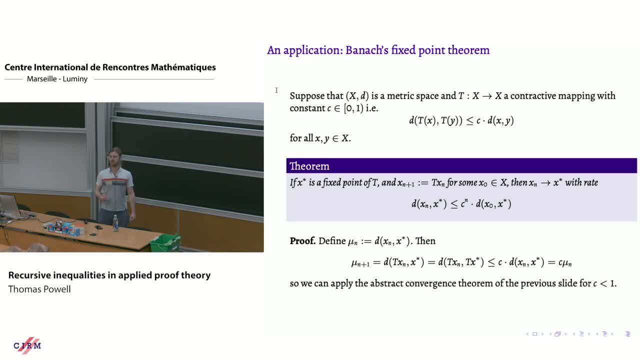 And, moreover, the usual iteration scheme converges to that fixed point. and so if we put aside for a second the existence of the fixed point, When it turns to in terms of converging to that fixed point, we can essentially reduce that situation to the previous, to the recursive inequality on the previous slide. 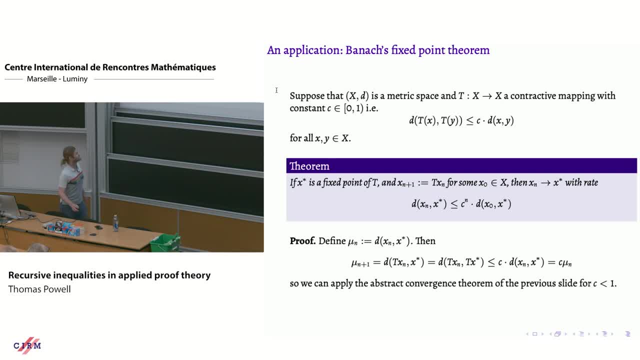 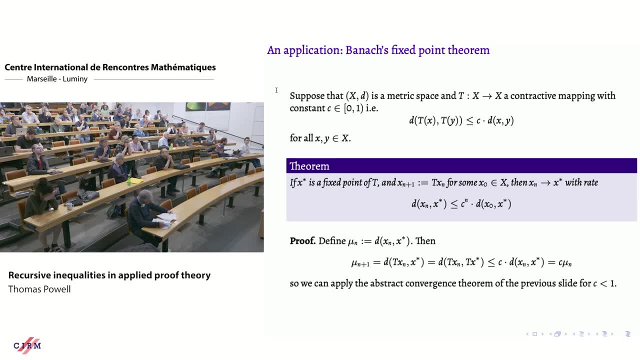 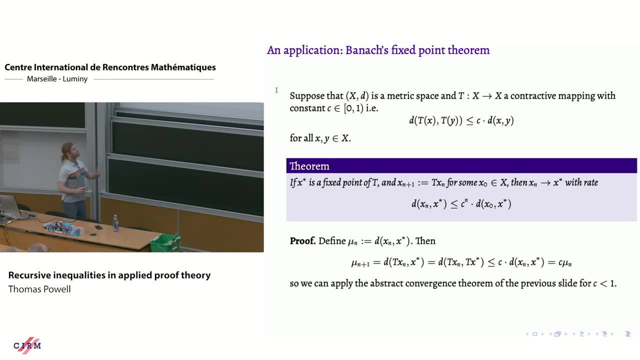 Okay, Just because if we look at the end, plus one element in the sequence, then kind of, because that thing is a fixed point, then it's a contraction of the nth, And so we just get, We just get. We get exactly this recursive inequality and the rate of convergence that we get from the recursive inequality is exactly the rate of convergence we get in benefits point theorem. 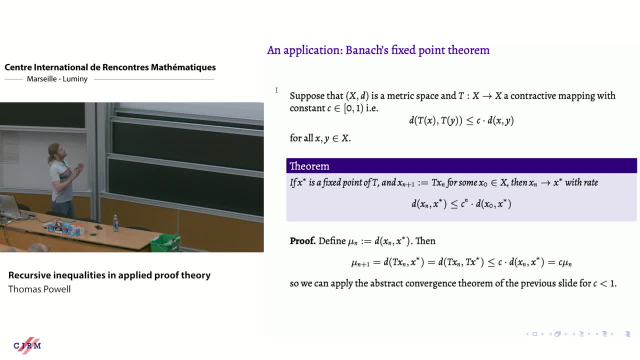 Okay, so the only point I'm making here is that this simple fact about monotone sequences of real numbers somehow underlies a theorem about metric spaces and non expansive mappings and things and contract of mappings. so there's a concrete, abstract mathematical setting that gets reduced to something much. 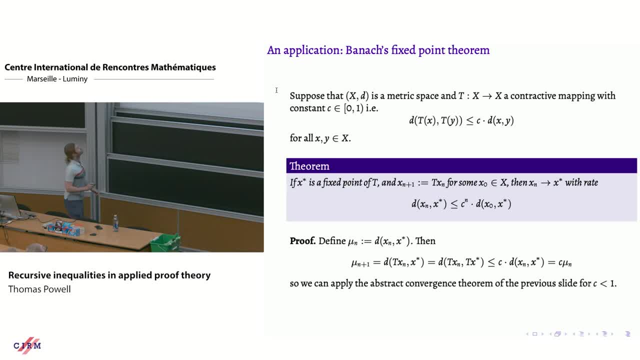 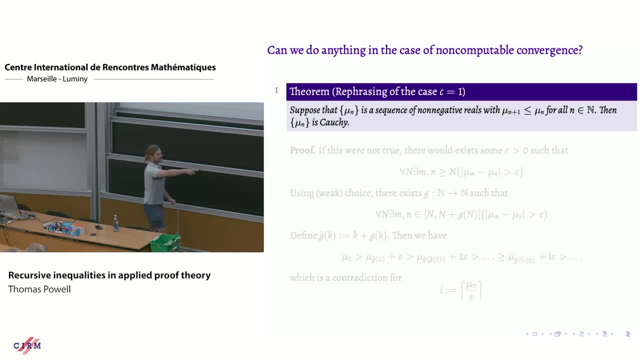 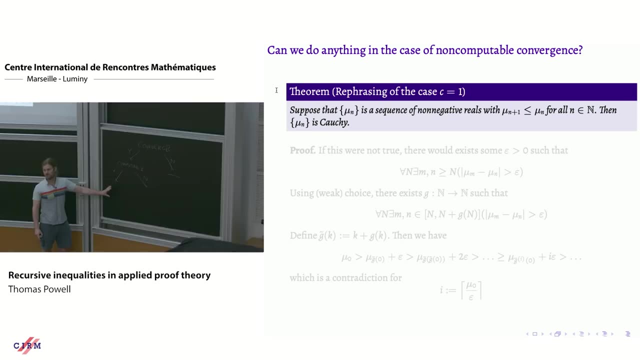 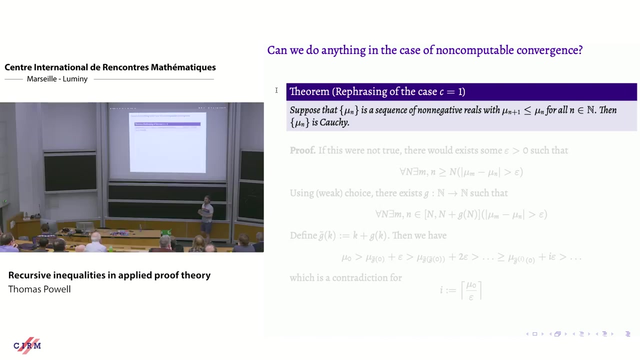 simpler to do with real numbers. So can we do anything In the case that we have non computable convergence? so if we don't have convergence, we're not interested in it. if we do have convergence and it's computable, that's great and we can use the rate in whatever setting we're in. so what happens if we have convergence but we don't necessarily know that we have a computable rate of convergence? can we get some sort of computational information out of that? nevertheless, 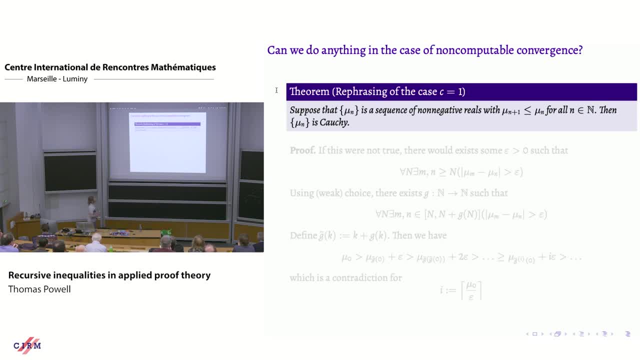 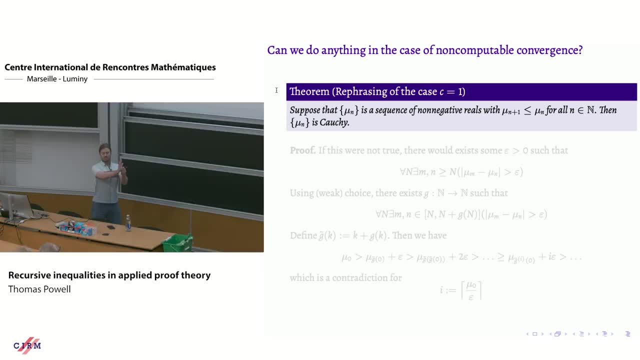 So The answer to that is yes, and it looks a bit weird. so this is a rephrasing of the case. equals one. so equals one is just that we've got A monotonically decreasing sequence of real numbers. we know they converge, but we're not quite sure to what. 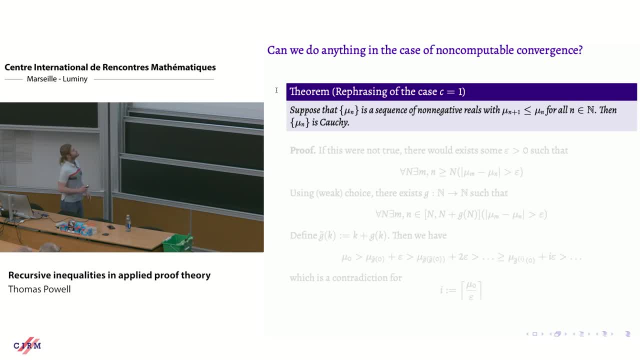 Okay, and that thing may not be even computable. so we can be formulate this: instead of talking about the limit, we can just say that that's a cushy sequence, right? so that's an equivalent formulation of this recursive inequality theorem. first equals one. here's a little weird little proof. 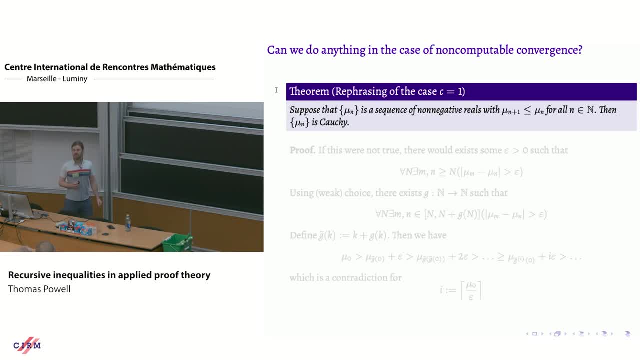 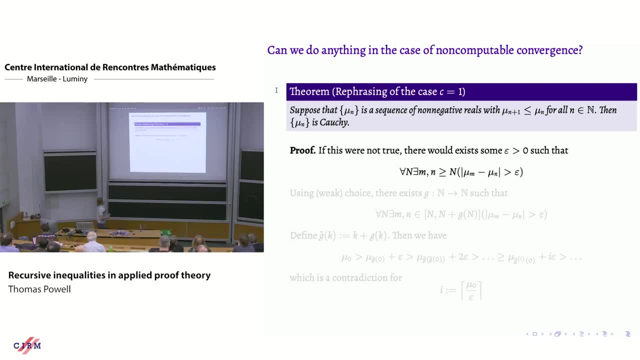 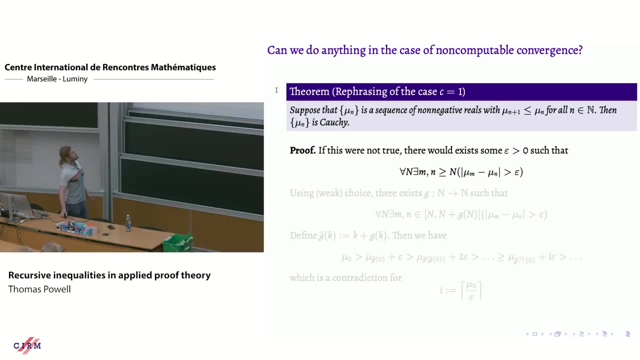 Of this fact. that looks a little bit proof, theoretic, and I'll explain where that's going in a second. so Why is this the case? well, If it's not true that a monotonically decreasing sequence of real converges or is cushy, then there would exist some epsilon, such that, for any point, we can find two things after that point that are bigger than epsilon apart. okay, so for any point, there's going to be two things that are bigger than epsilon apart. 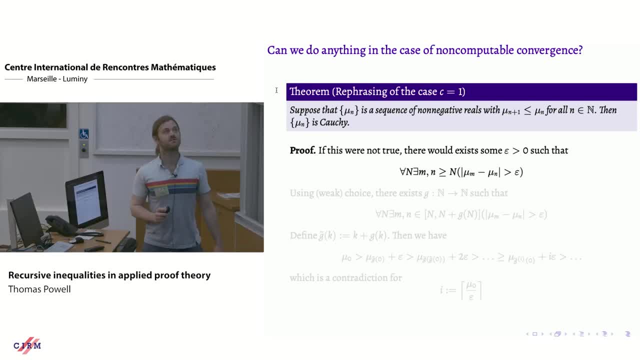 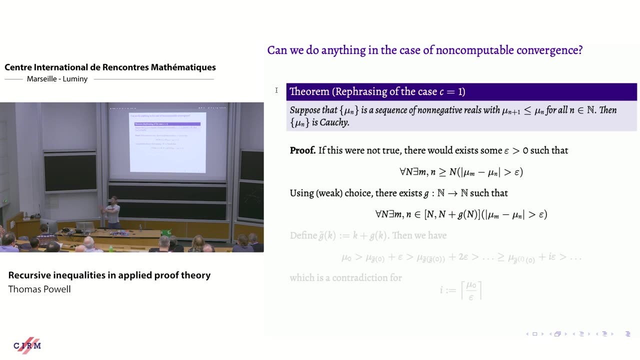 So that's just the, the contrapositive of the statement, that that sequence is cushy, the reasoning by a contradiction. And so now, using a little bit of logic, proof theory, there's going to be some choice function. right, If any n we can find two things after it that are kind of bigger than epsilon, we can find there's, there's, there's going to be some point at which we we stop looking. all right, so we have some choice function. 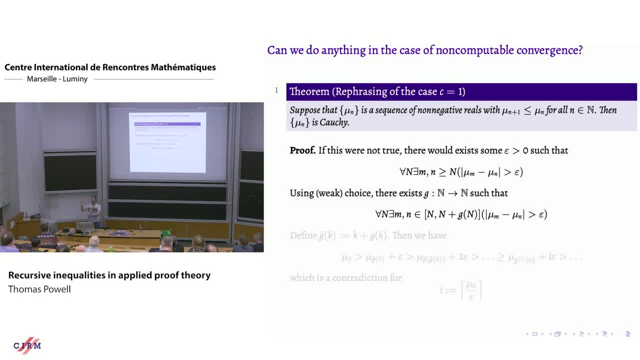 And so what we do is we just iterate. That's all right. so we start with the first element. at some point there's going to be two things bigger than epsilon, and then we go from here. we iterate again and we get that, we iterate again and we get that, and at some point our sequence goes below zero, which is not possible because this is a sequence of non negative real numbers- contradiction. therefore, the sequence is: 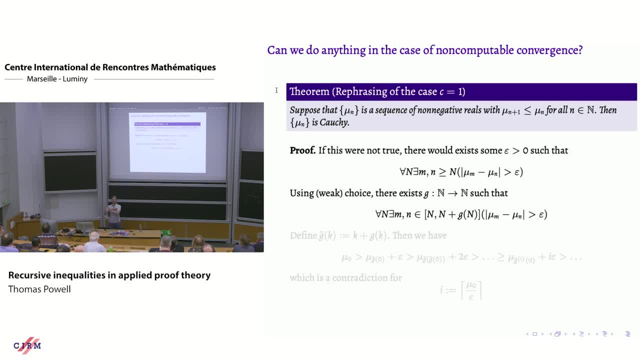 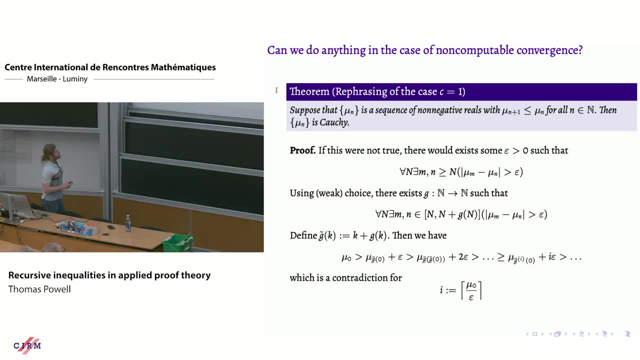 You probably won't see this sort of proof in a math textbook, because we know why would you be taking this g out and doing things like that and making it unnecessarily computational. Because what we've got here in this, in this form of proof we're actually each step- is very computational. we're saying, kind of, if we have a g that always finds the point where we've got two elements that are epsilon apart, we can iterate this and we know after a certain number of iterations when we must get this contradiction. so it's a proof by contradiction, but somehow a computational proof by contradiction. 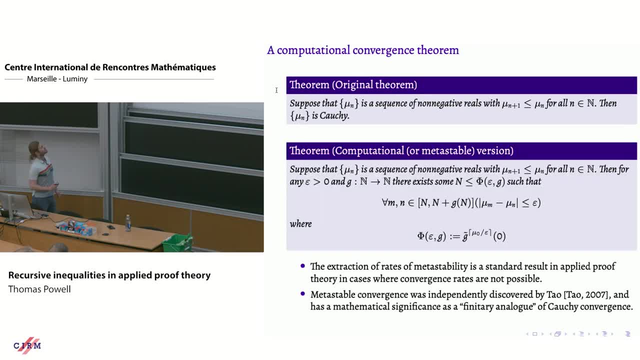 So what's going on? proof theoretically: Yeah. so just to state This: this is, this is, this is what we've achieved. so the original theorem just says: if we've got a monotonically decreasing sequence of of non negative reals, that must be cushy. we've got a computational version of this which is completely equivalent, which says that if we've got the same thing. 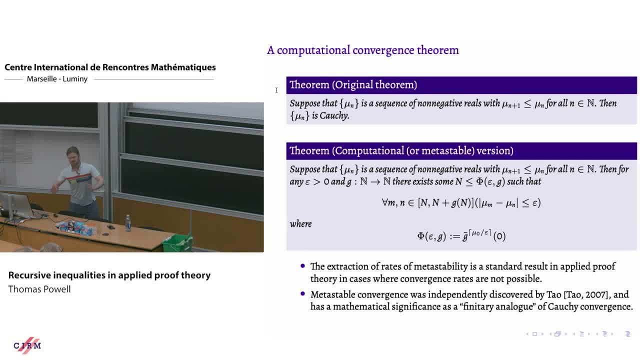 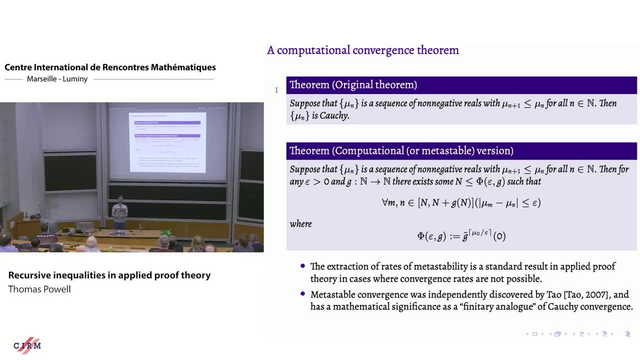 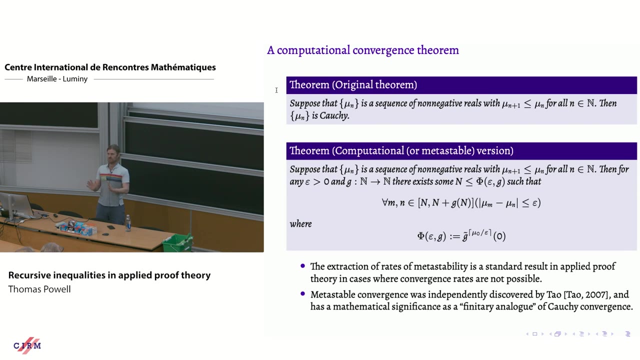 Then, instead of cushiness, we have this sort of metastable convergence statement where instead of saying that the sequence is always stable after a point, so always within epsilon after a point for any g, We can find Some sort of region where it's always stable in that region. so it's weird, it's a weird reformulation of cushy. convergence is logically it's equivalent, and in this reformulation we can come up with some sort of constructive analog, namely a bound on where we get this region of stability. 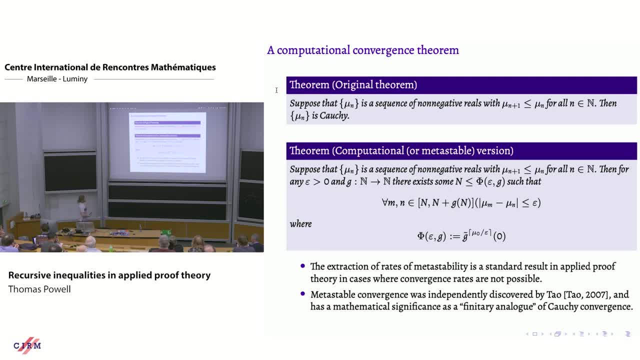 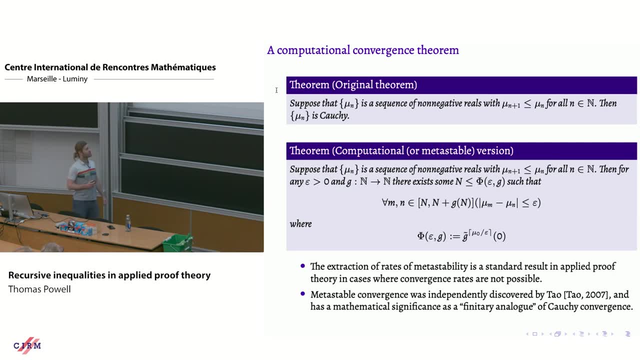 Okay, so the extraction of rates of metastability as opposed to rates of convergence is a completely standard result in applied proof theory, which we do whenever Convergence Rates are not possible, and explain why that's important in a second. they were also, really interestingly, independently discovered by Terence Tao, so he this was used in some of his papers, but he wrote a really nice blog post where we talked about exactly this sort of thing and its significance in ordinary mathematics. so this isn't just something that's a proof theoretic interest. it was independently considered by mathematicians. 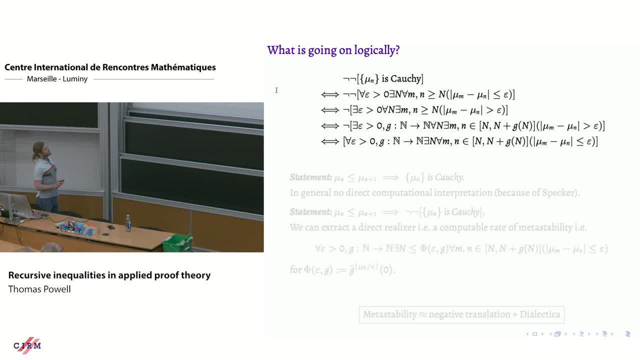 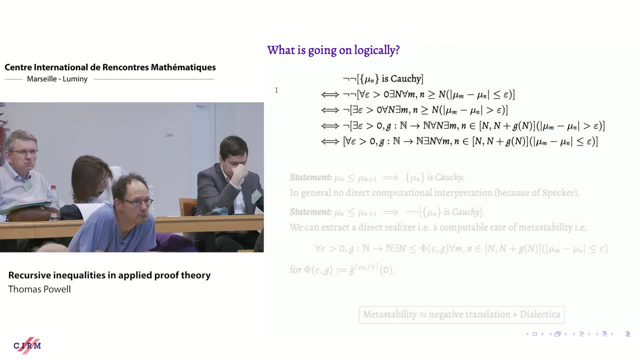 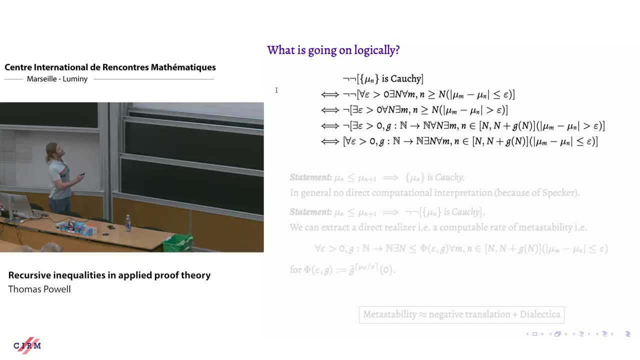 So what's going on logically here? so kind of This thing looks a bit weird, but I can Explain it in terms of what's wrong. she talked about yesterday monads and negative translations and things like that. okay, so we just do The double negation translation of the statement that a sequence is cushy. okay, so the second row here is just the fully explicit epsilon delta definition of being a cushy sequence. we put two negations in front of it and what we do is we just bring each negation into the interior one by one, so proving the first negation to the interior, the quantifiers flip. 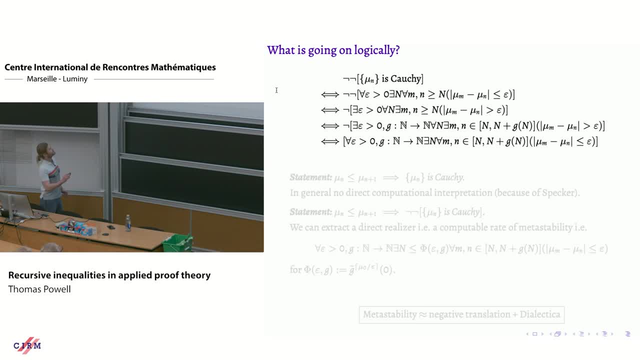 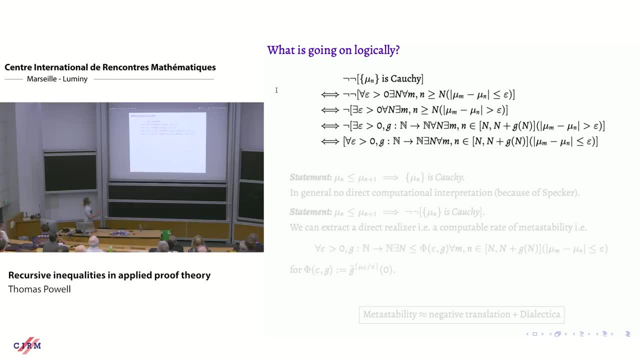 So that's the next stage: the for all becomes an exists, the exist becomes a for all, and so on. okay, So now what we do is, if we go on, exists for all exists, well, we know that there's going to be a bound on this exists and n, so we take that out as a function. so we're using a really weak form of the action of choice. and now we're saying that there exists an m n in this region here, so that's n up to n plus g of n. 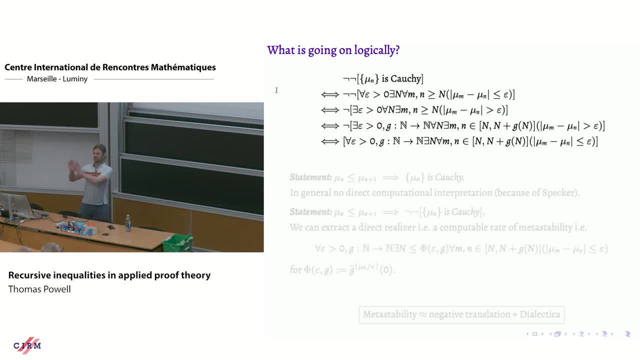 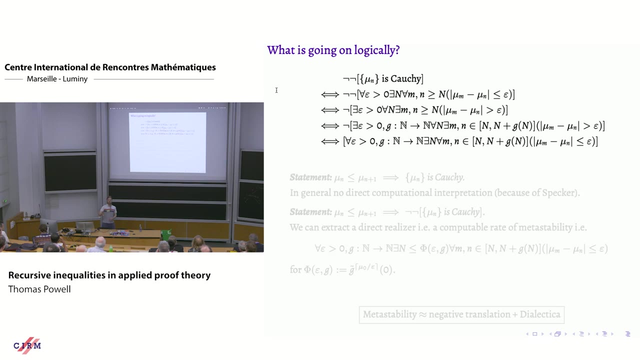 Where this is not true, and then all we do is we bring the second negation Back into the middle. the quantifiers flip again and we get for all epsilon and g. there exists an end, such that there is this region of approximate stability. so going from ordinary cushy convergence to this weird proof, theoretic looking statement is nothing more than applying a double negation, doing some manipulations on the quantifiers. that's it right, that's the proof, theoretic explanation. but the significance is the following: the significance is that our original statement that the sequence is cushy has injured 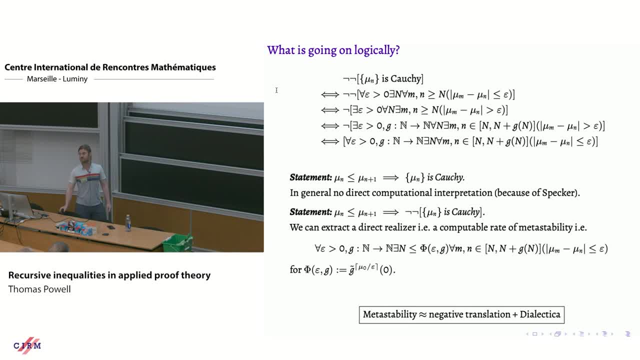 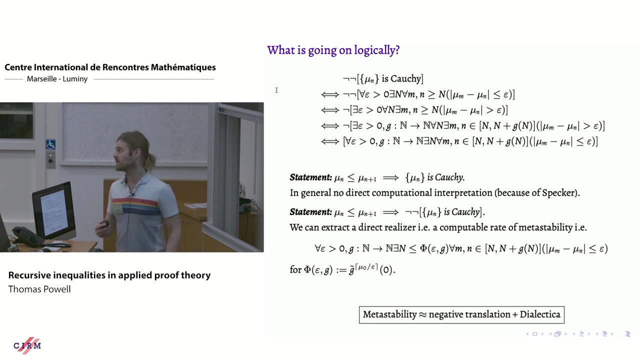 In general, no direct computational interpretation, because a direct computational interpretation of the statement that the sequence is cushy, convergence would be a rate of convergence, and the old result of specker says that we can't necessarily get that. okay, we don't necessarily always have that. on the other hand, a direct realizer of the double negation thing of this is exactly what we extracted here- is a bound on the existential quantifier and that's what's known as a computable rate of meta stability. so the phenomenon here is that if in general, you've got a statement that's proven, 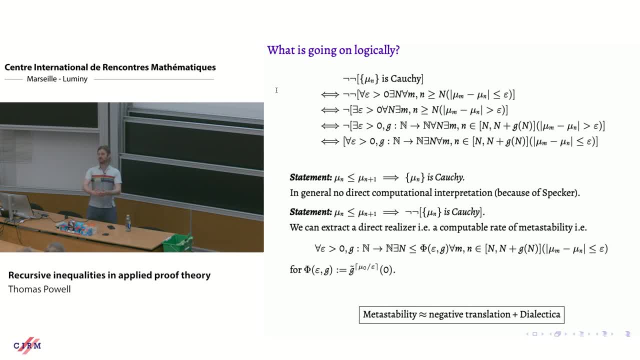 By classical logic you may not be able to get a direct realizer from it, but if you double negate it, do some funky business with the quantifiers, you can then often get a direct computational interpretation, and the idea here is that meta stability is somehow equivalent to the negative translation, plus dialectical, of the statement. I'm not going to go into the details of the dialectical interpretation, but for people who are interested in how that plays a role in this sort of area, it's essentially that we put some negations in. we do, and that's the 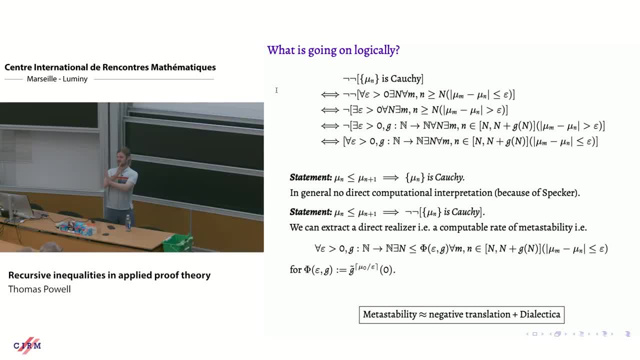 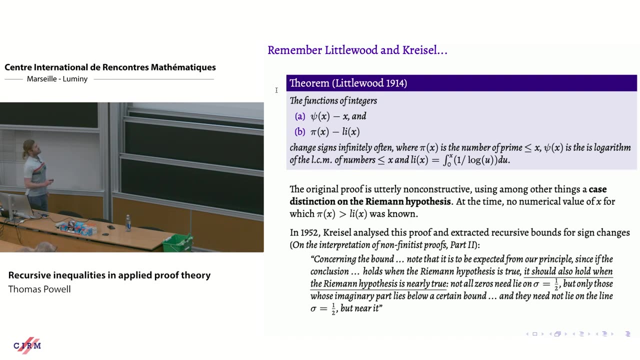 Double negative translation, and then we do some weird stuff with the quantifiers, and that's the dialectical, and if you do that throughout the proof, you have to end up getting bounds for some reformulation of the theorem. All right, so Back to little, which this is- this is just a slide from earlier in the talk. this bit, it should also hold when the Riemann hypothesis is nearly true. right, what we saw below, what we saw just above, is that we have taken cushy convergence. 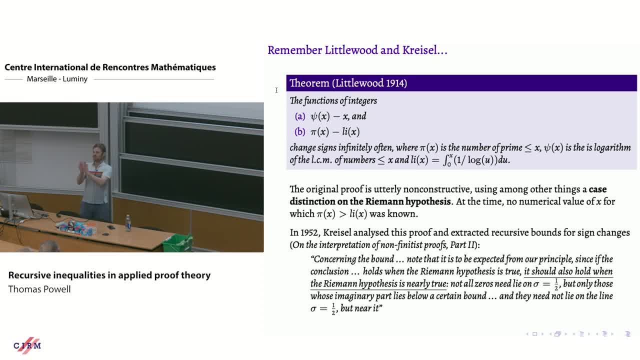 And we've kind of reformulated it into an equivalent but approximate form of cushy convergence. so rather than permanent convergence we've got sort of approximate intervals where you get stability. And this is exactly what the idea that underlies kreisel's original case study. so rather than taking the proper Riemann hypothesis, he takes an approximate version of the Riemann hypothesis and then the constructive information filters through the proof. so 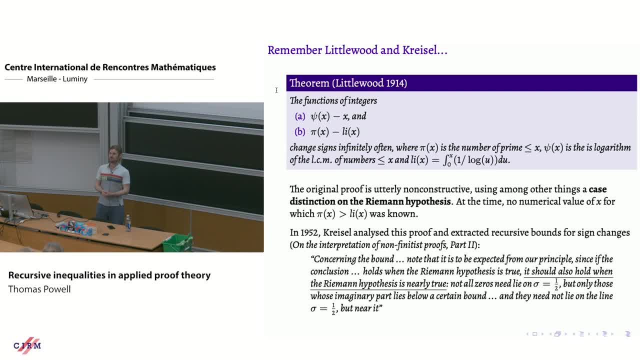 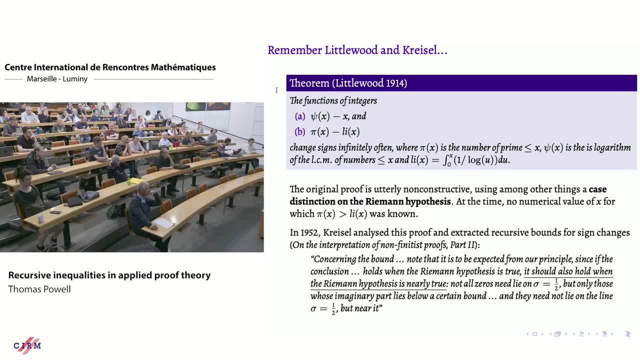 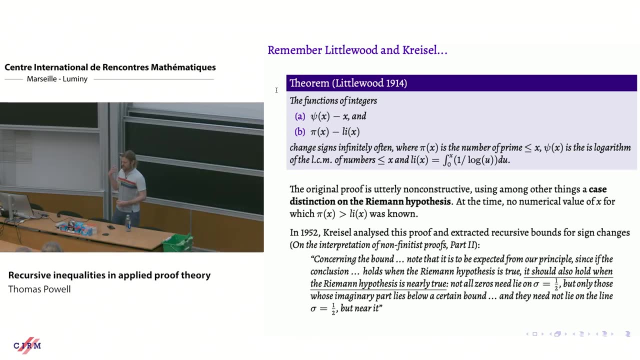 Kreisel wasn't using the dialectical interpretation. he was using, I think the that some some form of Epsilon calculus. But the idea is It's very complicit in all sorts of manipulate proof, theoretic manipulations of, of classical proofs, so replacing ideal objects with approximate versions of them. you know also in, in, in, in, in constructive algebra you see this without proof interpretations. if you've got the existence of a maximal ideal, you sort of convert that into an approximate maximal ideal. it's the same sort of idea you see in lots of different areas. 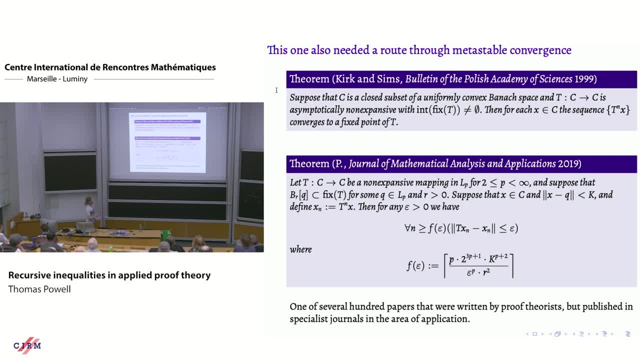 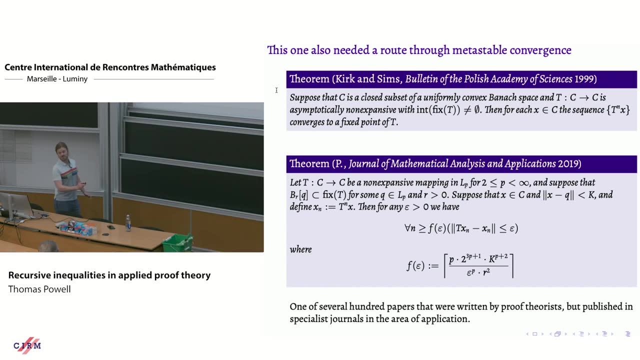 So In my paper I needed to go through meta stability to get this concrete results. Convergence property, a cushy convergence property. I needed to get the meta stable version of that convergence property and then from that one gets a concrete. this is called a rate of asymptotic regularity. so this is a very concrete result that doesn't use any sort of weird proof theory. but to get that concrete result one needed to go take the route via meta stability. so meta stability, meta stability is important because if you use 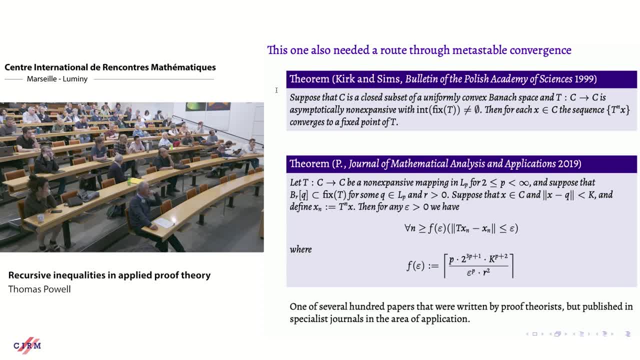 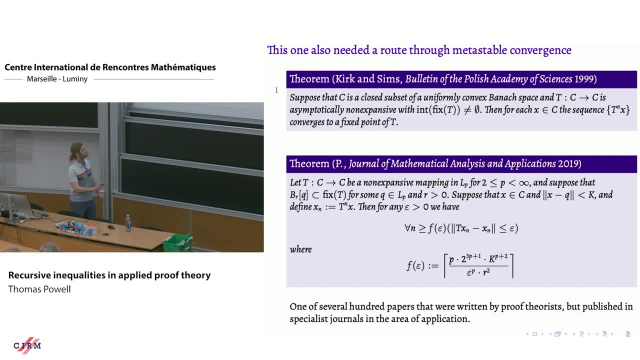 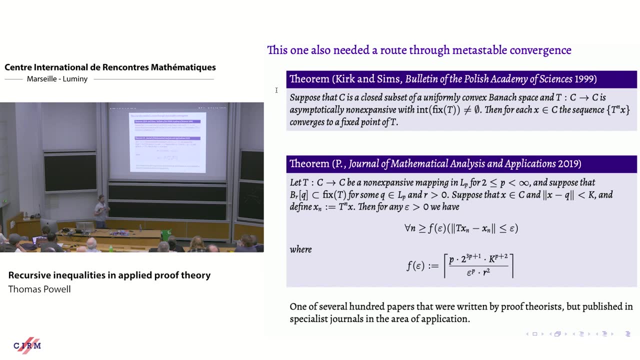 Convergence as part of a proof of something else. the meta stable version Allows you to get direct quantitative information, sometimes from the conclusion all right. so, even though this has nothing to do with proof theory, meta stability, choice or anything like that, one needed to go through meta stability to get that, and this is a phenomenon that happens again and again in applied proof theory. 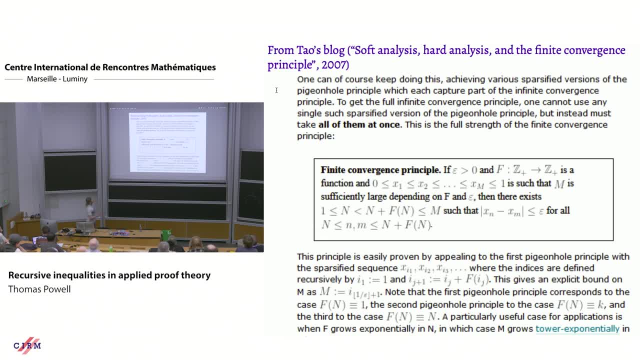 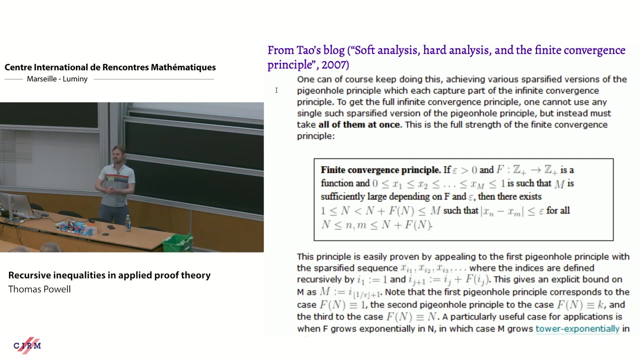 And then this- sorry this didn't come out very well, but this is just a screenshot of the blog by Terence tower and I really recommend this is super interesting because he's talking about A technique that was used for Example In these proofs that there are infinite arithmetic progressions in primes, where one takes some bit of analysis and looks at the final to reversion of this, and I remember when I was a master student, before I knew any proof theory, I studied some of these proofs. there was a course on this and they used to form a finite for your analysis, which is really interesting. 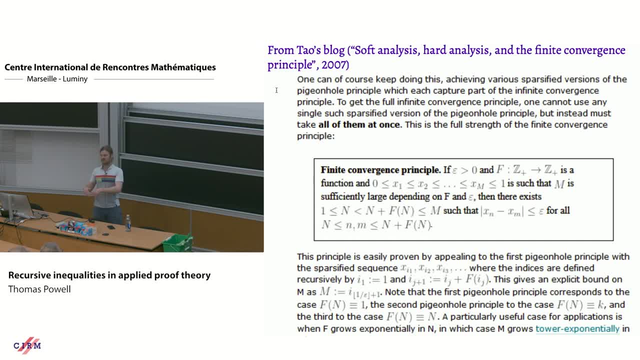 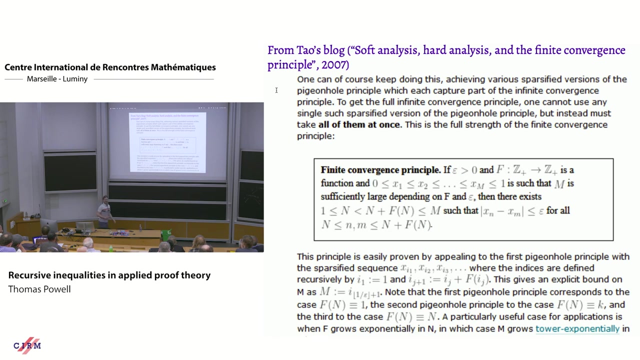 And so this blog post is talking about this, this process of taking an infinite tree statement and analysis and giving a final tree analog to it, and it explains where it's used, why it's important for mathematicians, and the example that he uses to illustrate this is exactly meta stability. so this is just sort of a mathematical reformulation of what it means to be kind of a meta stable sequence, and logically it's equivalent to being cushy convergence. so this was independently identified as useful from a mathematical perspective and actually at the end of this blog post, if you look at the comments, a bunch of proof theorists that said, yeah, but we know this, and so there's a little bit of a dialogue there. it's really nice anyway, 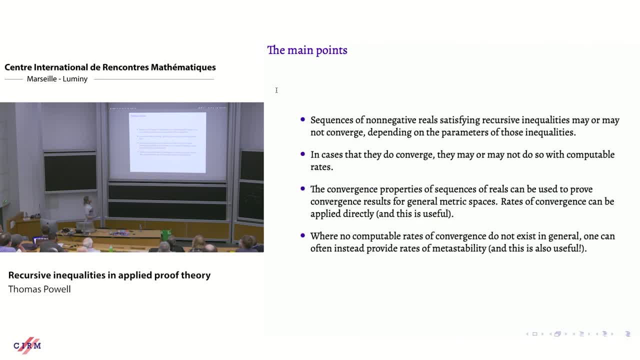 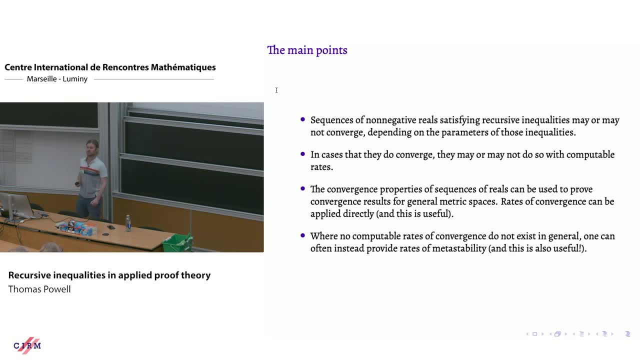 So, So So. The main point in all of this is the following: so, sequences of non-negative real satisfying recursive inequalities: they may or may not converge, depending on the parameters. where they do converge, they may or may not do so with computable rates. 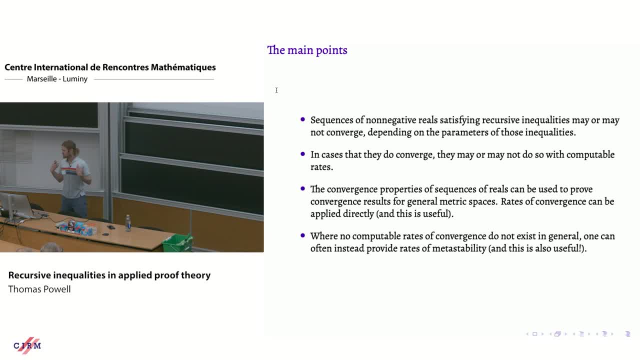 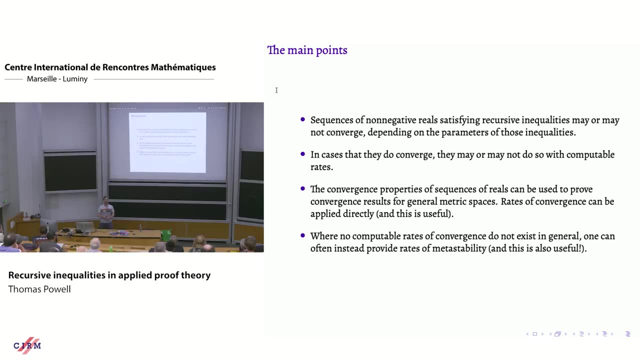 The properties of these sequences can be used to get general convergence results for metric spaces or whatever, like Banach fixed point theorem, and when convergence rates of convergence exist you can apply those directly. And when no computable rates of convergence exist, one can often instead provide rates of meta stability, and those are also useful. they're useful if you're an applied proof theorist and they're also relevant sometimes if you're a mathematician. 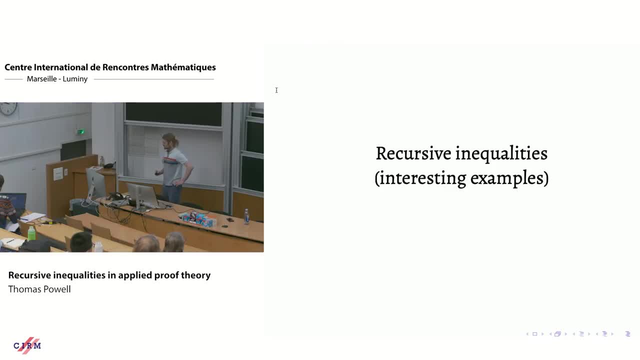 So those are the main points. So I'm now going to give some more examples of recursive inequalities and I'm getting to the stage of the talk where I'm going to have slides with a lot of mathematical detail, but I promise you that's not relevant. I really mean that all I want to do is point to bits and just explain. 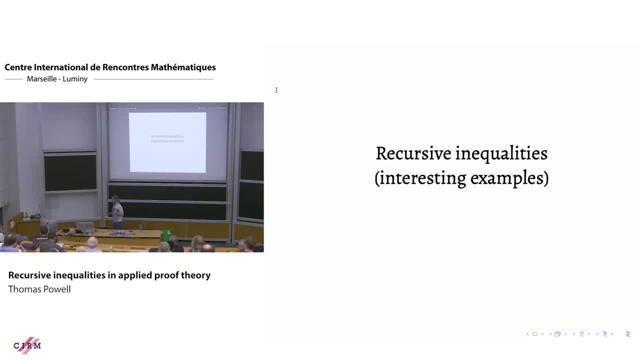 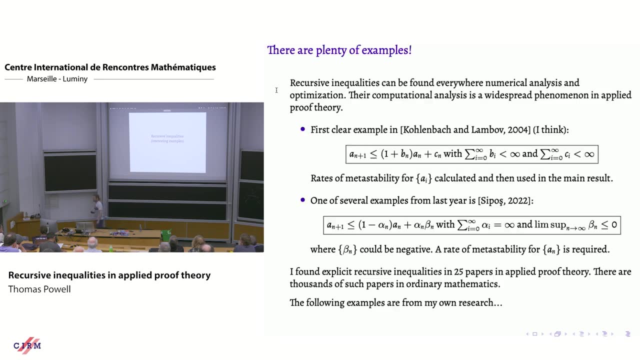 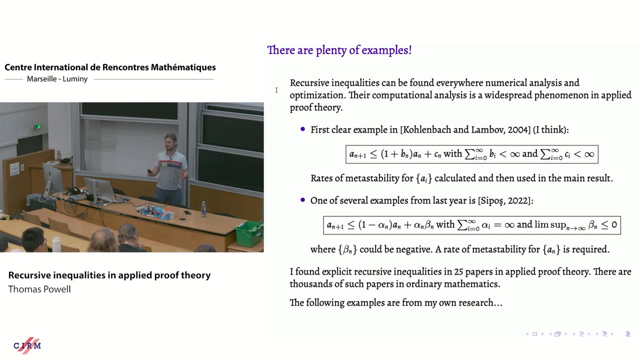 Kind of A How these recursive inequalities emerge in ordinary mathematical settings. Okay, so there are loads of examples to choose from. so recursive inequalities are everywhere in numerical analysis and optimization. I mean there's literally thousands of papers that have these and use them Where you want to prove the convergence of some algorithm to some minimizer or some fixed point or some solution to a differential equation whatever, and in order to establish convergence. 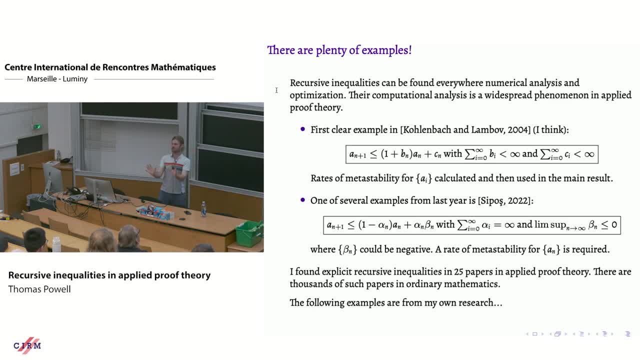 You look at the complicated setting, you reduce everything to a simple property of real numbers, where the real numbers in question are always the distance between the algorithm, the individual points in the algorithm and the point you want to approximate, And then you see what kind of recursive property they satisfy, and then you apply some sort of abstract convergence result. this is a really really common trick in optimization in other areas to establish convergence, and so, you know, in applied proof theory. 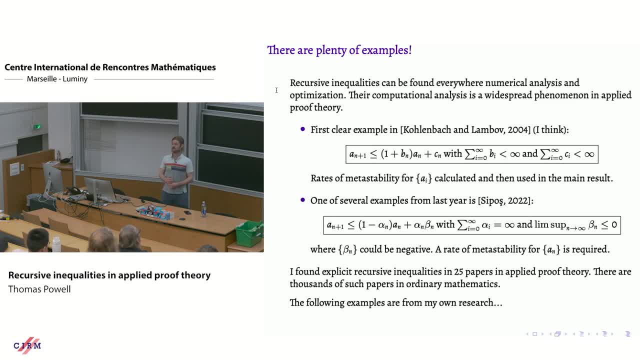 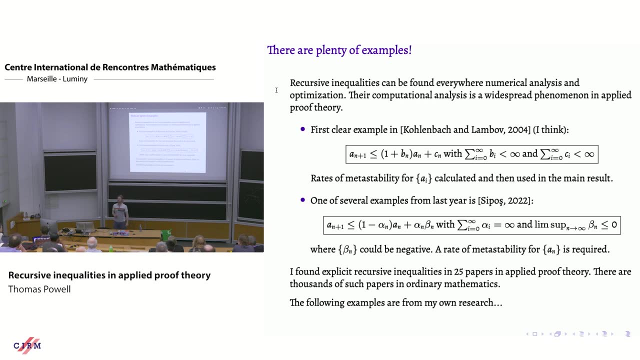 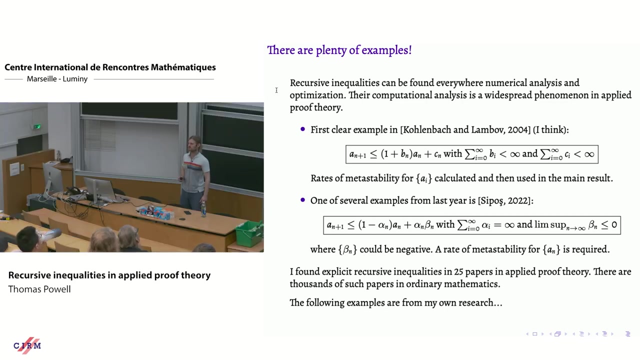 The computational analysis of recursive inequalities in general has proved to be really important. So So, So, So, when I was doing this project with my PhD students- because our main, our main topic was recursive inequalities- I felt I needed to understand the full extent of their use. so I applied proof theory is one of those areas where it's it's it's still small enough that you can know about all the papers. you can, in theory, look through all the papers in the area, and so I look through all of the papers, and there are about 25 of them that use some sort of computational, some sort of computational study of an abstract recursive inequality. so I think the first was in 2004.. 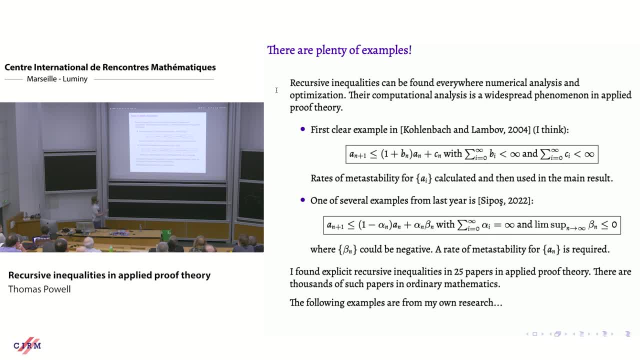 And that's what it looks like. so it's kind of a bit more complicated than than the monotone case and there's some other conditions and that's very typical. and then there are tons of examples last year. here's another one. it's slightly different and there's some some some properties. here is just wanted to kind of give you a general idea of what recursive inequalities look like in in the more interesting setting. yeah, so, like I said, there's a bunch of papers in applied proof theory that studies these explicitly and thousands of papers in ordinary mathematics that uses them. 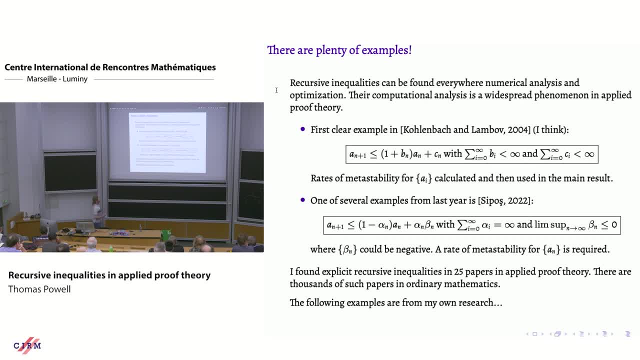 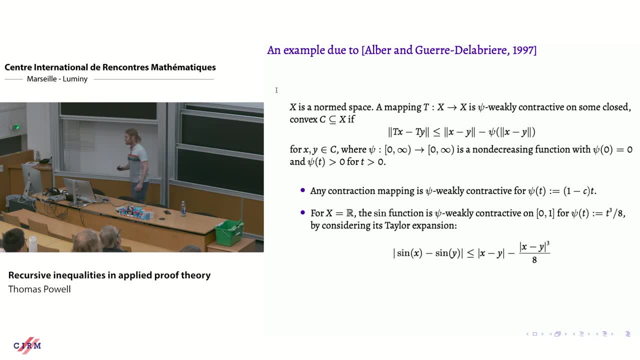 And So I'm going to give some concrete examples, and these are from my own research. well, they've been studied. so here's an example from: I mean, these aren't these, these people on on on logicians or proof theorists? they're just analysts. So 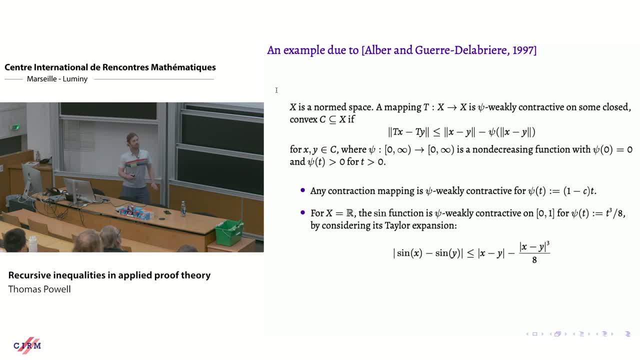 The details are not important. all I want to do here is is is point out that, if you know what a contractive mapping is, this is just a slight generalization of what it means to be a contractive mapping. okay, So it's a slightly 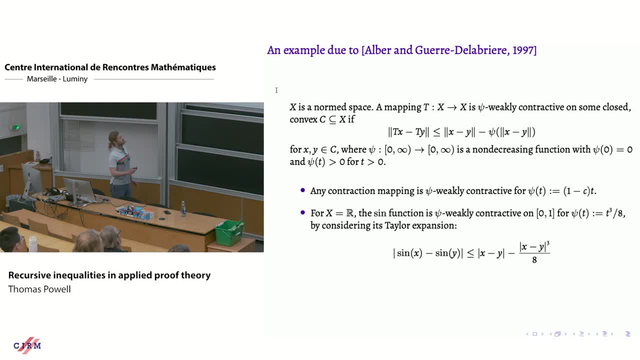 We could property and so things like the sign function satisfy this All right. so they studied this particular kind of mapping aside- weekly contract of mapping and it's just a generalization of what it means to be contractive. But I fixed point theorem. it doesn't apply. but one can prove that these things converged to fixed points using a slightly more sophisticated proof. 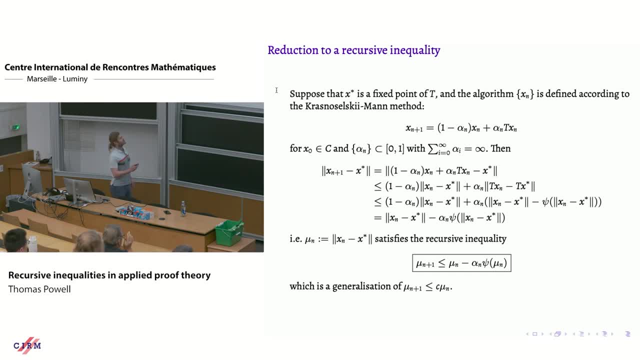 And there are various different algorithms as well. so, rather than just using the, The so-called Picard iterate, which is where you take the first point and you repeatedly apply the mapping to it, you can also do weird things like that. you can take linear combinations. 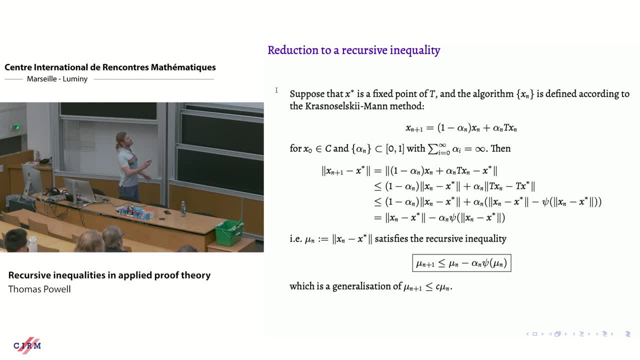 Of mappings- and you know these are really important- and optimization and often you can show that you get better rates of convergence for particular choices of the step sizes. but the long and short of it is that you have a general kind of mapping, you have an algorithm, you do a bunch of sort of elementary manipulations which just use properties of 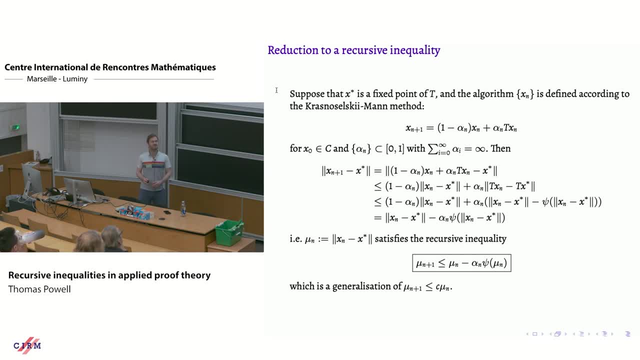 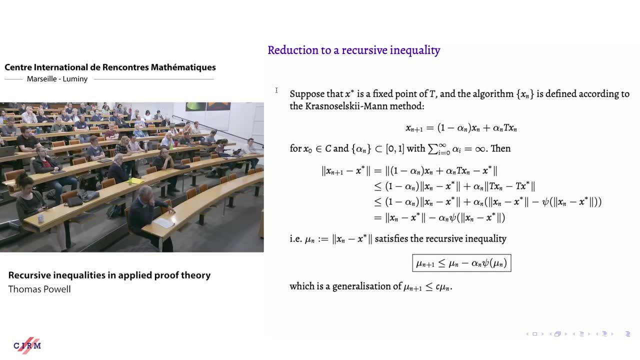 Of norms like the triangle inequality, stuff like that, and you end up with a recursive inequality, a slightly more complicated recursive inequality in comparison to what we saw before. All right, so that's all I'm trying to convey on these slides is that in more interesting settings, 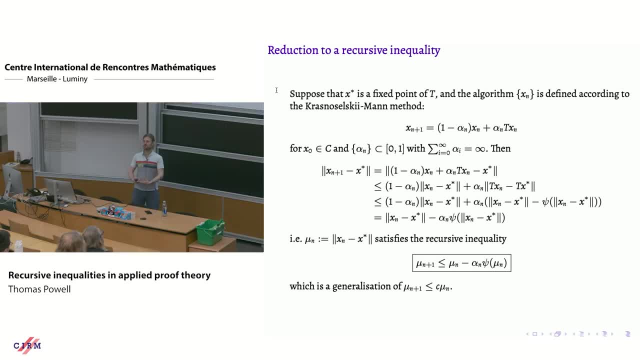 You often do still get recursive inequalities, but those recursive inequalities are going to be a bit more complicated. they're going to reflect the setting that you're in and they're going to involve components that are in your settings. if you, if you Modify The algorithm so that you've got step sizes, than the step sizes are going to feature in your recursive inequality. 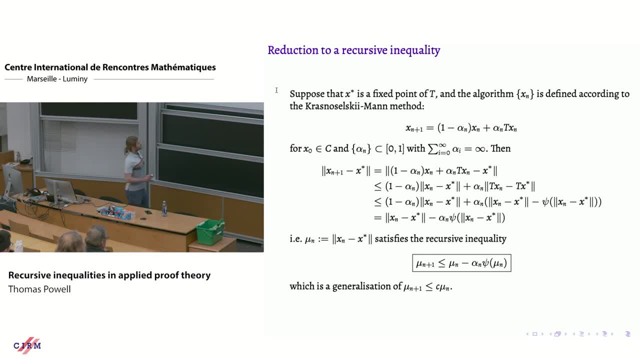 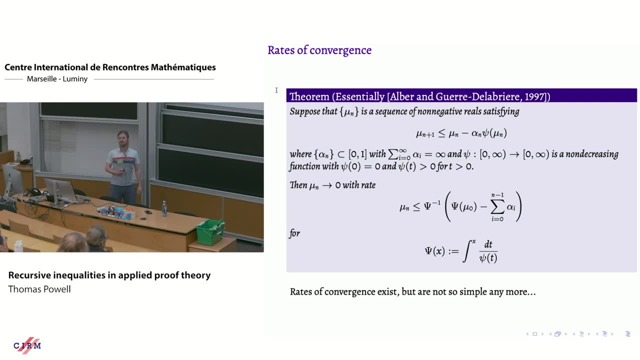 So the question is: well, does this converge? And the answer is yes, But the rates of convergence is suddenly no longer obvious. all right, so with with the banner, recursive inequality: if C is less than zero, you know if you've got a contraction, you know that C to the end is going to be the rate of convergence, or a rate of convergence is not difficult to see that. 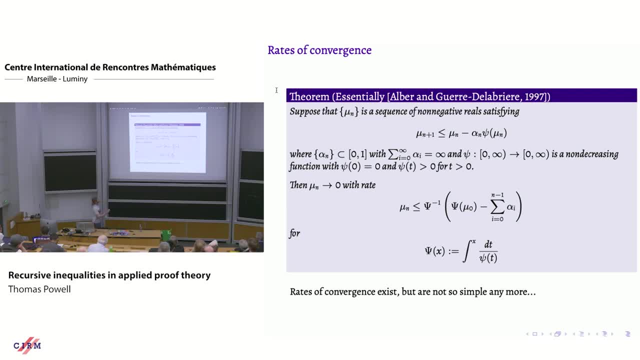 A slight modification of The Request, The Request of inequality, to something like this, and the rates you start to see in the mathematics literature are no longer elementary. you can no longer just stare at that and see that's obviously what the convergence rate would be right. so here we're using things like the inverse function theorem. we've got some integrals, you know a bunch of properties that show that this thing converges to zero as n goes to infinity. so it's no longer completely obvious. that's the only point I want to get across, right? 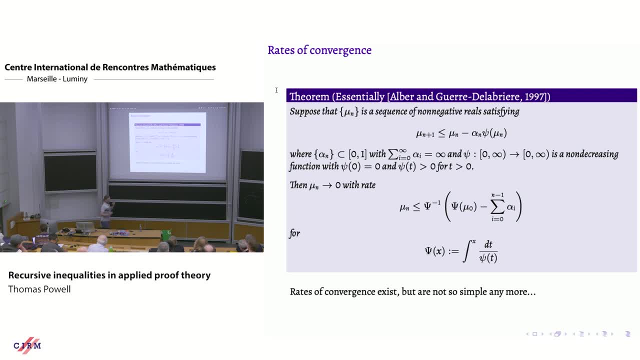 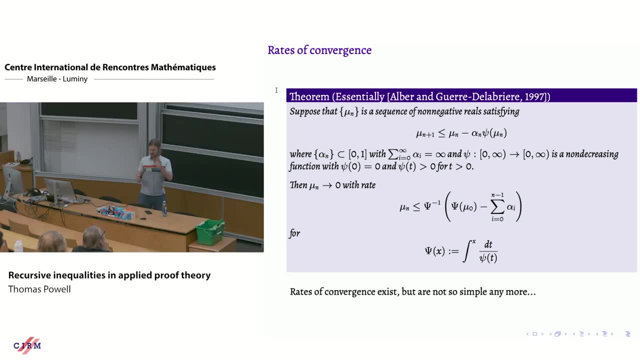 And what's more interesting is that at some Point Analysts stop giving explicit rates of convergence because it becomes a bit too complicated. like it's it's, it's just no longer obvious how you get those rates of convergence from from the recursive inequality. so 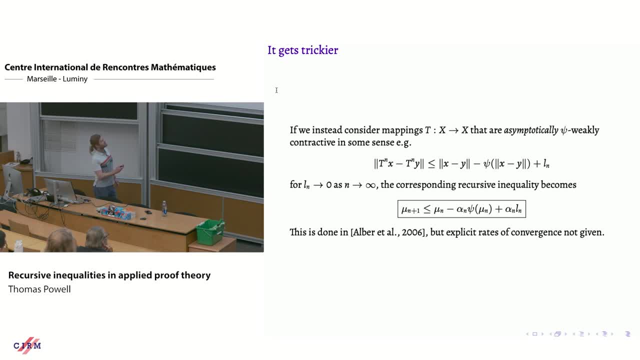 You know there's a slight generalization of this notion of being a sigh weekly contractive mapping. that just says it's asymptotically so. so rather than just being Contractive, it says that kind of in the limit it's contractive, so you have some error term. all right, so error terms are. 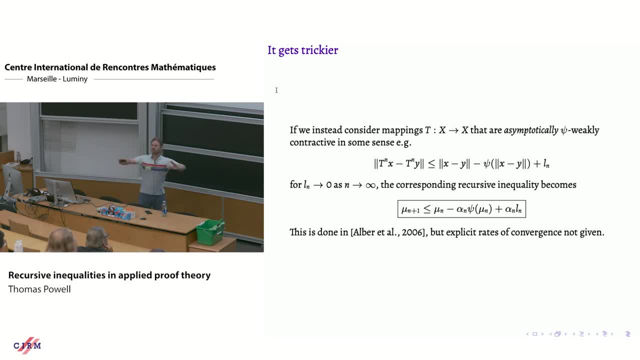 Obviously, really, really important- and optimizations. if you add an error term, it roughly be in the limit. it becomes a weekly contractive mapping. You can still show that the usual algorithms converge to a fixed point and that fixed points exist, but the recursive inequality you get then involves an error term as well, and 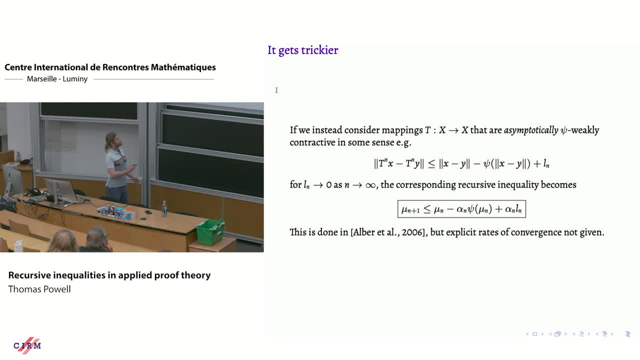 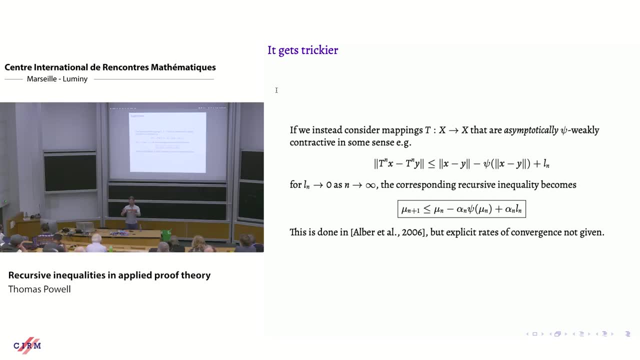 Normally when things like this are encountered in the literature, explicit rates of convergence are not given. so is that you know? I've seen lots of papers where they have this recursive inequality And they say They say, okay, in special cases we use this integral rate of convergence that we know exists from from the other paper, but in general we're just not going to give them. 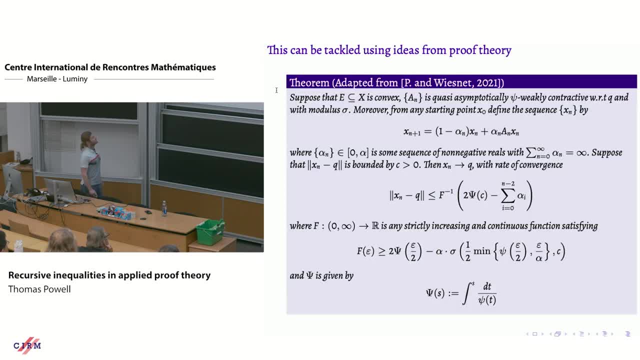 They can be given, and This was a paper that I wrote with Franciscus reason. it's where we looked very carefully at the proof theoretic structure of these convergence proofs and came up with a generalization that did give an explicit rate of convergence, and you know I've talked about this elsewhere. I'm not going to go into the details, but 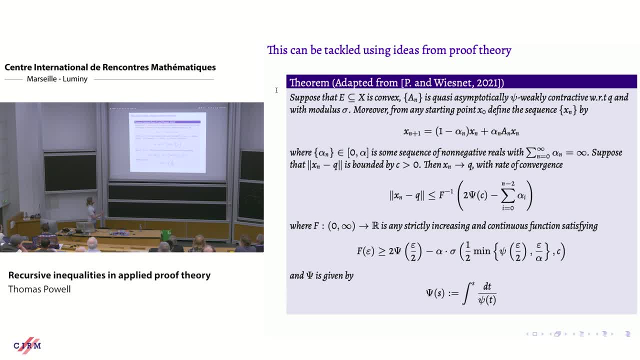 The point is that we were able to give A very general class of mappings and give a slight generalization of that rate of convergence that existed in the literature. that also applied to asymptotic variance and a bunch of other things as well. it looks similar but it's a bit more complicated, and the key thing here is that we arrived at that by using sort of a careful proof, theoretic analysis of the underlying convergence proofs, many of which use classical logic. all right, so that's the only point I want to make, that 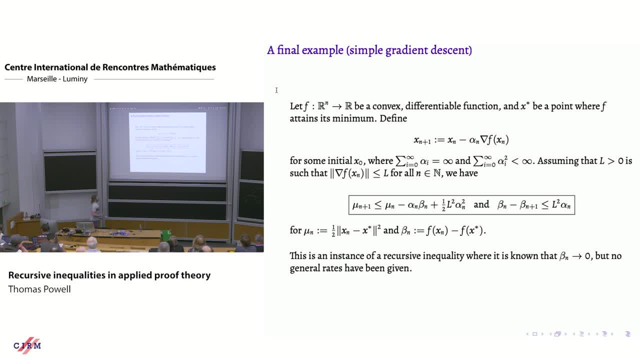 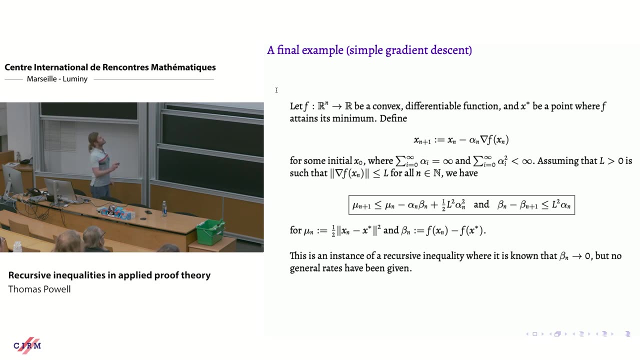 There are other examples Of recursive inequalities where No kind of rate has been given from the recursive inequality. so I mean there's, there's, there's a is everywhere now. so here's, here's, here's a simple gradient descent algorithm One can show. one can show that simple gradient descent algorithms satisfy these recursive inequalities. the details aren't going to be interesting, but I just wanted to point out that if you have gradient descent, you can show that these recursive inequalities are satisfied. 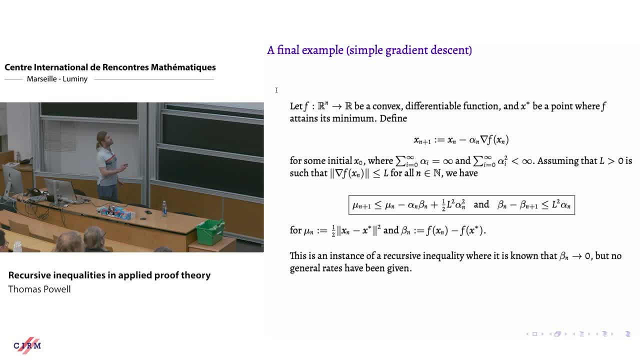 In the literature that say that whenever we have a recursive inequality of this form, with this little condition, here The beta n converges. In other words f of x n converges to f of x star, where that's the minimum of the function. But 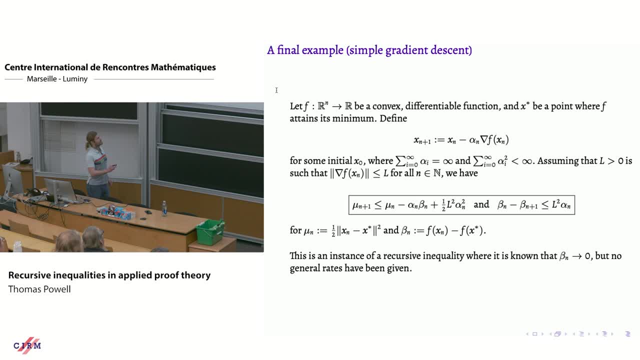 The lemmas that state that all recursive inequalities of this kind converge. not only do they use classical reasoning, but they never provide rates, which looks suspicious. Okay, so those are just a bunch of examples of recursive inequalities in the literature. there are, like I said, sort of twenty five to thirty papers in the proof mining literature that have used a quantitative analysis of recursive inequalities to get some sort of computational information from a general mathematical theorem. 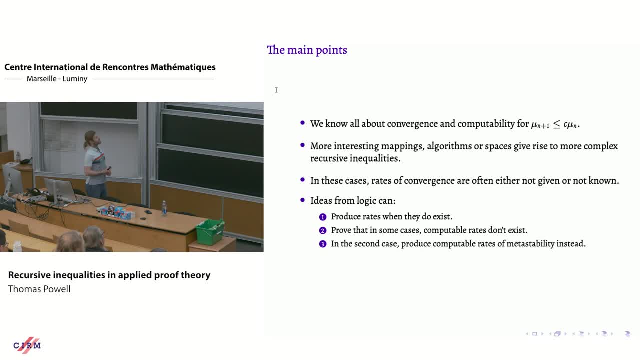 And using ideas from logic you can do one of several things. so Sometimes By looking at the proof, You Actually get rates of convergence. They weren't stated in the mathematical papers. but if you, if you kind of carefully look at the proof, theoretic structure of that proof, you can often generalize them and give more generalized rates of convergence. 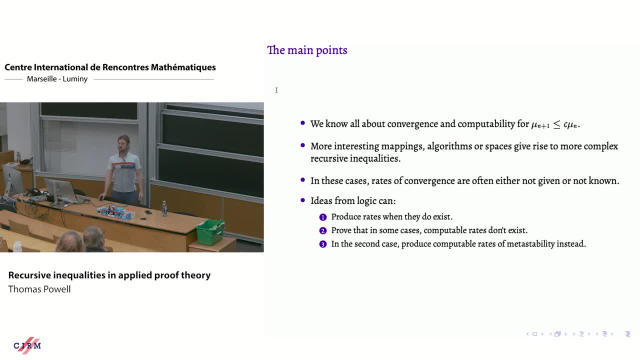 You can also prove that in some cases computable rates don't exist. and that's interesting because then you explain why in certain cases, you know the mathematicians who've been proving these results just say, well, yeah, we don't have rates of convergence in this case. 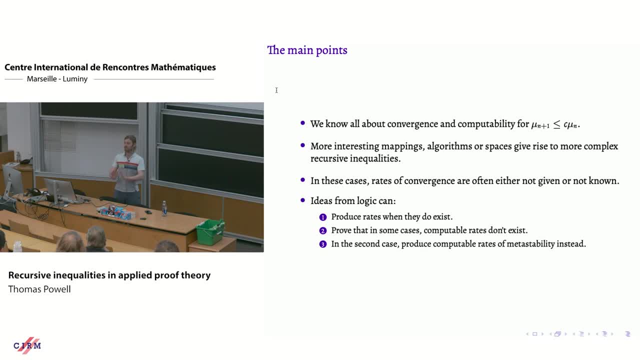 You can actually say why that wasn't possible, why, by looking at the proof, it wasn't possible to get computable rates, and then in this case one can produce computable rates of metastability instead very often. So I finished at quarter past, right, Yeah? 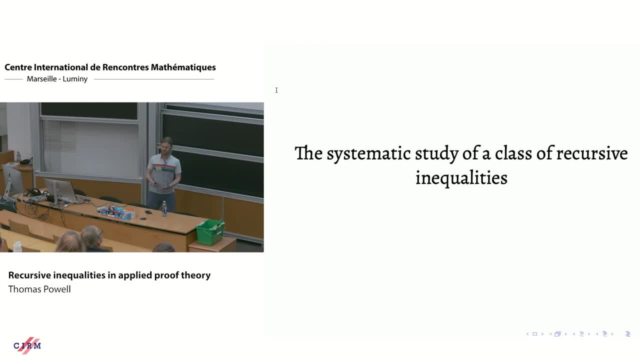 Okay, so I'm going to go very quickly through. so I presented the main idea of recursive inequalities and why they're important, and that was sort of the one of the main aims of my talk. so I just want to just flash them things that we did. 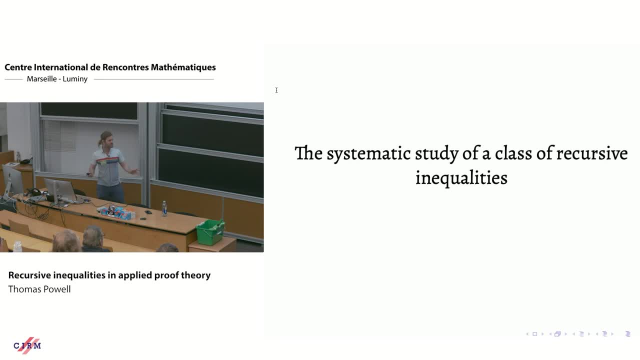 In the paper just to show you, and then I'm happy to talk about these with anyone afterwards. so the idea of a project was a systematic study of recursive inequality. so rather than taking a problem, reducing it to the recursive inequality and studying that, why not look at a general class of recursive inequalities and ask general questions about when do they, don't they, converge, when do we or don't we have rates of convergence and can we produce them? and if not, can we produce rates of metastability? 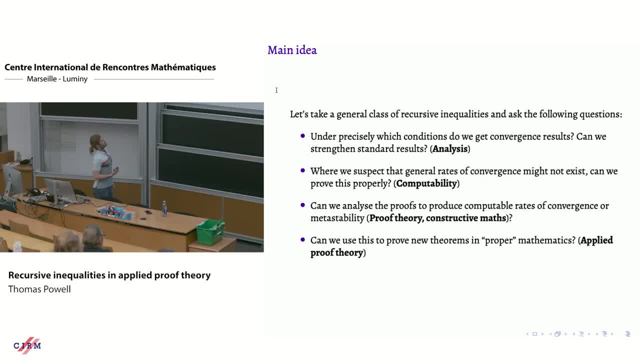 So this was the project. so we look at a general class of recursive inequalities and ask: when do we get convergence results and, if so, can we strengthen those results? If we suspect that general rates of convergence don't exist, can we prove this, Can we analyze these produced proofs and produce either computable rates of convergence or metastability, and then can we use this to prove new theorems in sort of proper mathematics that talk about things that may be gradient descent algorithms. so 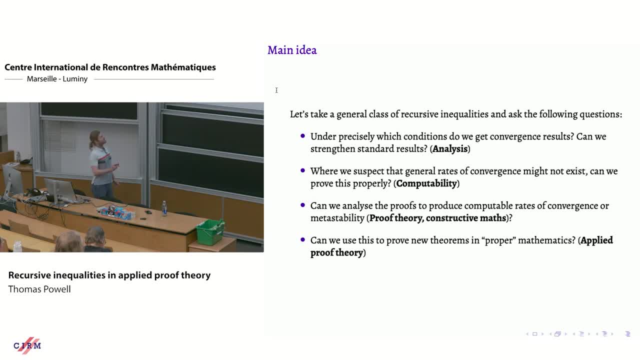 This is a nice project because it brings you through sort of elementary analysis, computability theory, proof theory and constructive maths and also applied proof theory, and that's why I worked on it with my PhD student, because it also gave him a tour of all of these different areas. it was a really nice project to work on, with somebody just coming into into into applied proof theory. 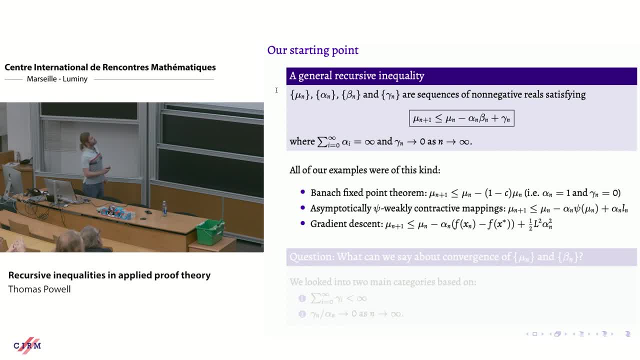 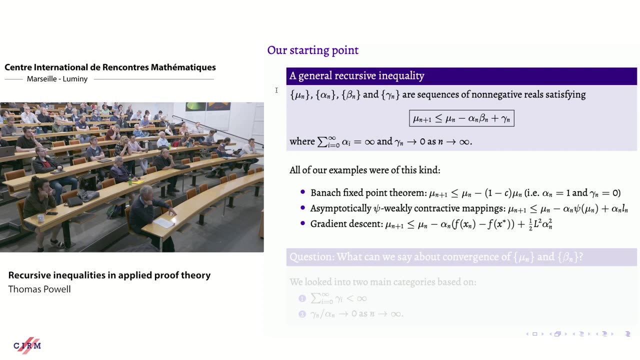 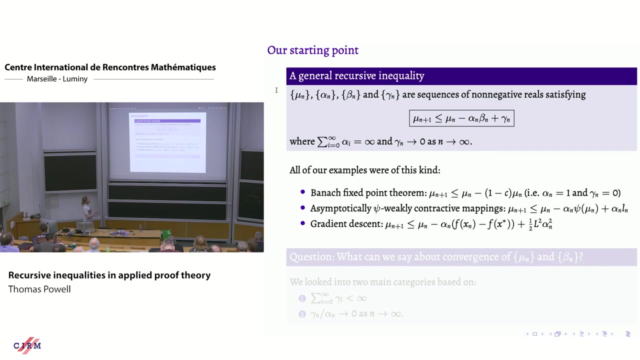 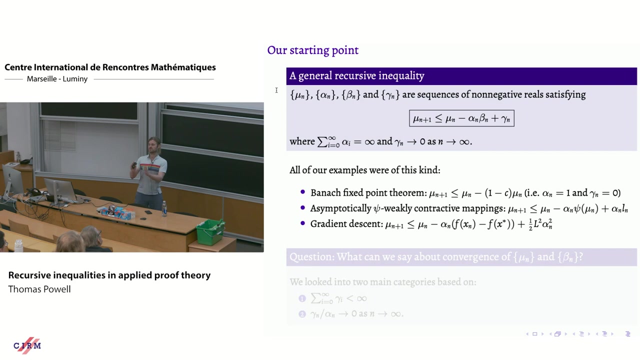 So what we looked at in this paper were sequences of non negative real numbers satisfying this very abstract recursive inequality, And all of the examples I gave are instances of this recursive inequality. So the alpha typically always step sizes and the gamma are typically error terms. now this alone is two weeks. so you don't get convergence of anything here with just those conditions. but if you add further conditions then you do get different classes of convergence results depending on which conditions you add. so what we were doing in this paper, we're just looking at the different classes you get depending on different additional conditions, and so the main two categories we looked at were when, rather than 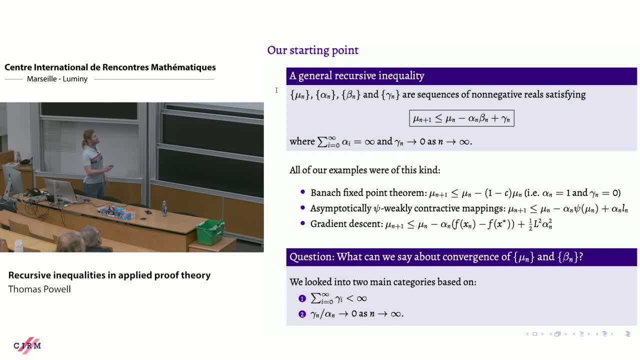 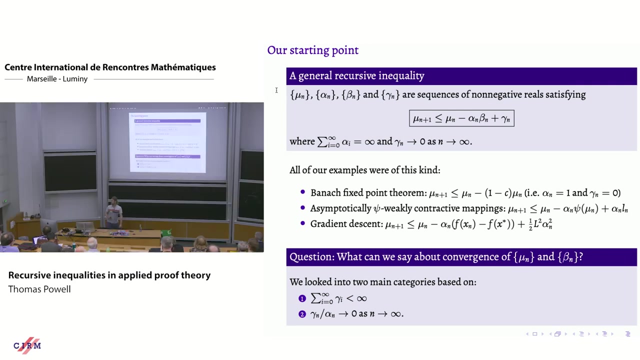 The gamma converging to zero. the infinite series generated by the gamma converges which is stronger, and the second one was that the gamma divided by alpha converges to zero. so each of those two things- and that allows you to say stuff about the convergence of mu or the convergence of beta, and so we just studied that quite systematically and try to establish exactly what you needed to prove convergence and when and when you didn't get rates of convergence. so I'm just going to flash a bunch of results to show you what sort of thing we're doing. so 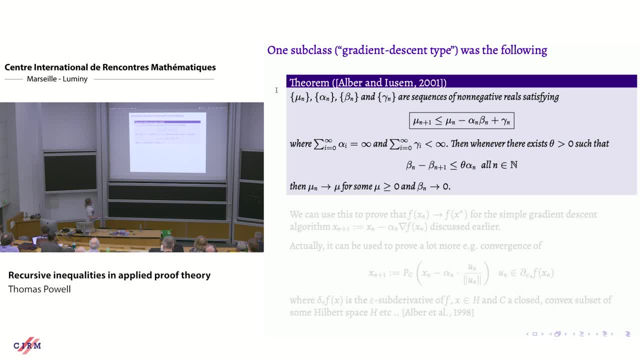 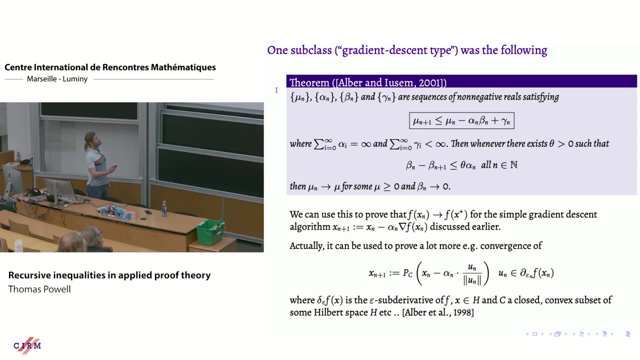 You know, one subclass of this recursive inequality is really important in proving convergence of gradient descent type algorithms. so you know, for the simple gradient descent one can show that it reduces to a special kind of this, this kind of recursive inequality. but there's really sophisticated gradient descent methods that also reduce to this recursive inequality and that's primarily where it's used is to establish the convergence of kind of quite complicated gradient descent methods. so I'm just putting that there just to show you. 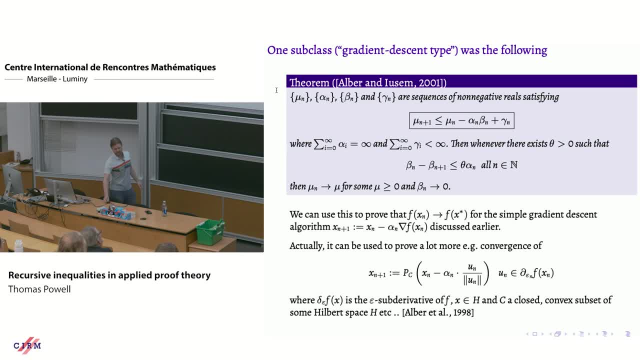 That you can generalize these quite interestingly. you know, instead of looking at the derivative, you can- if you've got a convex function, you can look at the, the, the sub derivative, or you can look at an approximate version of the sub derivative and then recursive inequalities are really important for establishing convergence. 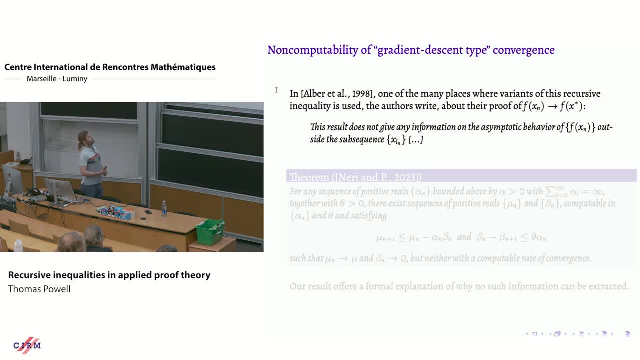 So you know, and there was a really nice paper on the convergence of one of these gradient descent type algorithms where the authors say that the established convergence, They also have some sort of subsequence convergence results, and then they say This result does not give any information. 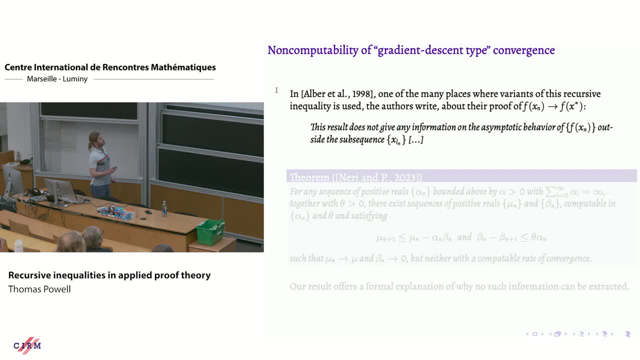 On the asymptotic behavior of f, of x and outside of that right. and so is that they just did. they just state this, and so the suspicion is that the recursive inequality they're using, although you get a convergence result, you don't get a computable rate. but actually proving that is really hard. so we adapted this speck of construction to the particular case of this in a recursive inequality, showing that in general you can have a bunch of things that satisfy those conditions but none of the convergence results come with a computable rate. 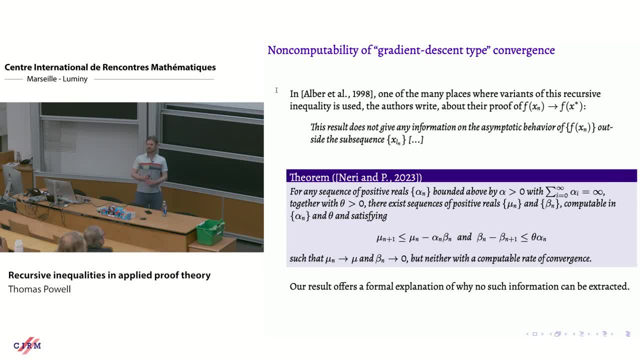 And And. that's sort of a three page proof. it's not easy, it's not obvious, trying to embed the speck of sequence construction into into concrete cases. but once you've done that, you give it an explanation as to why it was not possible to extract just by looking at the proof. get rates of convergence. 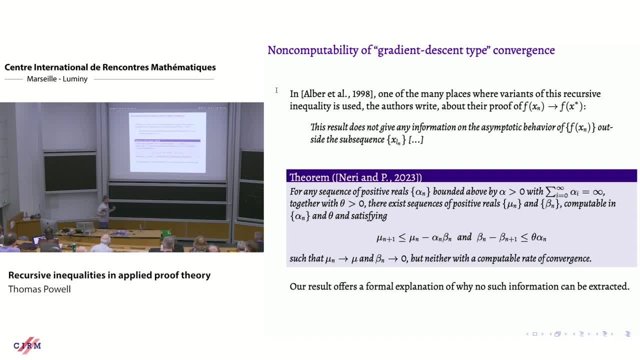 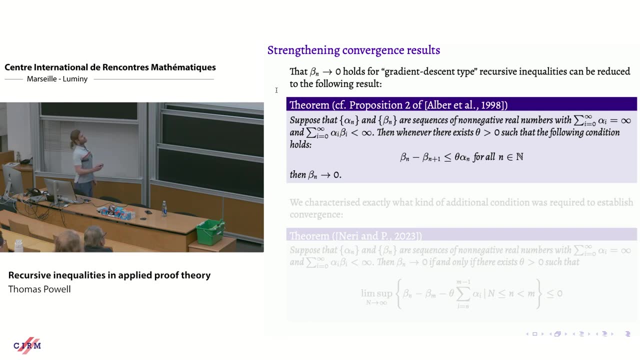 So it's kind of you know this is not so much to do with applied proof theory of the extraction of bounds. it's an explanation of why whenever you have this, you can't automatically get rates of convergence by looking And And And. we did a bunch of strengthening results where we showed that kind of when you have a convergence result of the form if, whenever we have this condition we have convergence. we showed, we came up with an if and only if statement where we showed: okay, in this situation, this is the exact characterization of what you need to get convergence. so I'm not going to talk about that too much, but this is one of the 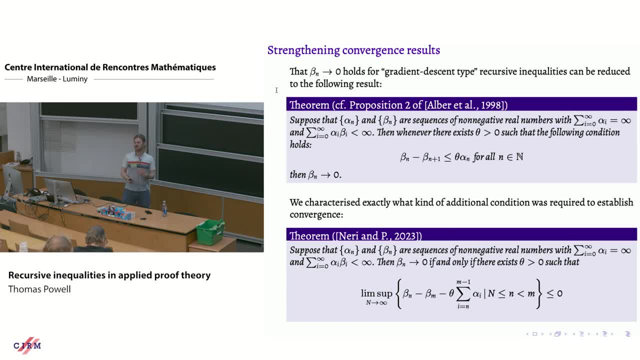 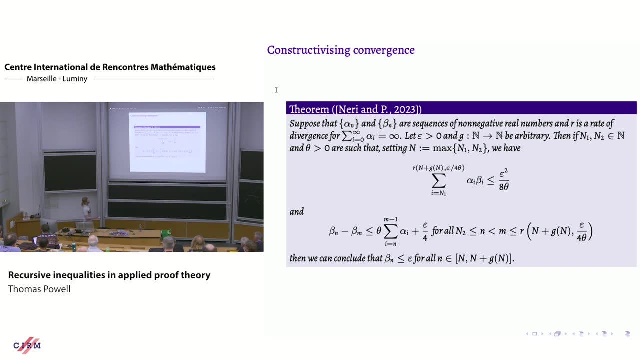 The bits of our project where we're just doing analysis. we're not doing any proof theory of computability theory. we're just strengthening these and trying to get the most general quantitative results we can. So We're giving quantitative analysis analogs of these. so the only thing that's important here is we're basically getting rates of metastability for this recursive inequality. so just like there are rates of metastability for the simple monotone decreasing sequences, we can get those for these more complicated recursive inequalities. but just the rates of metastability are correspondingly a bit more complicated. 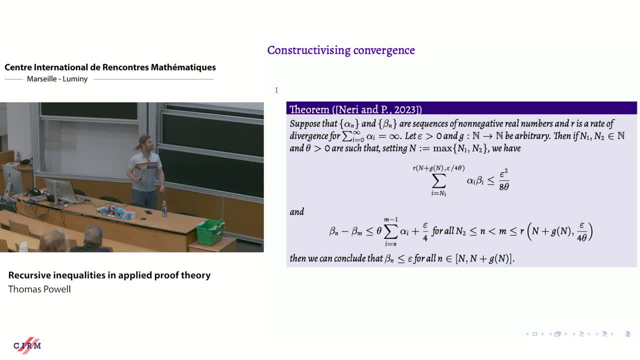 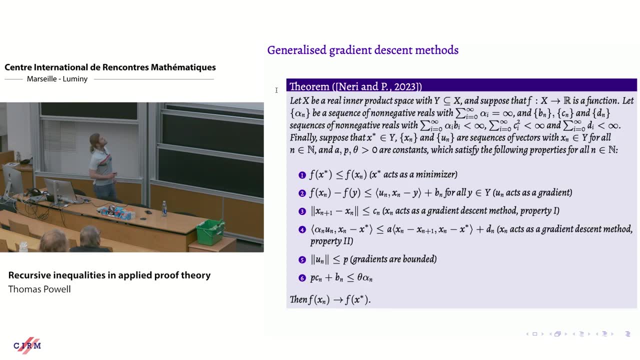 And now we come to the second thing. that always needs to be an applied proof theory talk, and that's a theorem that's so complicated It spreads over multiple slides. so here it is. so the details aren't important, but the point is that once we've- once we've done this sort of computational analysis of recursive inequalities, we can then use that to prove numerical facts about complicated algorithms. so we gave a very, very general gradient descent type. 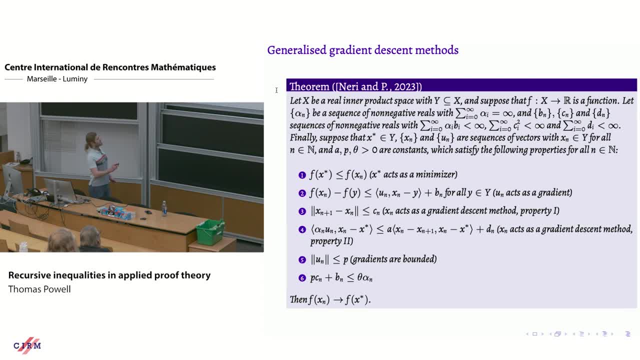 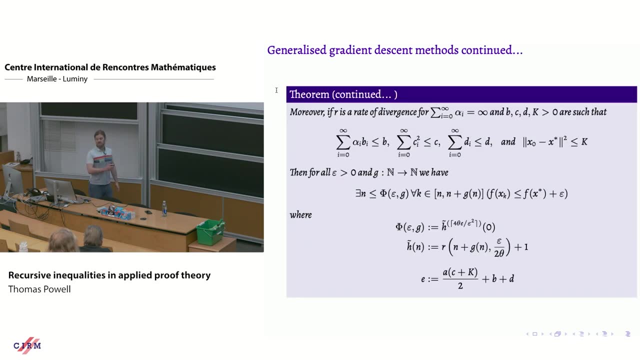 Algorithms. so we defined exactly what Abstract properties and algorithm needs to kind of look like a gradient descent method. So We give a gradient descent method and reduce to this recursive inequality. we give a convergence result and then we also give a rate of metastability for that, and then that rate of metastability can also be used to prove sort of regularity results as well. so it's not just an abstract proof, theoretic thing. 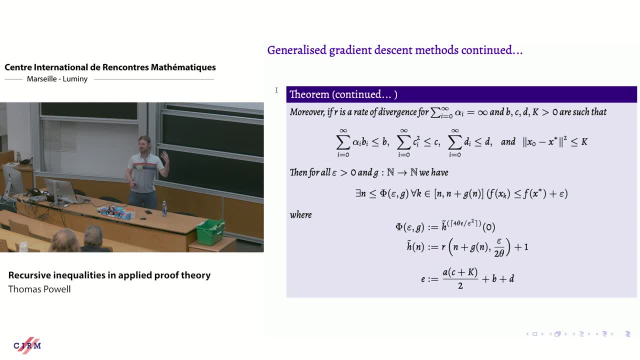 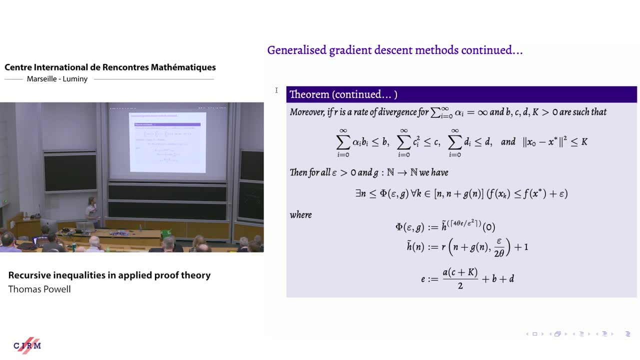 And so the this projective sub gradient method I flashed up on the slide that falls out as a special case of this. So that was the project. You know I'm not going to Make you suffer Through the horrible details of this paper, like, like all. 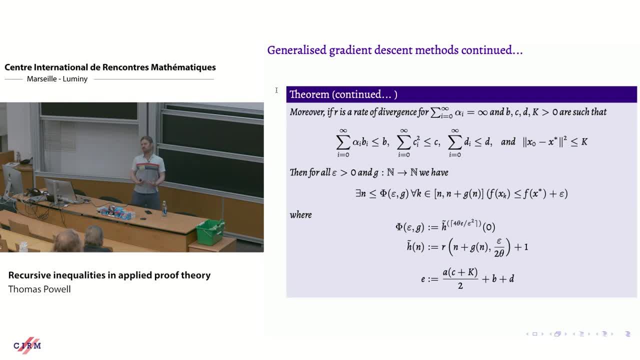 Projects in this area, kind of there's a, there's a lot of mathematical detail, a lot of proof, theoretic detail, but I just wanted to convey what we're doing, what the results look like and why they're interesting and what methods we use to get them. 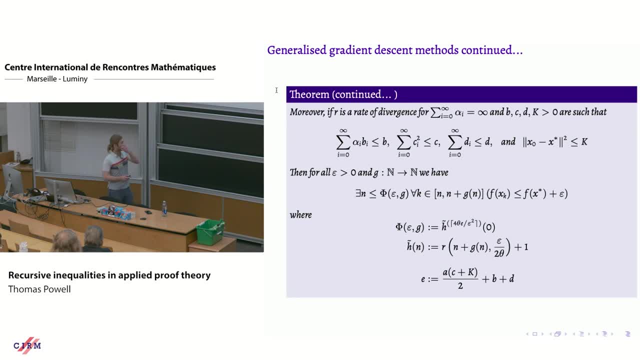 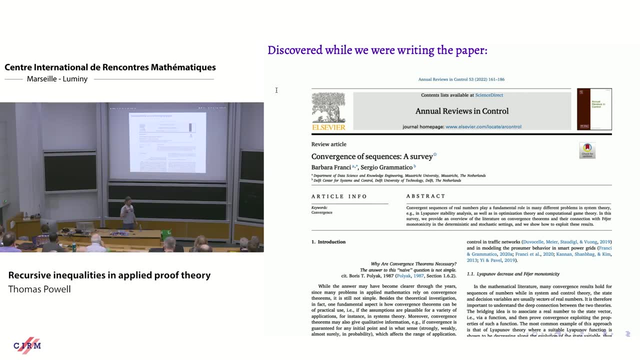 But in the last few minutes, what I want to do is explain where we're going in the future. so While we were writing this paper, we discovered a paper that was being written in parallel In it, just in the maths community- nothing to do with logic- and it was really like: well, my first thought was like, oh my God, have we been scooped? but of course we haven't, because they weren't doing applied proof theory, it was just mathematics. 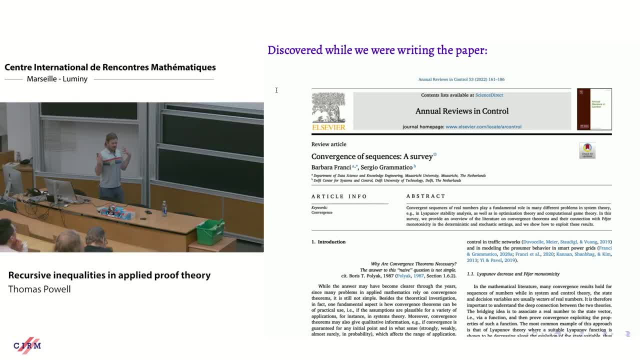 It was, and this is one of these really nice realizations- that what you're doing is somehow being done in parallel by other people and that probably reinforces what you're doing. so this was a survey article just about convergence sequences. so just about recursive inequalities in the literature, trying to survey where they came from. 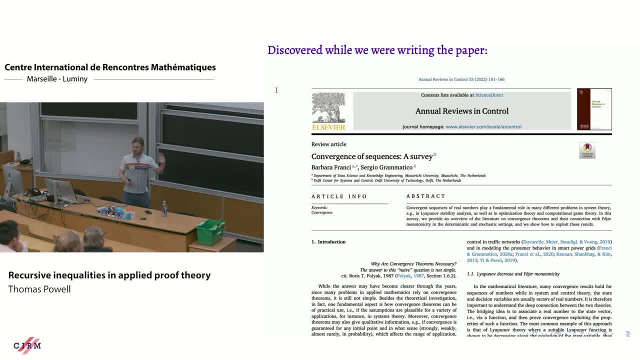 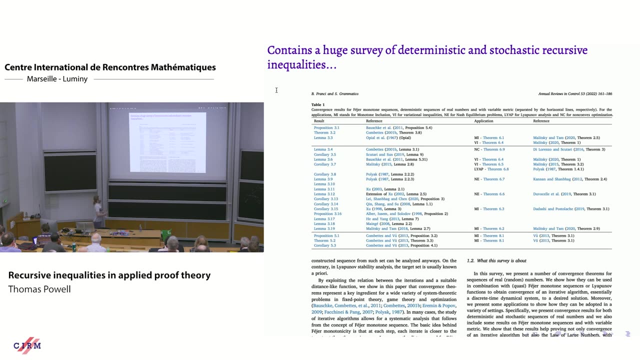 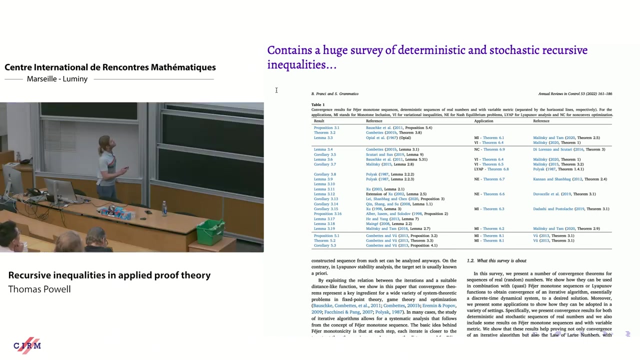 From where they were used and the differences between them. so this doesn't focus on rates of convergence or meta stability or anything like that. it's just mathematicians looking at this from a, from a kind of giving a broad overview of the field. It's really nice paper, so they give kind of big, complicated tables of kind of various different recursive inequalities in the literature and then what they're applied for. and so our, the one that we looked up for gradient descent, is just this one here, proposition 3.16, but it's just one of many. 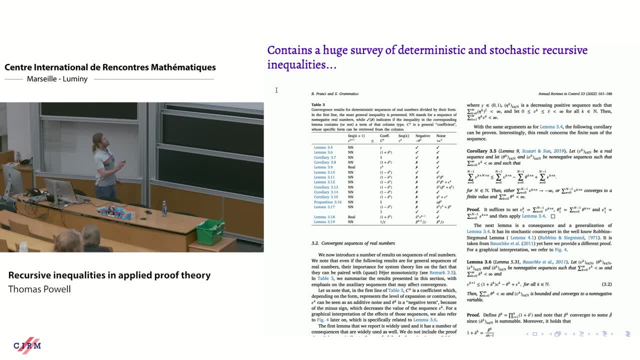 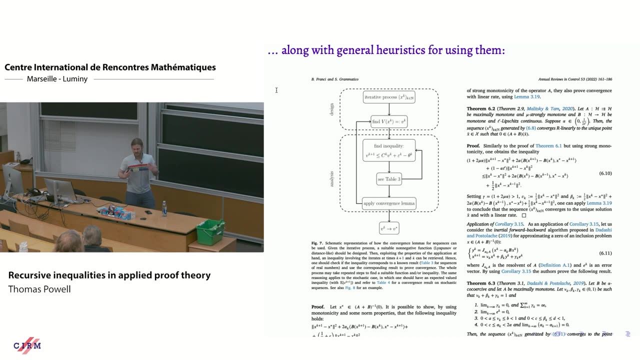 And then they also give sort of tables that classify these recursive inequalities based on different mathematical properties, so the leading coefficient, the noise term, things like that. And really interestingly they also give General heuristics for how those are used. so you can, if you know, if you've read enough of these papers, you realize kind of there's a, there's, there's, there's just a technique, and they outline really nicely what those techniques are for using these recursive inequalities. 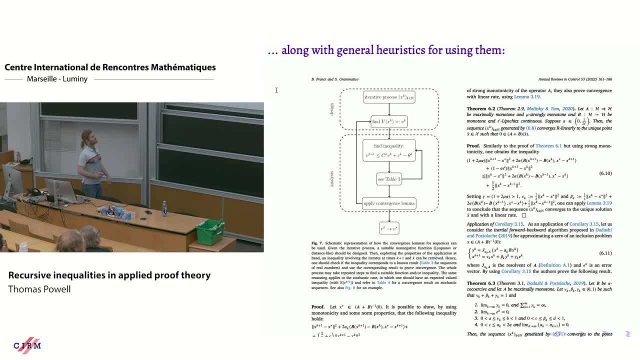 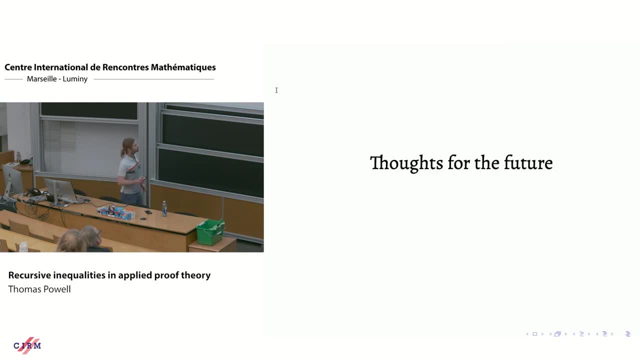 So it's a really cool paper, is really happy that this this got released Once we started In the paper and of course we cite it now and talk about it. but this brings me nicely to two thoughts of the future. so there's a bunch of recursive inequalities. we've we've studied a few of them and applied proof theory. but 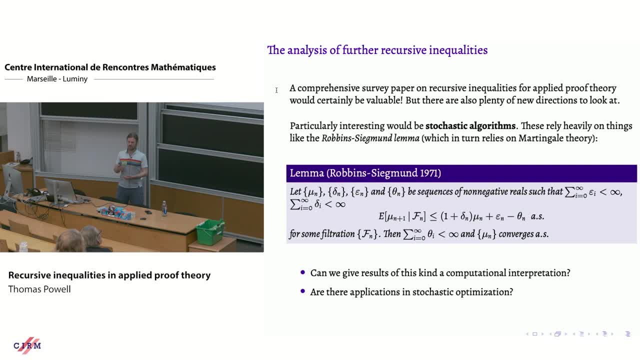 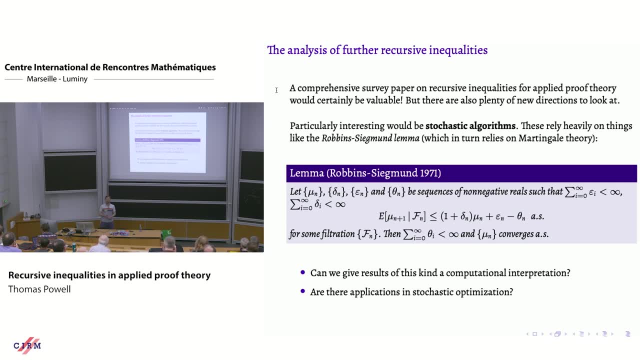 There are a lot of interesting ways to go here, so one really interesting possibility would be to look at stochastic recursive inequality. so those haven't been studied at all in applied proof theory. just look at sequences of real numbers. so stochastic recursive inequalities look very similar. but 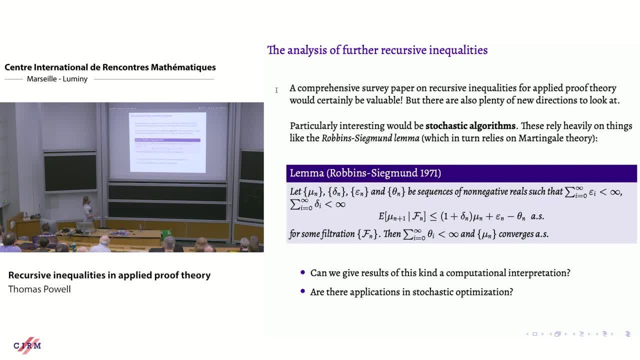 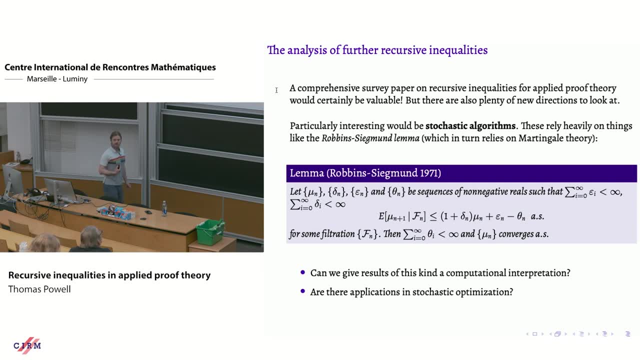 What we get is we get that all of the properties are true, almost surely, and then the convergence result is also almost sure convergence result. These are really interesting and difficult from a proof, theoretic perspective. so ordinary convergence, non stochastic convergence, is was it's, it's for all, exists for all, and so you can kind of manipulate those quantifiers and get something reasonable out. 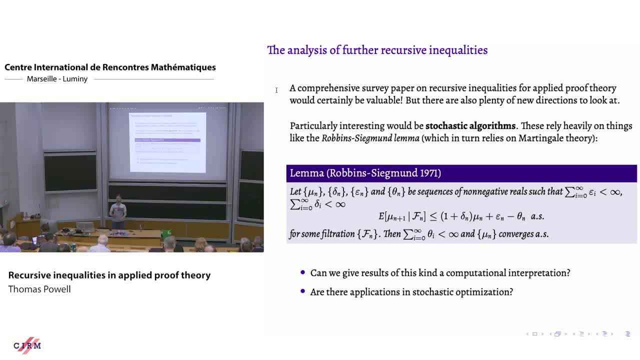 Almost sure. convergence is, logically speaking, much more complicated, and so even trying to formulate the correct way of looking at this From a finite area perspective is not obvious. and then the proofs of these convergence results tend not to use elementary analysis. they almost all rely on things like the martingale convergence theorem. 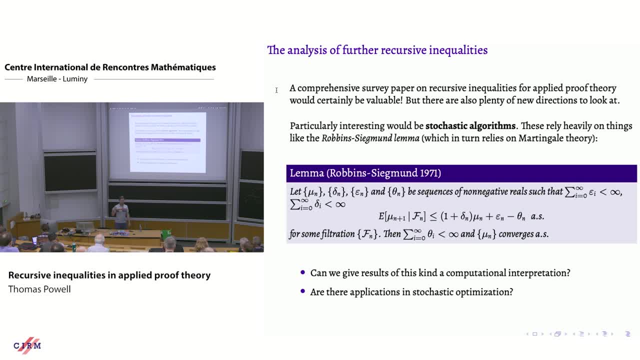 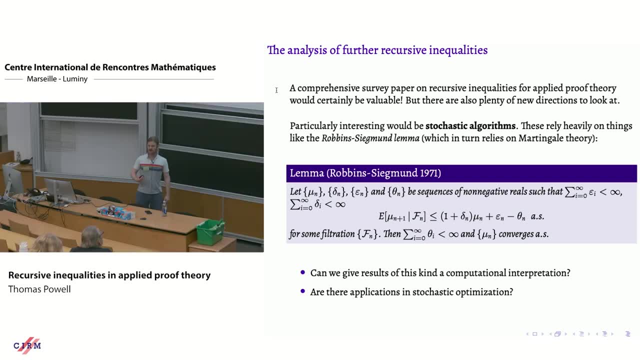 So automatically. the proofs are much more complicated, so there is some precedent in the literature. so get. jeremy avagad and some others have looked at martingale convergence theorems and try to give quantitative versions of those proofs, and so what my PhD student is looking at at the moment is trying to take the ideas that are there in the proof theory. 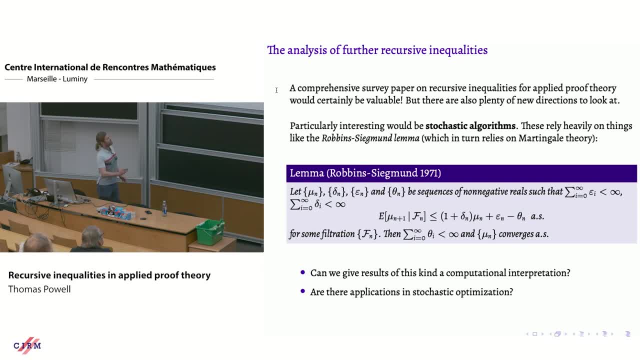 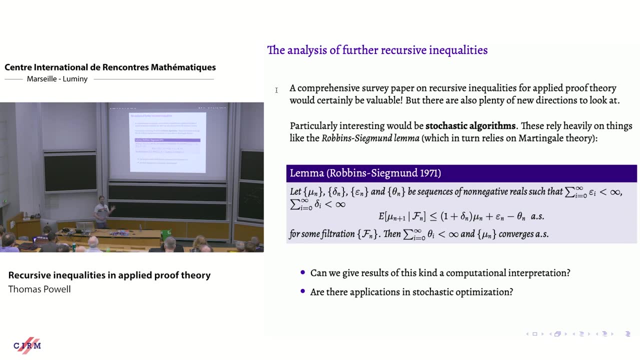 In the proof theory literature and incorporate them into giving finitary analog of some simple stochastic recursive inequalities, and this stochastic recursive inequality is called the robin siegman theorem. That's so important in probability theory that it's just tends to be shoved in the appendix of textbooks. it's just, it's just absolutely essential. and so once we give a quantitative version of that, 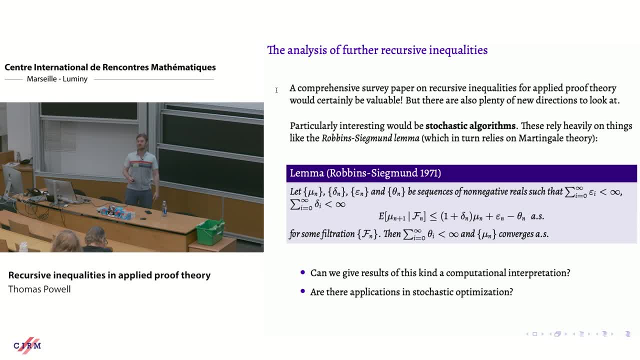 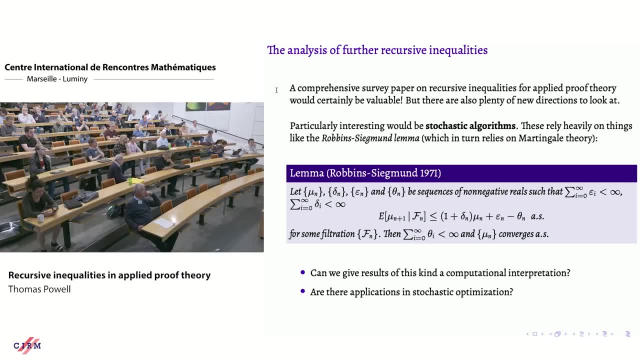 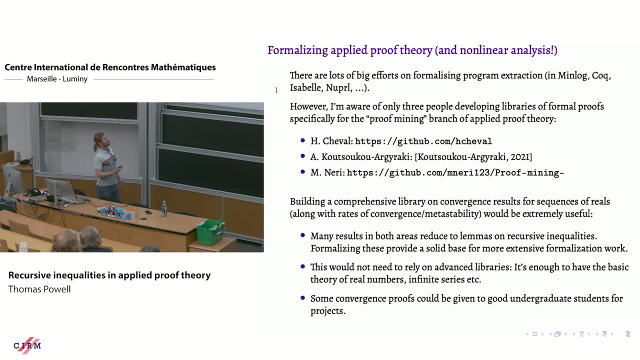 We maybe have some way in to giving interesting quantitative analogs of a lot of results in stochastic optimization. So that's the first interesting direction of future research. A second is of course formalizing all this stuff. all right, so you know there's a lot of stuff on formalized program extraction. so far, of course there's there's, there's min log and people like 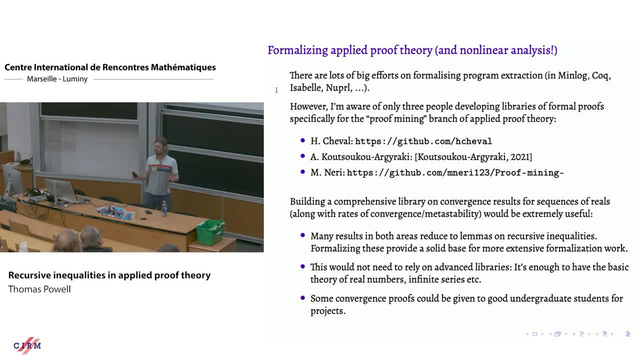 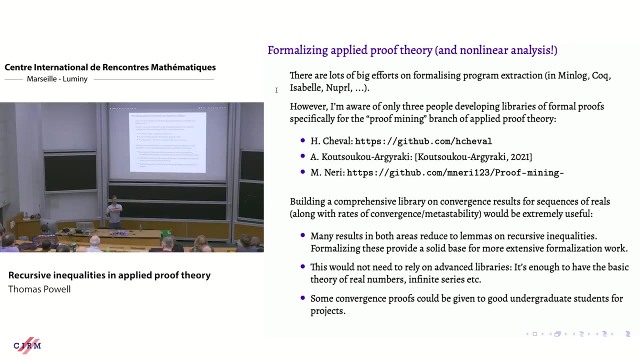 Professor schrittenberg and Ulrich Berger have been. have been have been doing this for a long time, but I'm only aware of three people developing libraries specifically for proof mining, so applications in analysis. So there's there's someone in Bucharest Who's got a really nice Lean library, now that that there's a lot of things. it's formalized dialectical but also is formalized actual, proper proof mining results. so it's formalized almost an entire paper in in applied proof to, which is no mean feat. 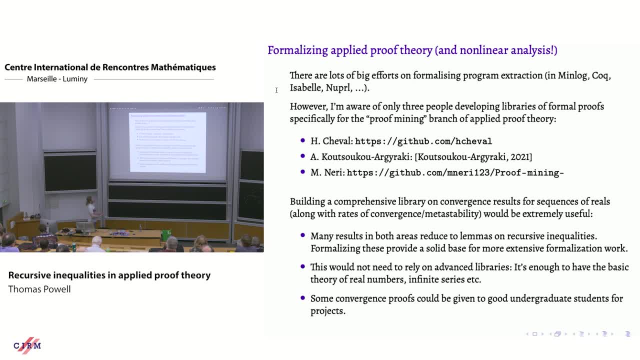 And leaky could Suka Iraqi has got she's. she's written a lot about this, so she's working with, with, with Isabelle, And she's written a lot about the virtues of having a library of Lemmas that have constructive analogs. 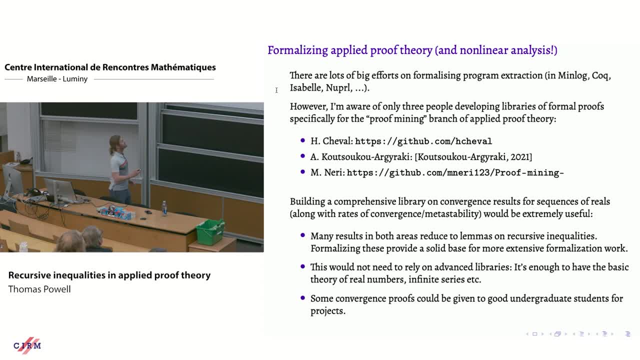 That you can use to Potentially program extraction. So I really recommend reading this paper. that was in CIE And my own PhD student- I mean, he's from this generation where they just learn formalization as undergraduates. He went to one of the Kevin Buzzard summer schools and so he already knew how to use 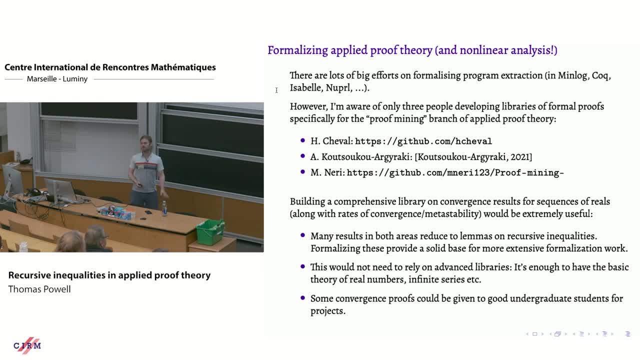 Lean when he started And I said, well, why don't you formalize some of these? And he's like, okay, And then one afternoon he's done it. So it's incredible. I'm too old to do this, but but Kejie's, Kejie's. 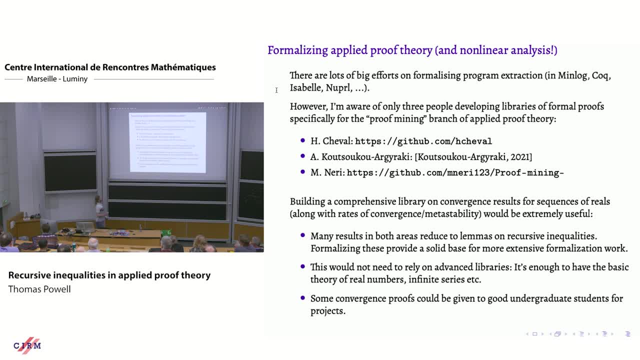 I'll tell myself that, So you know. the specific idea I'm getting at here is that you've got a bunch of recursive inequalities. These are really important in both optimization and in applied proof theory, So we can start building a catalog of formalized versions of these. 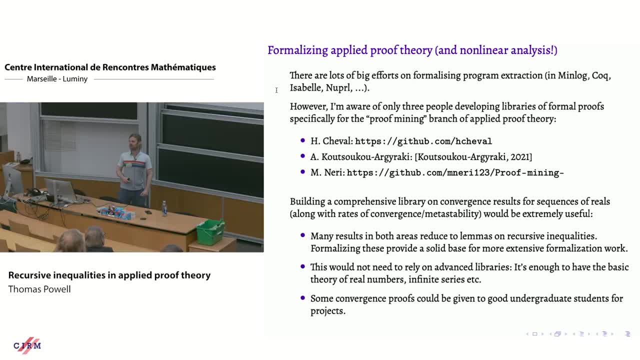 recursive inequalities in an effort to formalize bigger parts of both nonlinear analysis and applied proof theory. And the point is that you know you don't even need to rely on advanced libraries for this, You just need to know basic facts about, about for most of these recursive inequalities, the non-stochastic ones, it's just elementary. 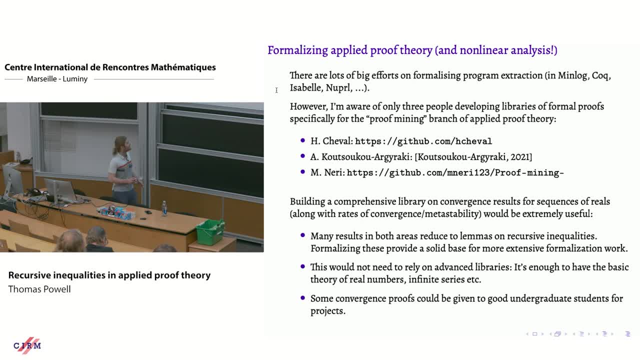 analysis, So you don't need to have learned a load of Lean to be able to do that, And so this could even be a project for good undergraduate students, where they do something that has some sort of meaning but which could realistically be done in a few months. So it'd be really. 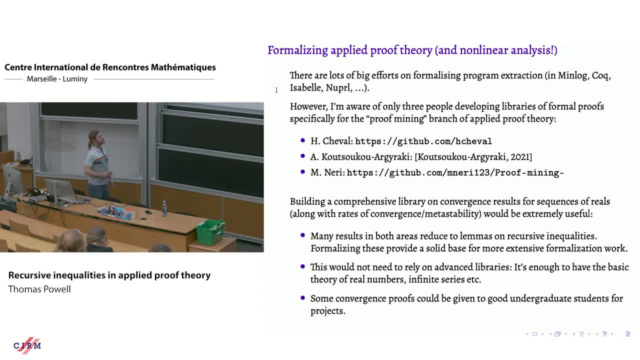 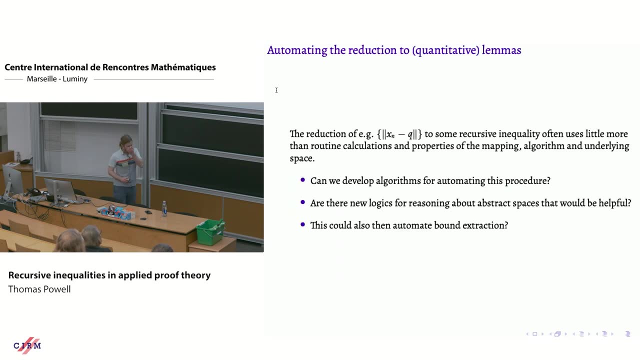 nice to and we're we're we're starting to build these libraries, but but hopefully within a few years we'll have a good kind of a good basis to formalize more analysis and applied proof theory And the final idea, which is so that's just an example, it really exists, The final idea. 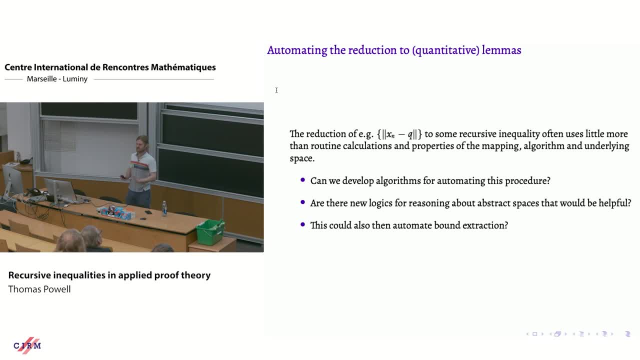 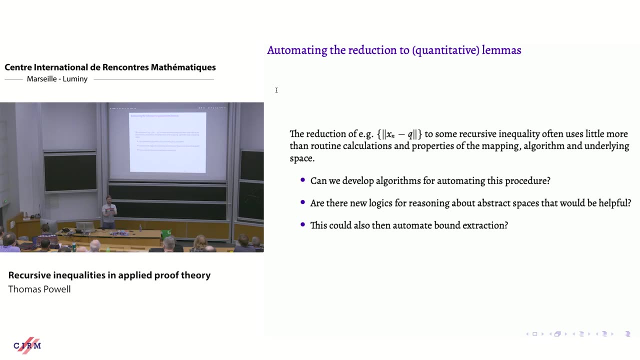 which I kind of- there's no initial work here at all, So this is really wishful thinking, but I'm really interested in it nevertheless- is to apply automated reasoning. So when these convergence theorems are reduced to recursive inequalities, typically all that's involved.